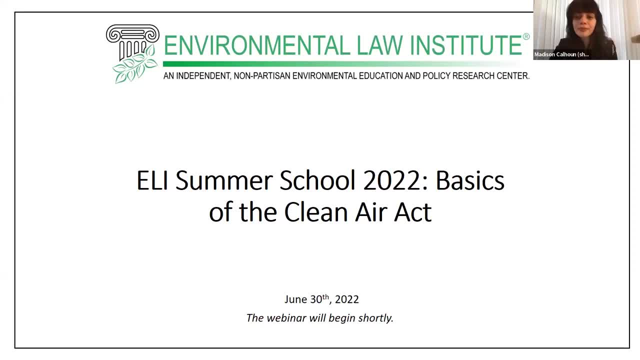 Thank you, Thank you, Thank you. Hello everybody, I'm going to give everyone one more minute to join and then we'll get started. Thank you, All right, Welcome everyone. Welcome to the Environmental Law Institute's fifth summer school session. 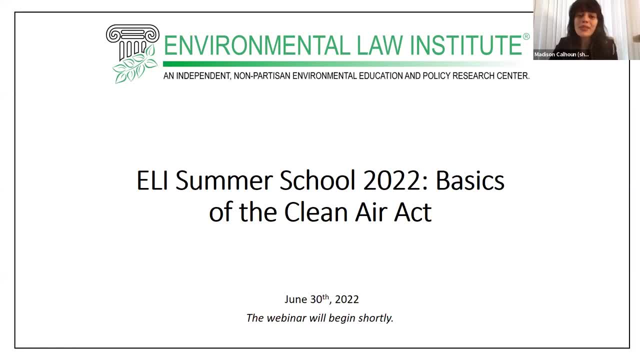 This week's webinar will be focused on the Clean Air Act. My name is Madison Calhoun and I'm the Senior Manager of Educational Programs here at ELI. We have a great program in store for you today. I want to take a moment to thank all three of our fantastic panelists, who spent a lot of time preparing wonderful content for you all today. 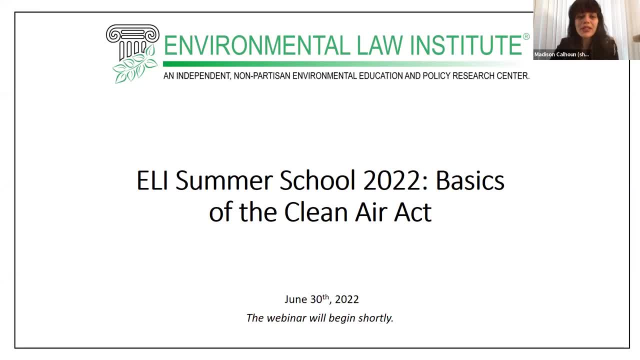 I also want to thank our audience for taking the time to tune in. We hope that you find this series engaging and informative. I have a couple of logistical notes before we get started. If you have any technical issues during the webinar, please send me a direct message. 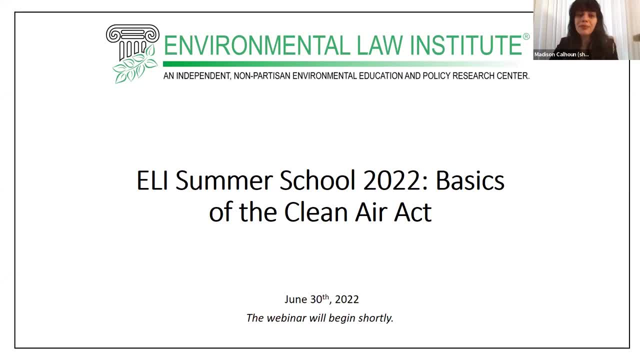 Today's event will consist of two presentations followed by a roundtable discussion. We are saving a good amount of time at the end for audience questions. Please don't wait until the end to submit your questions, though. As soon as you think of something you'd like to ask, please submit it in Zoom's Q&A box. 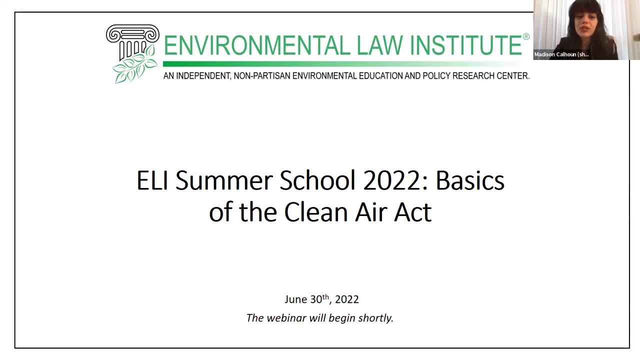 You're free to use the chat as you'd like, but it's a little easier for us if you ask your questions for our panelists in the Q&A box. Today's webinar will be recorded and posted on ELI's website. If you can't stay for the full two hours or if you have any colleagues who cannot make it, please check back on the event page for the reporting early next week. 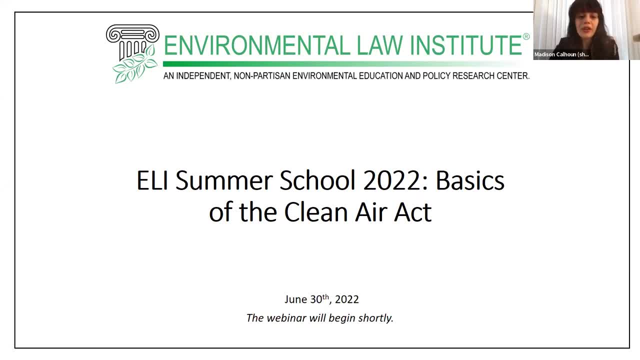 I will now introduce our moderator. Summar Prisupati is the Inaugural Environmental, Justice and Community Engagement officer at the Bay Area Air Quality University, Bay Area Air District. Before joining the Air District, she was appointed by Governor Gavin Newsom in 2019 to serve as Assistant General Counsel for Enforcement at California EPA. 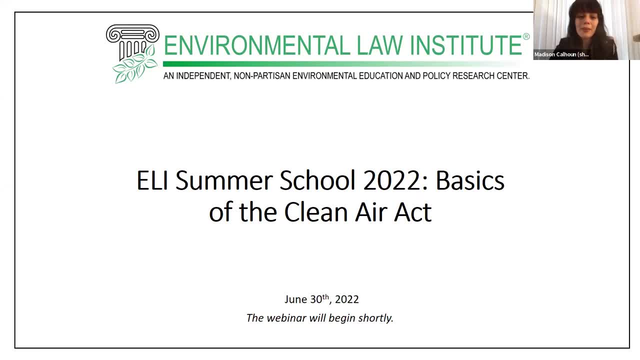 She has more than 20 years of experience practicing law in the private, non-profit and public sectors, specializing in environmental law. Prior to her appointment, Suma was a Deputy Attorney General with the California Attorney General's Bureau of Environmental Justice, where she focused on environmental enforcement in low-income communities and communities of color. 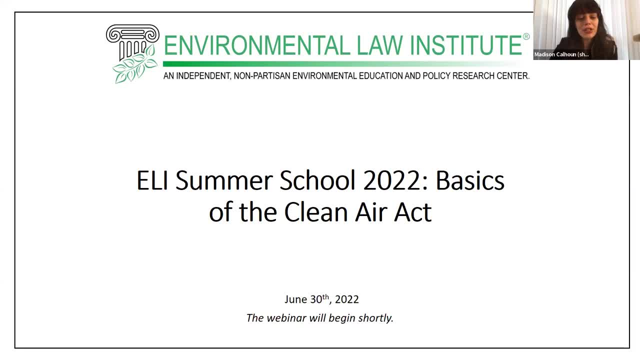 In 2017, she founded Peace of Body Law, a plaintiff's environmental law firm in San Diego. She served as a Visiting Assistant Professor at UC Irvine's Environmental Law Clinic and as adjunct faculty at UC Davis and UC Berkeley Law Schools. Earlier in her career, she practiced law. 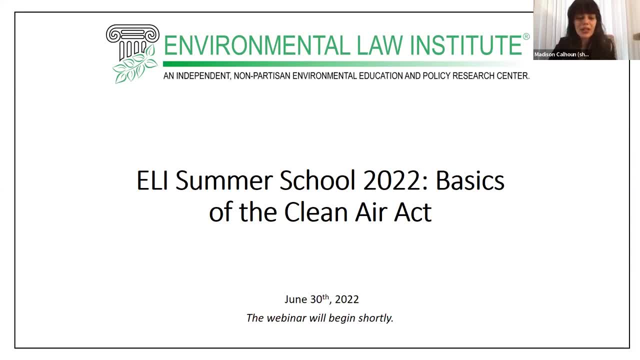 in the Bay Area as a Staff Attorney with Earth Justice, as an Associate Attorney with Small Plaintiff's Side Law Firm and as a Staff Attorney, and an Equal Justice Works Fellow with Communities for a Better Environment. She has also served as a Deputy Attorney for the US Department of Justice. 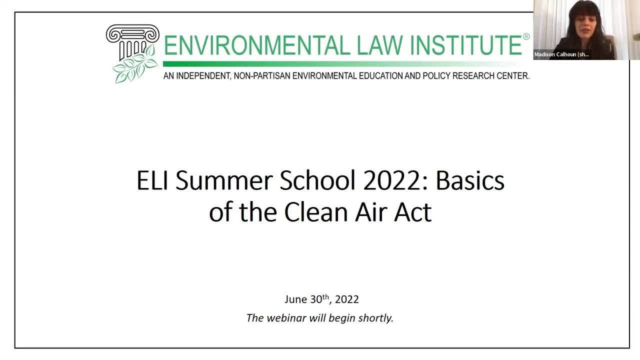 and the Department of the Environment. Suma is also an advisor to the Executive Committee of the California Lawyers Association's Environmental Law Section, Suma. I will hand things over to you and thank you so much. Thank you, Madison, for that kind introduction. 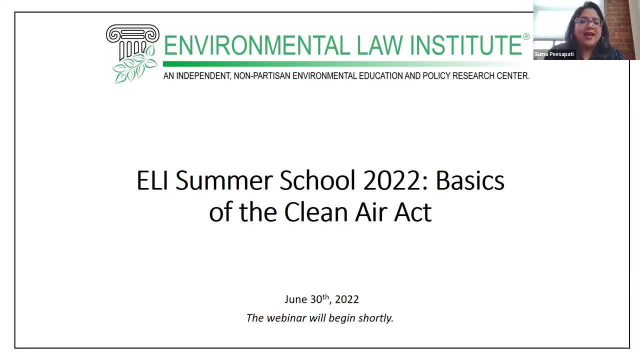 and welcome everyone to the summer session. basically a Clean Air Act 101.. And I, in turn, would like to start by introducing our esteemed panelists. For me it's still morning, for, I think, some of you it's afternoon. So, starting with Angela, Angela Morrison is a member of the Florida Bar and is a partner with 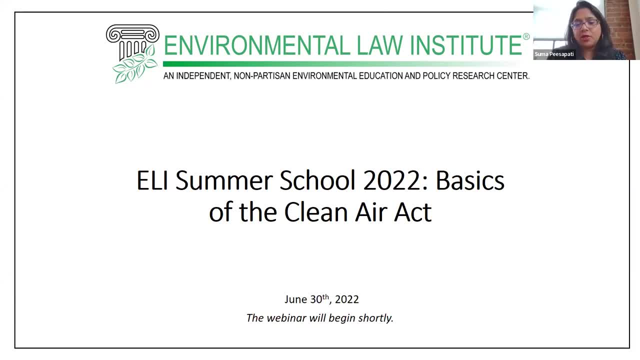 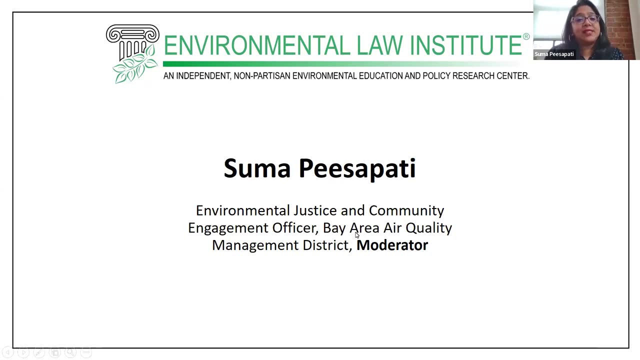 the Washington DC-based virtual law firm Earth and Water Law, Angela has focused most of her 32-year environmental law career on air quality and climate change issues, air permitting and the siting of energy facilities. Angela has significant experience with New Source Review. 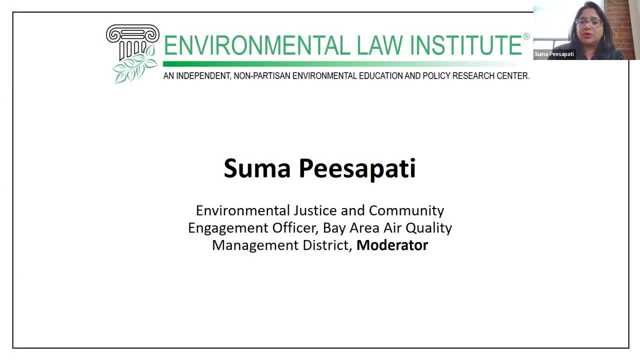 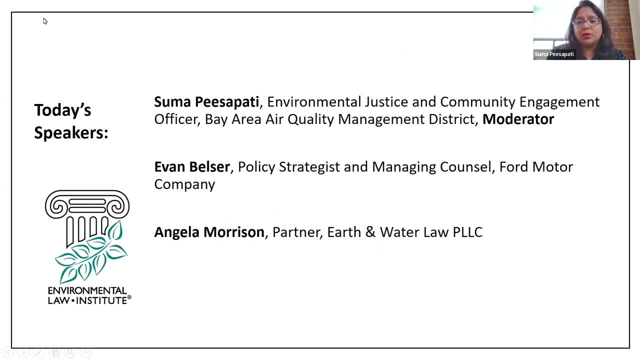 New Source, Performance Standards, Hazardous Air, Pollutant Requirements, Risk Management Plans, Emissions Trading Programs and Renewable Fuels. on behalf of utilities industry and trade organizations. Angela is the co-author of the American Bar Association's Clean Air Act Handbook, both the third and fourth editions, and is also the co-author of the ABA's 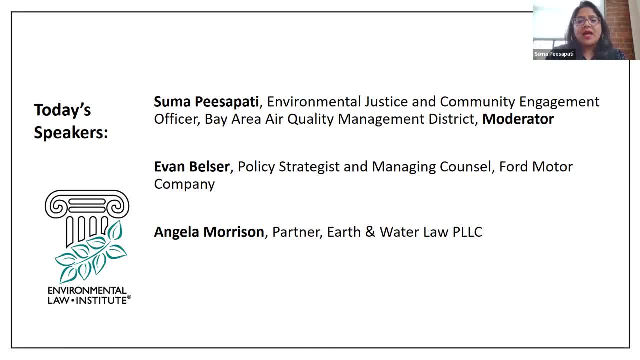 Clean Air Act: Essentials, third edition. Angela just completed co-authoring the Clean Air Act chapter for ELI's treatise on environmental law. Angela has been active for many years with the Florida Bar's environmental and land use law section and also the ABA section of environment. 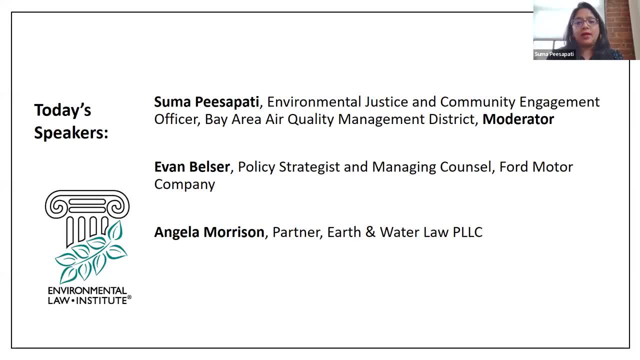 energy and resources, having served on council, the book publications board and as executive editor of Trends and as the chair of the Air Quality Committee. I'm sorry my eyes for some reason decided to suddenly start watering. Please ignore it. 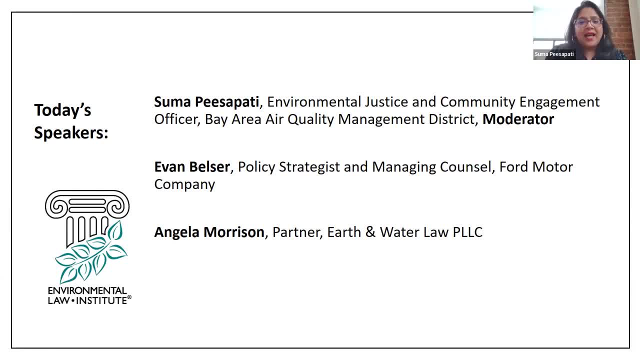 Turning to Evan Belser. Evan Belser specializes in legal and policy matters concerning air pollution control, climate change, environmental enforcement and remedies, and the decarbonization of transportation and energy. Before this year, Evan joined Ford Motor Company as a policy strategist and managing counsel. 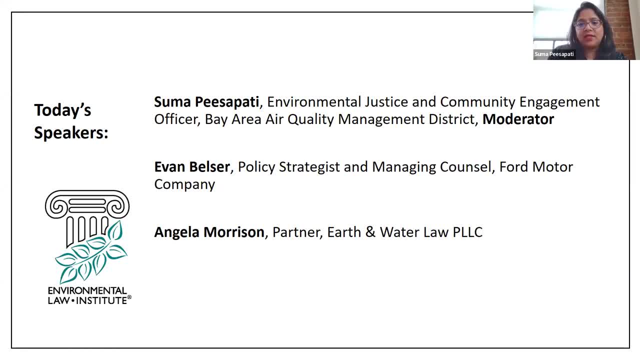 Before 2022,. this year, Evan served in numerous roles, including acting director in the US EPA's Air Enforcement Division. Before EPA, Evan graduated with honors from Vermont Law School. Evan lives with his wife and three children in Washington DC. 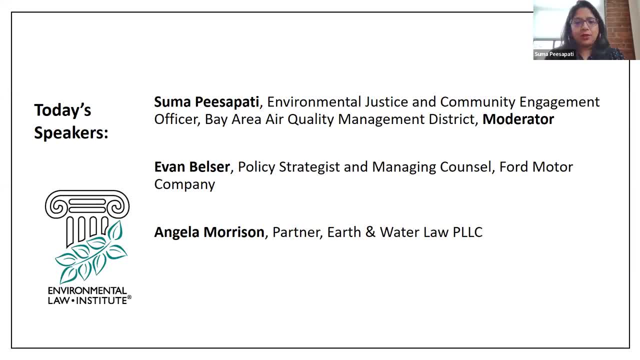 As Madison mentioned, Evan is also a lead administrator in a board of directors and policy-making group run by the Florida State Department and India's Federal Government. I'd like to start with a very brief introduction to the Clean Air Act, followed by longer presentations by both Angela and Evan on stationary and mobile sources. 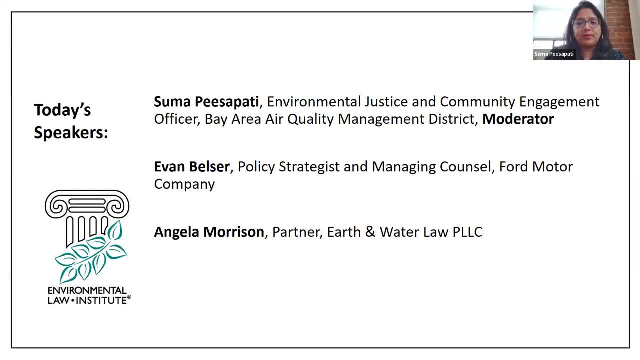 respectively. Then I'll facilitate a Q&A with our panelists and welcome audience questions. in the time, that remains a very brief and simple- perhaps you know, overly simple- introduction to the Clean Air Act, which is a very complex and interesting statute. So the Congress passed what's known as the Modern 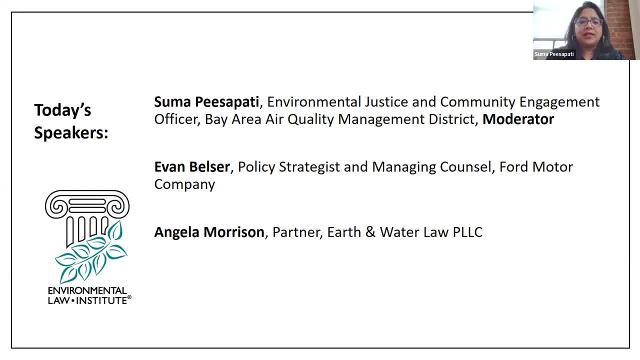 Clean Air Act in 1970. It was a groundbreaking legislative effort, both in its scope and its guiding principle of what's known as cooperative federalism, where the federal government and states share power work together in implementing the statute In the state and federal partnership. 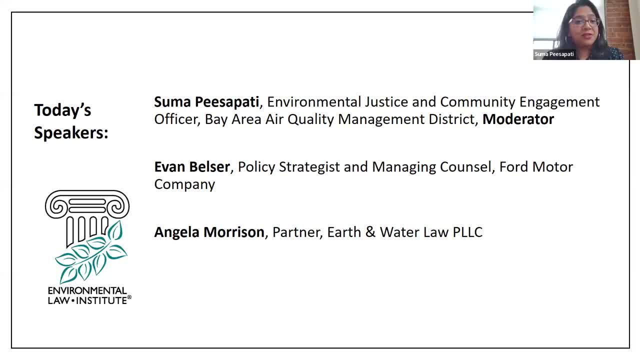 the federal EPA sets national public health-based air quality standards that apply throughout the country. They're known as NACs- those air quality standards. Then the responsibility shifts to each state or, in California, California's case, local air district to develop an air quality monitoring system to first determine. 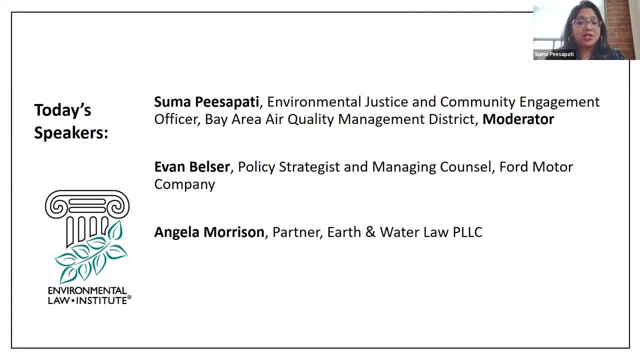 whether local air quality meets those national standards developed by EPA and to develop a plan to either meet, if the local air basin is not in compliance, to either meet or, if it is in compliance, maintain compliance with those national air quality standards. So those local and state implementation plans are then subject to federal EPA approval. 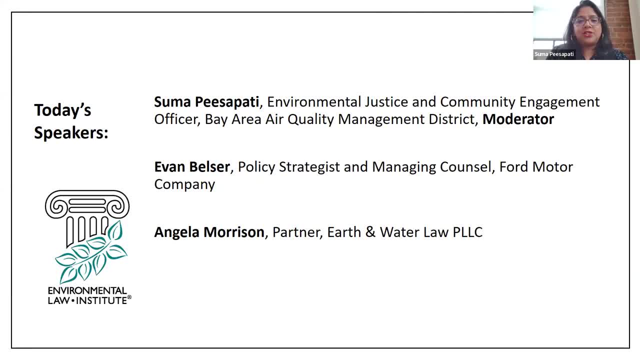 If a state can't produce an acceptable plan within the statute's deadline, the EPA is authorized under the Clean Air Act to prepare a federal plan on its own. That said, EPA imposed federal plans are rather uncommon. Usually EPA will give a state or you know. 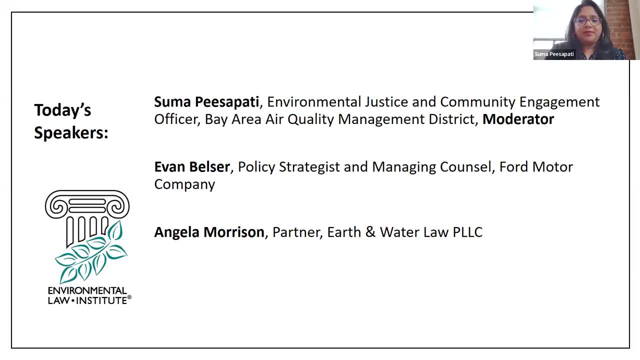 a fair chance, They will give a fair chance to get their plan right. So there's actually a relatively small universe of air pollutants that meet the Clean Air Act's criteria for requiring national standards or the NACs, And those six kind of categories of 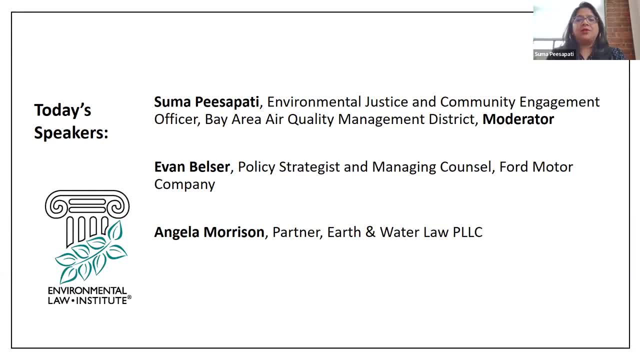 pollutants are particulate matter, which includes both large and small particle pollution, ozone, sulfur and nitrogen. And those six categories of pollutants are particulate matter, which includes both large and small particle pollution, ozone, sulfur and nitrogen, And those six categories of. 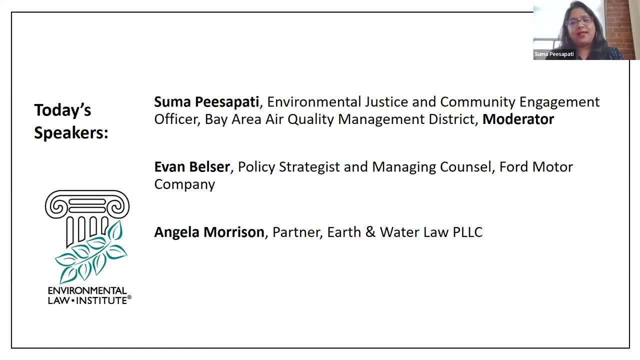 pollutants are particulate matter, which includes both large and small particle pollution: ozone, sulfur dioxide, nitrogen dioxide, carbon monoxide and lead. A defining feature of the Clean Air Act is also its technology-forcing provisions. The statute requires state-of-the-art pollution controls on new major industrial facilities. 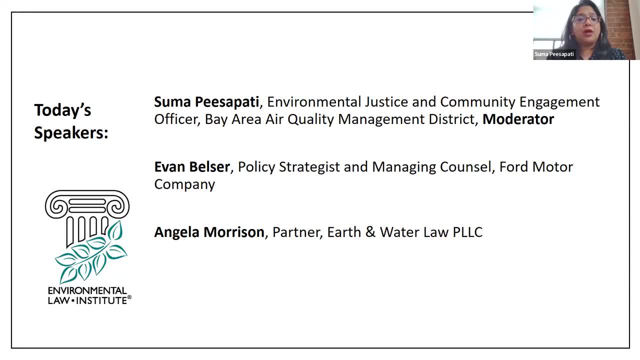 It also requires state-of-the-art pollution controls on major modifications to those facilities, And when a region's air quality doesn't meet EPA's national standards — isn't good enough to meet national standards — then the costs of those controls aren't even included in the 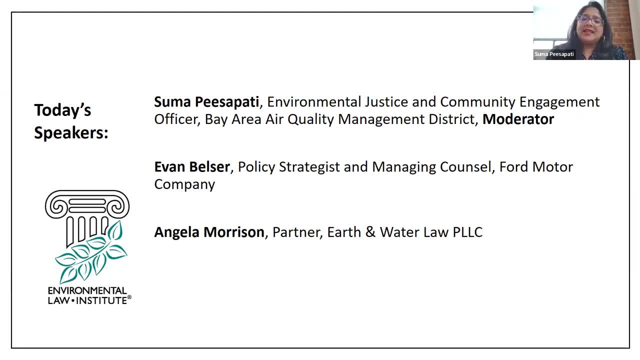 technology analysis. So the point of this statutory framework is to really to drive innovation in the field of pollution control And perhaps, you know, even over time to eliminate industrial pollution. So you might ask yourself, you know with, you know this innovative approach? 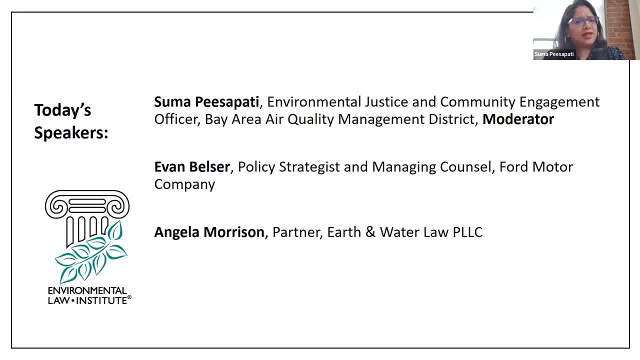 with a statute that is unique in being premised on protecting human health and forcing the very best pollution controls. you might ask yourself: why hasn't the Clean Air Act solved the problem of environmental injustice, where air pollution is often concentrated in low-income communities? 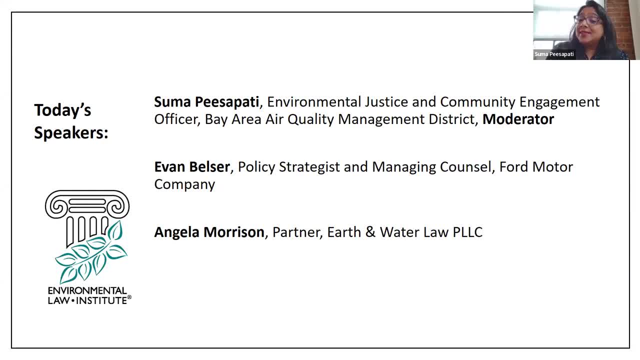 and communities of color throughout our nation. This is a particularly thorny question here in California, where we have some of the most polluted air basins in the country, specifically the LA Air Basin and the San Joaquin Air Basin. So there are a couple of reasons for this disparity. 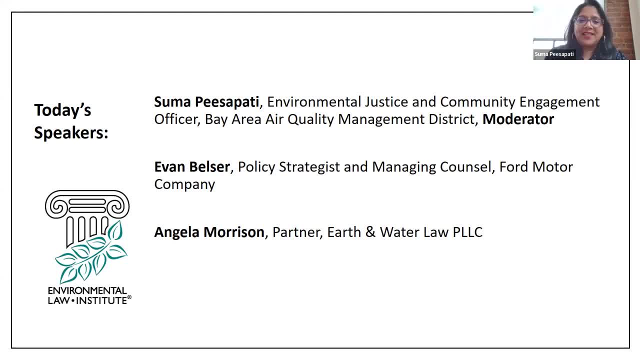 What's known as the Great Air Act is a grand compromise of the Clean Air Act was its focus on new sources, Not entirely, but almost to the exclusion of existing sources. So you know, the existing sources were basically grandfathered into the statute. And if you think about it, where the 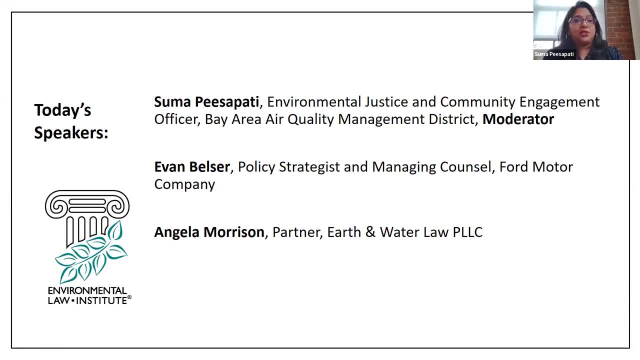 vast majority. where were the vast majority of industrial sources located when the statute was passed in 1970?? Obviously in poor communities, in black and brown communities right, And actually the presence of industry was a major factor in the practice of what we call redlining right, which made it. 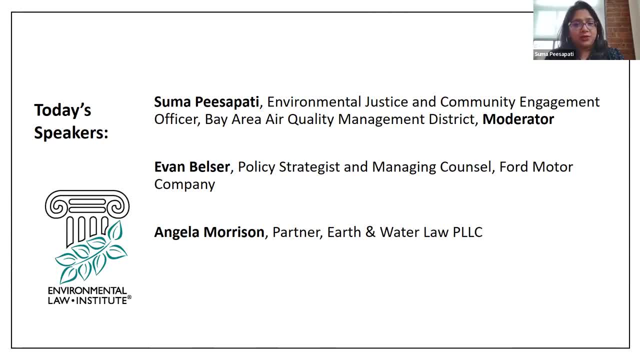 difficult for people in redlined communities to get mortgages. Making matters worse, industry would often target redlined communities to site their facilities due to the perceived lack of power in those communities to fight off those undesirable land use. And so you know there's a lot of. 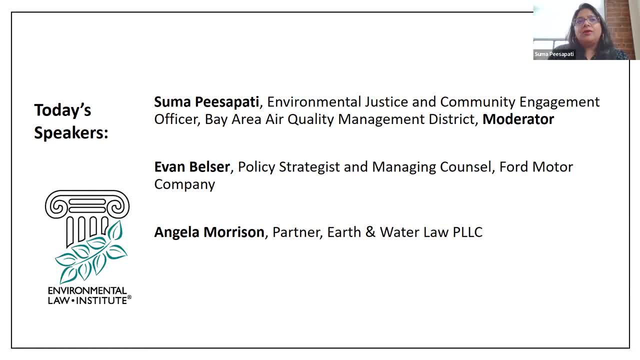 change here for the demand uses. Another unintended consequence of the Clean Air Act is, you know, it's technology, it's forward-looking technology, forcing provisions. Oddly enough, in most cases, building a new industrial source is so much more expensive than extending the life of an existing control tool. 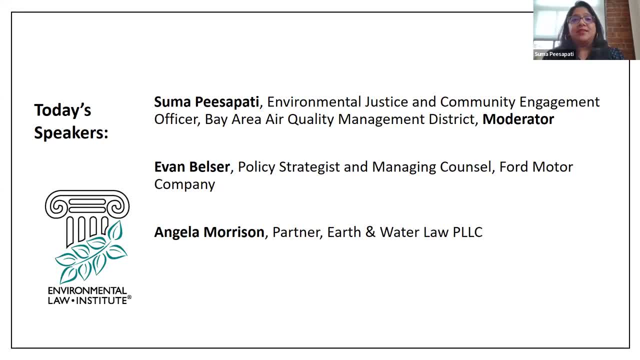 facility that there's a disincentive right to building new, cleaner sources And perhaps an unintended incentive of just continuing poorly controlled sources by making small, minor modifications to that facility that extend its life over time. So you know what we've seen. 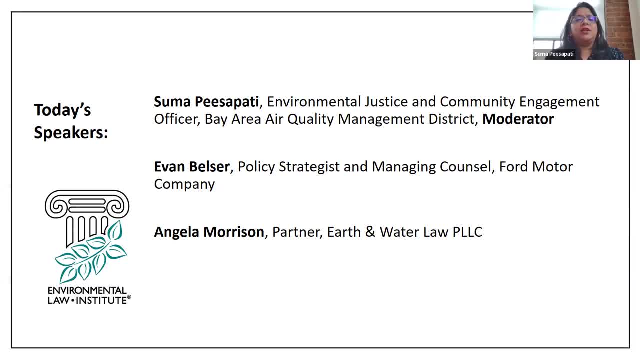 here in California is that, even though the engineering and financing assumptions for major industrial facilities usually don't go beyond a 30 to 50-year life, we routinely see large facilities like oil refineries that have been around for more than a century. So what is the point here? It's not simply to depress the audience, It's to urge the importance. 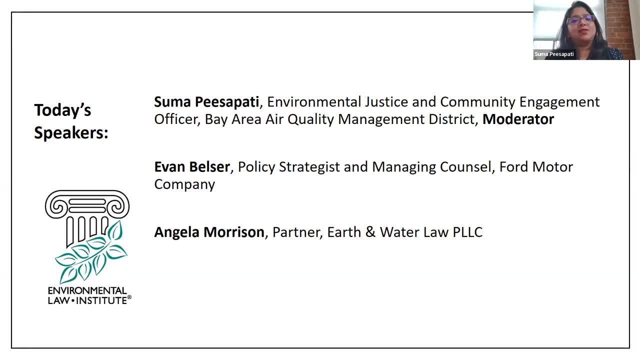 of understanding the importance of building new, cleaner sources. And so you know, I think it's important to understand that our environmental laws exist in a social context, And I say that because environmental law, and air quality law in particular, is a pretty technocratic field of. 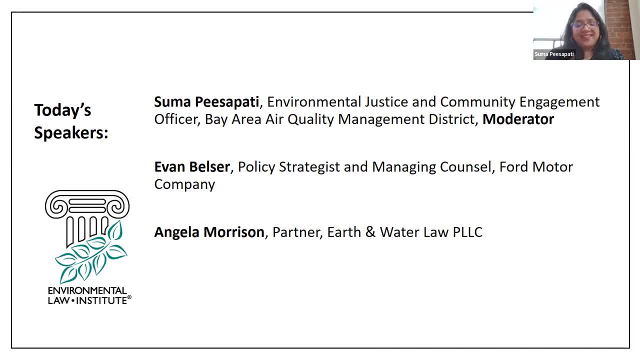 practice, And as much as I personally love to nerd out on all the fascinating and deeply complex aspects of the Clean Air Act and air quality law generally, it's equally important to understand that this regulatory scheme exists in a social context And that our practice should be informed by on-the-ground lived experience. 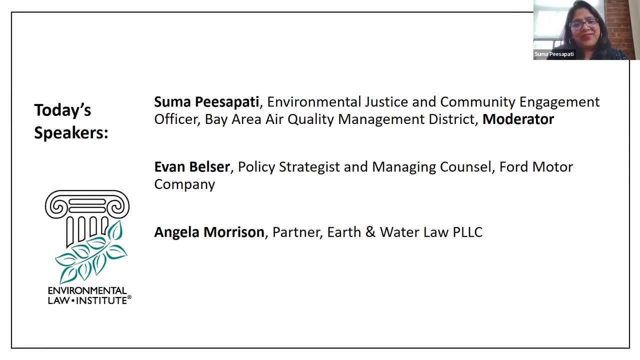 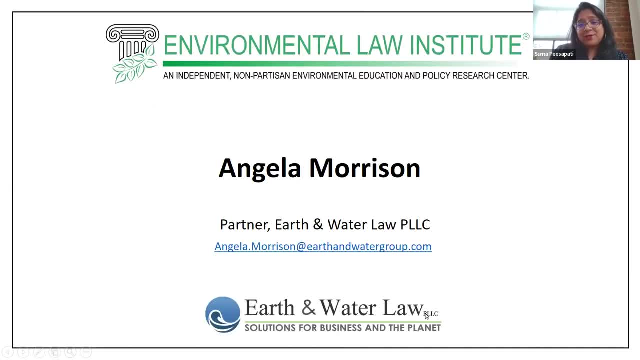 And so with that I'd like to turn it over to Angela and Evan. Angela will start with a bit of a deeper dive into the world of stationary sources. Thank you, Angela, Thank you Suma, for that introduction and for also giving those background principles of the Clean Air Act. 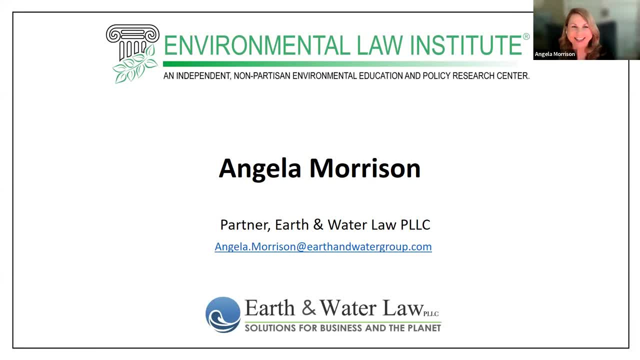 And I guess this is a little part of what we're going to be talking about in the next few minutes. This is a little portion where we're going to nerd out a little bit with the Clean Air Act, But I appreciate that background And we should keep all of that in mind And I'll help. 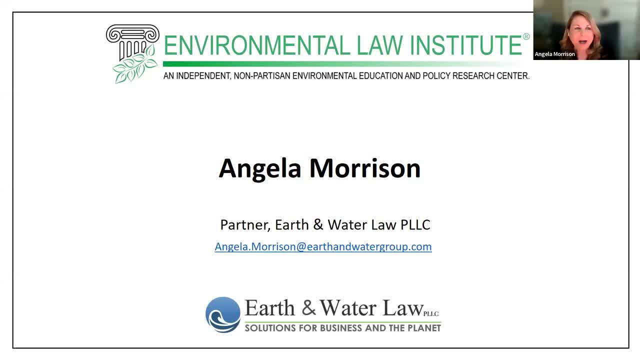 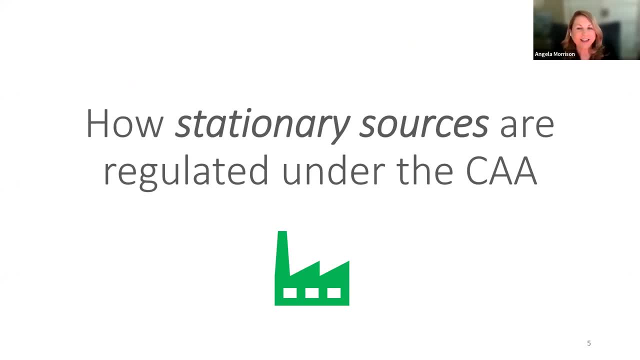 I'll try to interject some of that as we go through these slides. Next slide: We're going to start by talking about stationary sources and how they're regulated under the Clean Air Act, And I'm especially excited to be presenting on this today in light of the 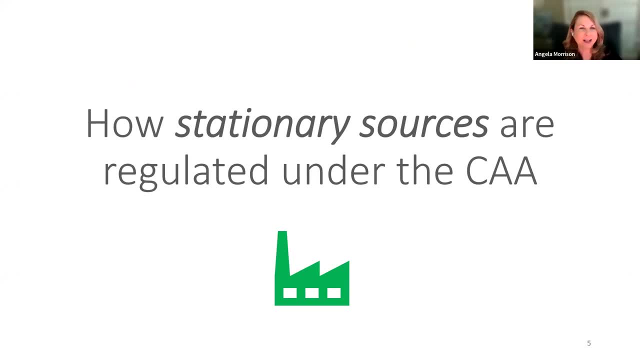 Supreme Court decision that came out earlier And this might, you know, provide some helpful background as you begin to review and analyze that decision. I'll just be scratching the surface of this topic. My intention today is to give you a very high-level. 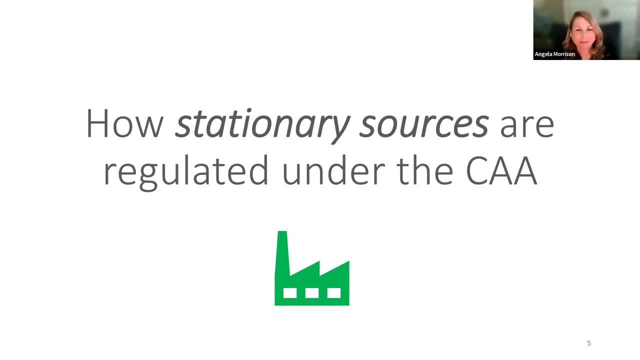 overview of how the Clean Air Act's many different parts work together or don't, in their overlay to regulate stationary source air emissions. Between the 70 Act and the 77 and 90 amendments, there has been overlay after overlay, making it more and more complex. 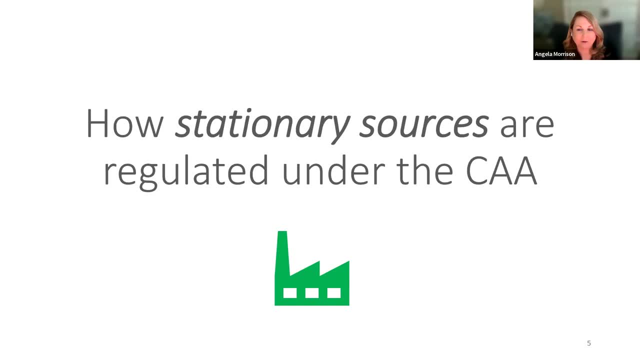 If we were starting from scratch today, it would look much different, But unfortunately that's just not the case. So we have the Clean Air Act as it is, with all its many overlays and duplications and inconsistencies. But I'll do my best, But please just realize. 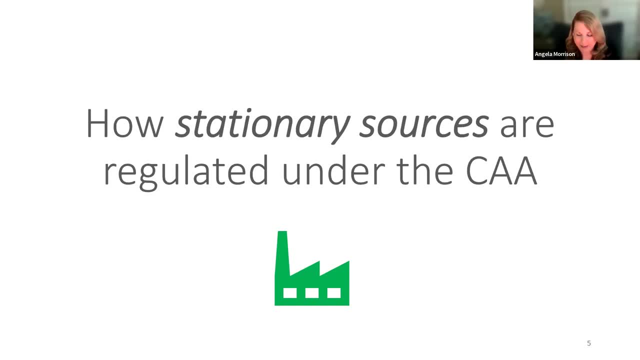 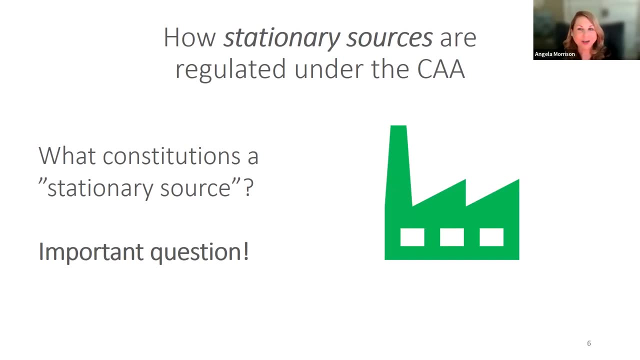 that the Clean Air Act is a bit complicated. Next slide. So what constitutes a stationary source? It's probably really good to start with a common understanding before we just delve in here. Many of the terms under the Clean Air Act have very specific meanings under different parts of the Clean Air Act, So you have to be careful to 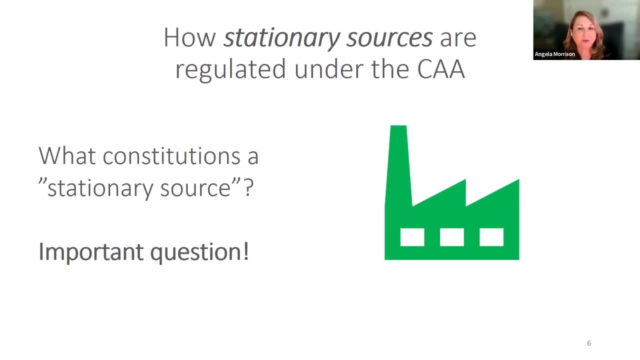 always know and appreciate the particular definition that applies to your specific rule or program, And my thought in picking the term stationary source was really to distinguish it from mobile sources. that Evan will be covering, And it's not a bad place to start, but there 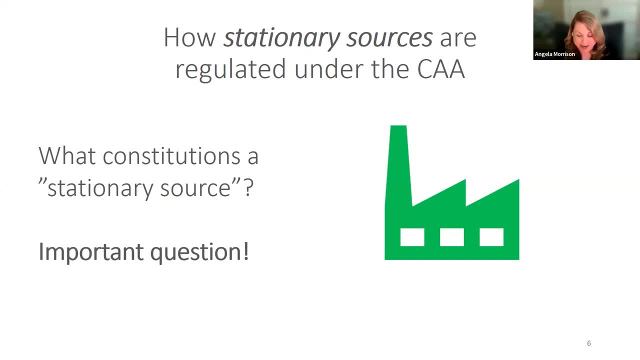 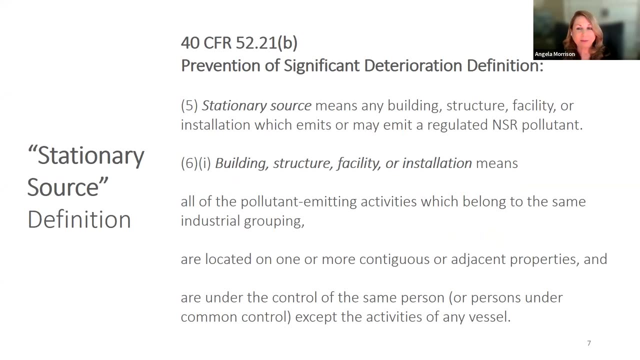 are too many definitions to go over, So I just have to say that it's a good place to start. Thank you. Next slide, So I picked one from the Prevention of Significant Deterioration: PSD New Source Review Permitting Program Reminder. this is only one definition out of many And you can get the sense. 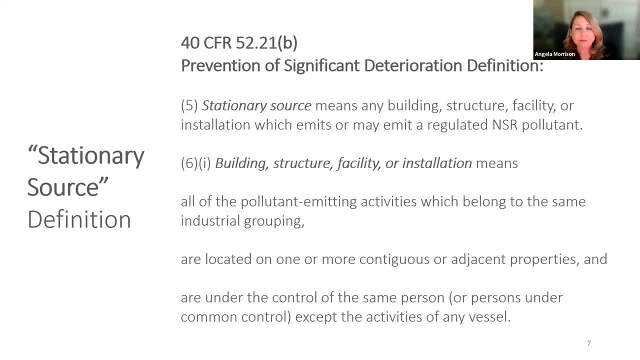 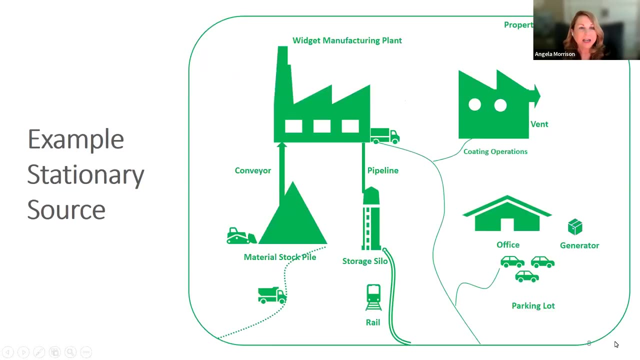 from this definition that it's a whole site. It's more than one. what you think of as an emission unit It's everything at a site and generally references pollutant emitting activity. As we go through this process, we're told to select certain types of equipment, such as: 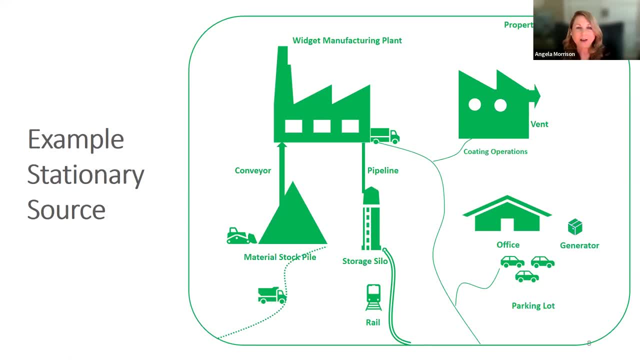 equipment in storage as well as other types of equipment. For example, if somebody owns 12 to 15 units, they may need to collect a total of 10 units of equipment, And you can tell the difference between these components in terms of how to do the work. So we have a lot of ten points to look at here. Two points to look at if you want to stay specific. we're going to have to take advantage of the quality of the equipment that's included in this, and we need to look at it to see if it is a good fit to use. We also have ahadeha. To help you visualize this, I've developed this illustration. This is a widget manufacturing site with many different buildings and operations and roads and offices and stockpiles and silos and pipelines, all kinds of things. Next slide. 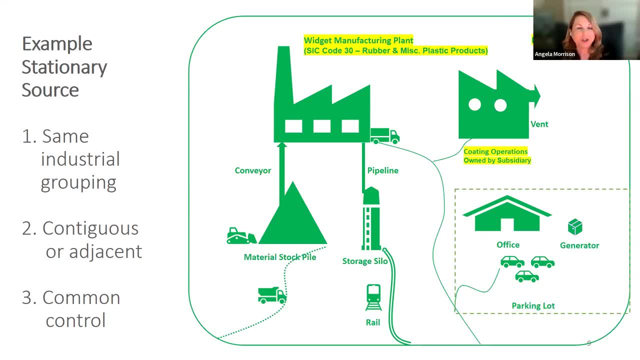 look at. you know, is it part of the same industrial grouping, which is really a two-digit SIC code, and I picked number 30, which is rubber and plastics, not really knowing what makes up a widget. so does everything on this site fall within the same source category and you've got coding operations. 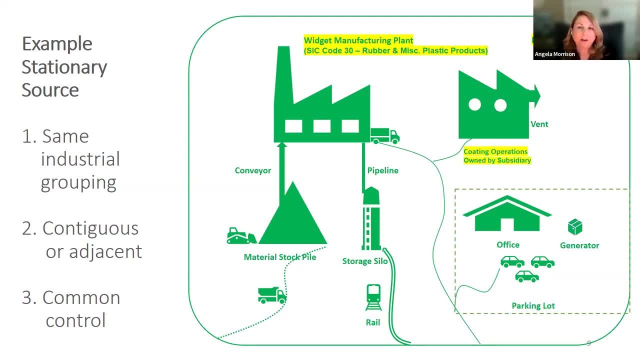 which are different. but if they're a support facility for the widget manufacturing, then perhaps it is part of that. if it's completely separate and not tied at all, maybe it's a separate facility, a separate source. is it on contiguous or adjacent property? I marked off the office with the fence, but fences don't really separate sources. that would all be one source, even. 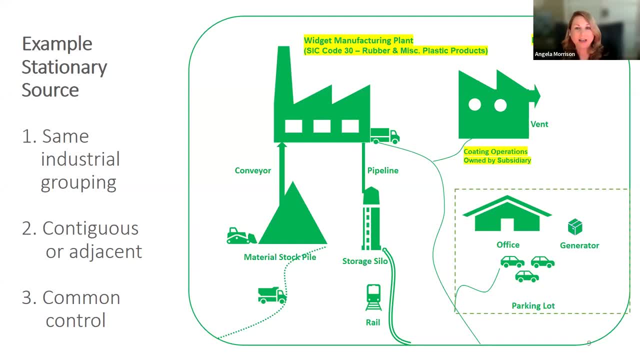 if part of it's fenced off, it's all contiguous or adjacent. and the next question is that under common control I have the coding operations owned and operated by a subsidiary. usually that's not enough for separate controls. it might if it's a wholly separate company with separate management. perhaps then it is not under. 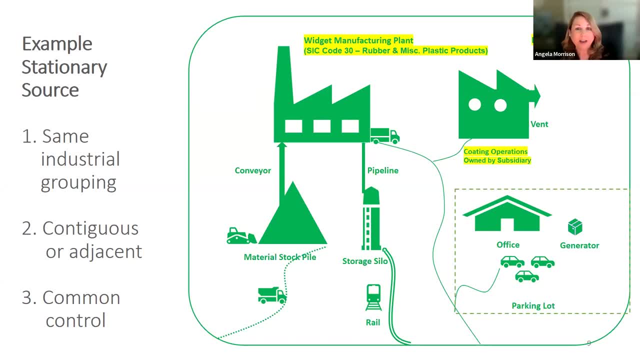 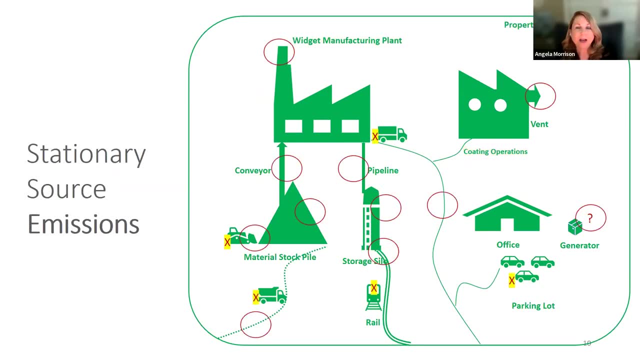 common control. but these are some of the questions we face when we're looking at what is a source- next slide. it's also important to identify which activities might have air emissions that are subject to stationary source regulation. what you think of as a stack or event? obviously. 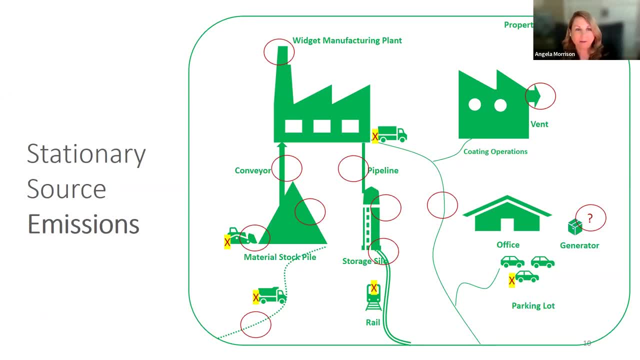 those are part of a stationary source. but things you might not think of if you're new to regulation under the clean air act are conveyors and stockpiles and materials handling fugitive emissions and leaking pipes and your backup emergency generator- maybe just all kinds of emissions. 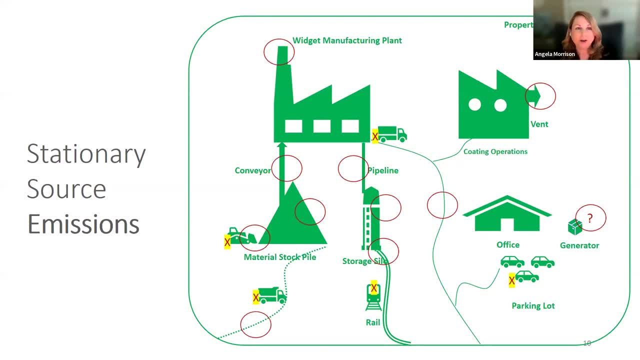 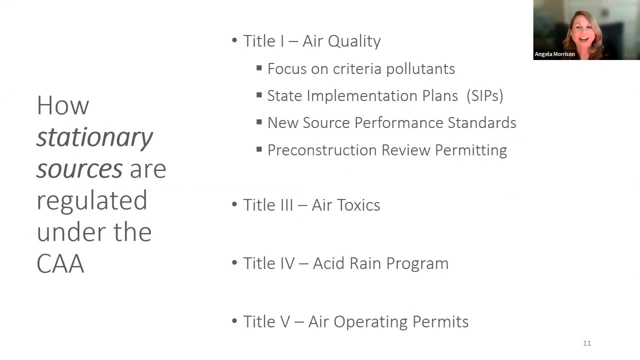 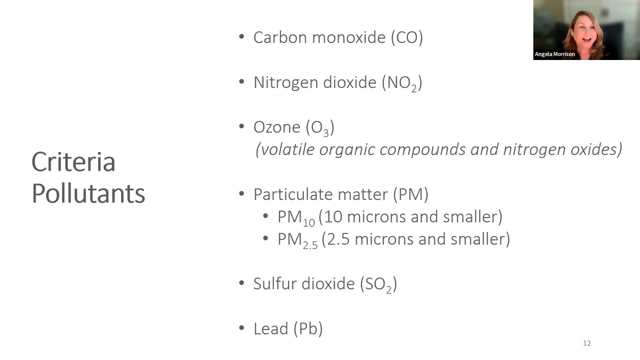 at a site, usually tailpipe, emissions are not regulated as stationary sources. sometimes you use volunteer or sewage a casserole. you know you don't make a good next slide. there are a number of different titles under the Clean Air Act that regulate stationary sources and we'll be covering some of them today. there are others that we just don't have time to cover проблем. 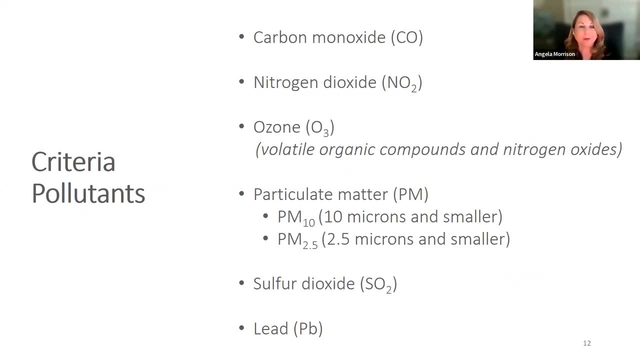 putions and suma mentioned. i've just laid them out here. there's a separate list of elements that same year already out. forär would be super important here on post. sixty Congrats. would you please share some of the credits from the information descriptors them out here. There's a separate list of hazardous air pollutants. That's much longer. 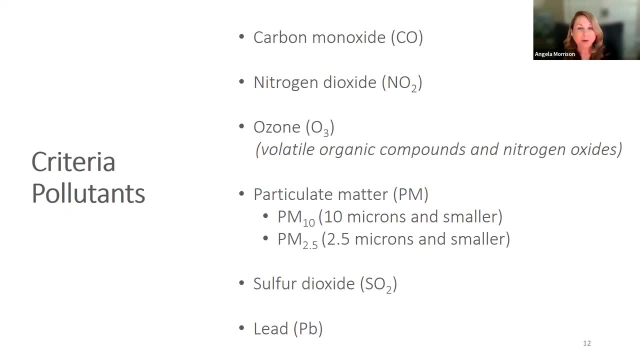 There are currently 187 hazardous air pollutants or air toxics. We use those terms interchangeably. That's much more extensive than this. Originally it was 189.. Two were removed, One's in the process of being added, but for the most part it stayed pretty much the same since the 90 amendments. 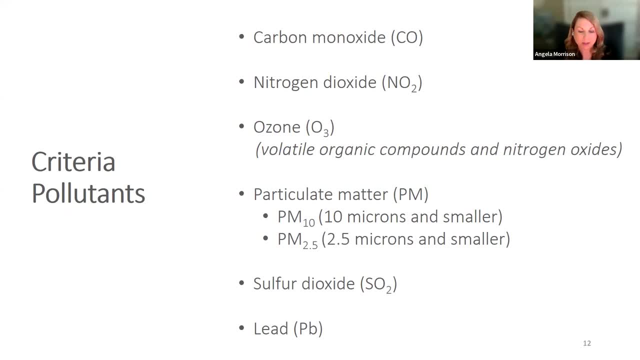 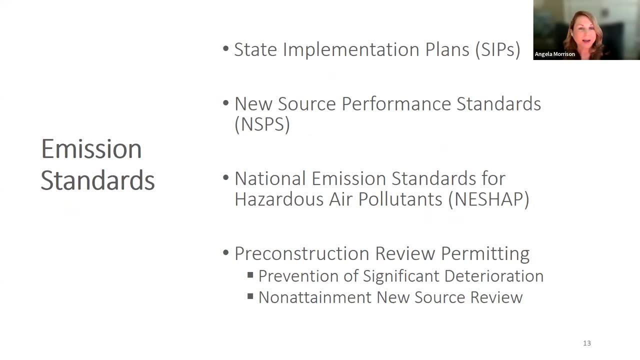 But it's important to understand the difference between criteria, pollutants and HAPs. So that's the reason for this slide, Next slide. So emission standards can be established through a number of different programs, state and state implementation plans that Suma mentioned. 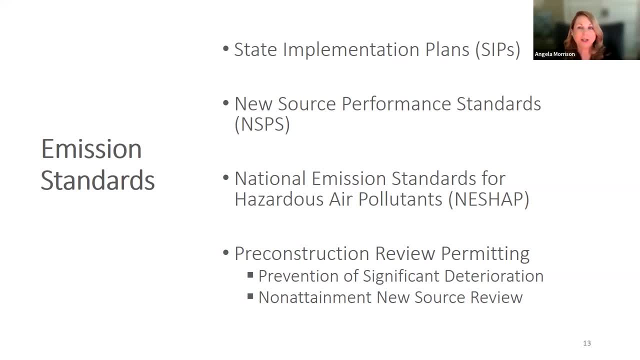 which is under cooperative federalism. new source performance standards, NESHAPs, the National Emission Standards for Hazardous Air Pollutants. I've listed these here just so you understand that there are just a number of different programs, including permitting. 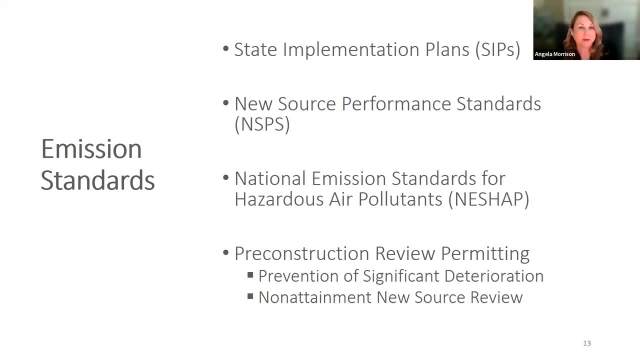 programs. So we'll get into some of those, And some of these are for hazardous air pollutants. I've listed these here just so you understand that there are just a number of different programs, some for HAPs and some for criteria pollutants. Next slide: 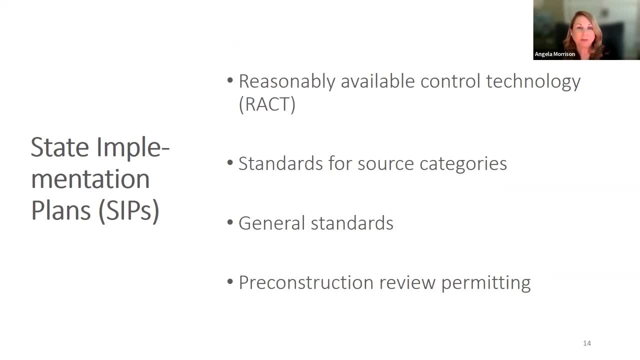 We'll start with state implementation plans. They can regulate emissions through different standards And you'll need to look at your state local program or even a tribal. I use the term state implementation plan here, but there are also tribal implementation plans And it's not. 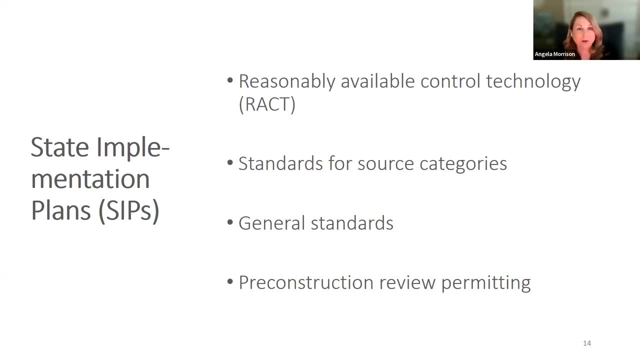 limited to state. Sometimes there are local programs, especially in California. You'll find those also in Tennessee. So you look to those local state tribal rules and you will find air emission standards that apply to stationary sources. And it also encompasses some of the permitting programs. Next slide: 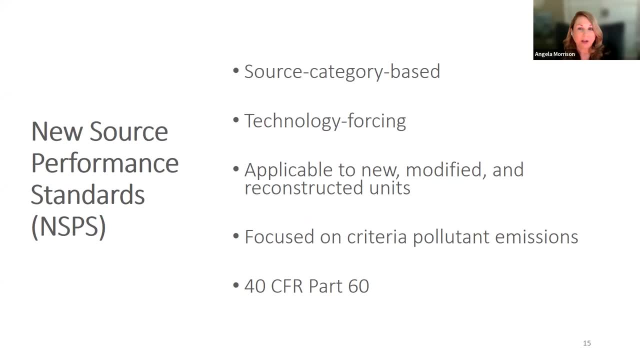 New source performance standards, on the other hand, are established by the EPA. They're proposed and there's an opportunity for comment, And then they're finalized And it's sometimes challenged, but they go into effect once they're set up, unless they're. 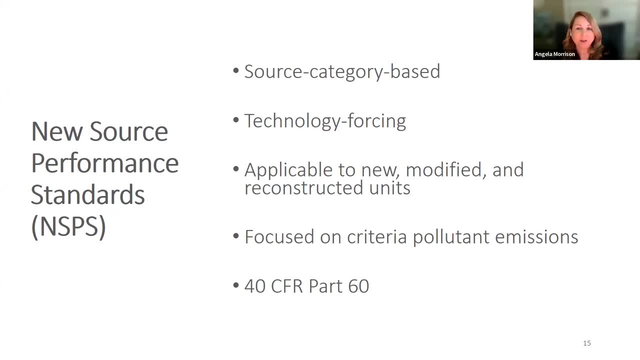 stayed by a court And then they're finalized, And then they're finalized And then they're set up unless they're stayed by a court, which has happened, And for the most part, the new source performance standards are established under the authority of 111 of the Clean Air Act. 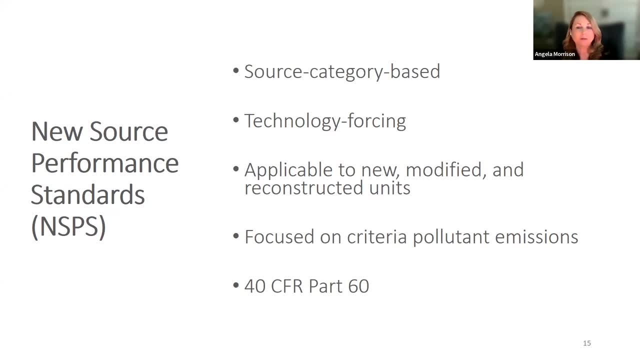 But it's a little bit of a misnomer. but they're also- and those are primarily for criteria- pollutants, the ones for which I had on the earlier list and that are subject to an ambient air quality standard. But NSPS standards under 40 CFR Part 60 also encompass standards established. 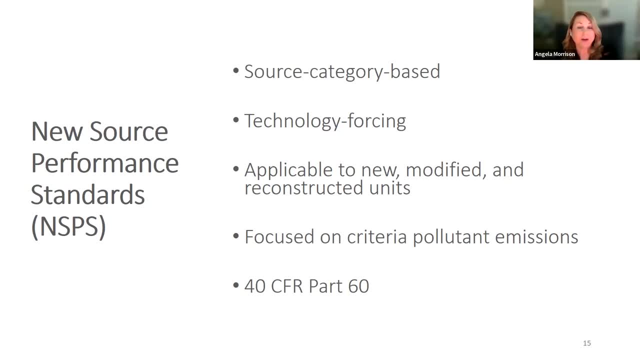 for solid and hazardous waste incineration units Under 129 of the Clean Air Act. new source performance standards, as the term implies, generally are focused on new sources. For the 129 standards it would be new and existing And for: 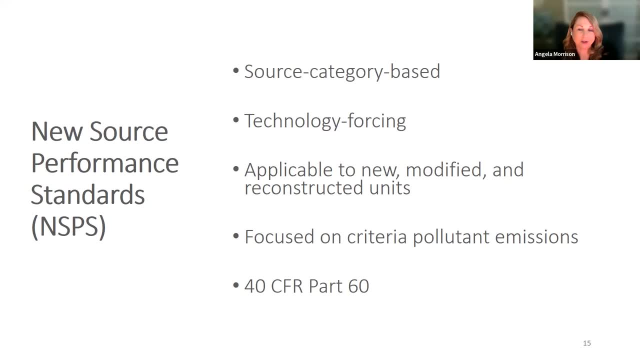 the existing sources. it's a guideline and implemented by the state. Too complicated to go into, but just know that there's a lot more to NSPS than oh. you just look up the rule and this sweat applies. They've also been established for greenhouse gases for certain categories, So 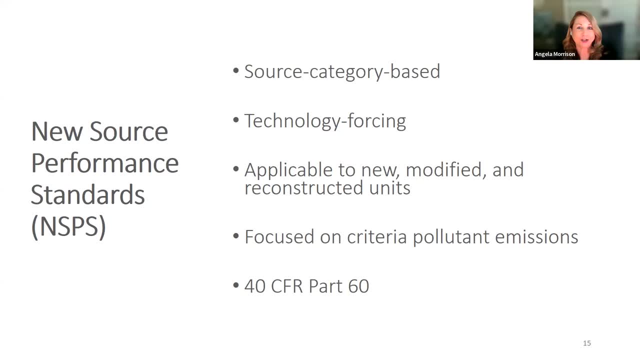 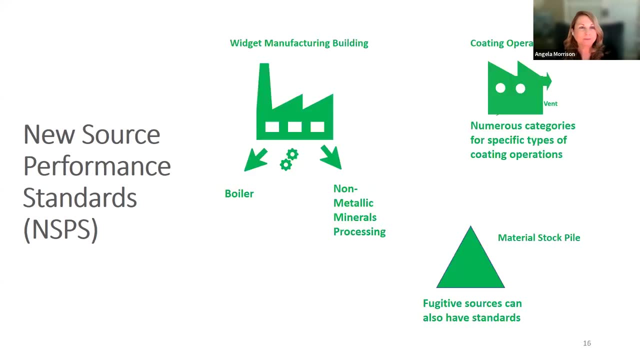 there's just a lot, And so you know I think it's a little bit of a misnomer, but they're different things going on. even though it's just supposed to be new source performance, standards, criteria, pollutants, it's grown much beyond that. Next slide There's a different. 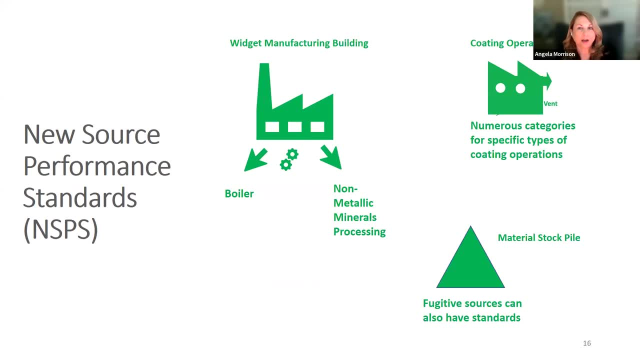 definition for stationary source under the under NSPS rules And it focuses only on the individual unit really. So even within a building it says building, but it's not usually the entire building. You look and you know you look at the building, you look at the. 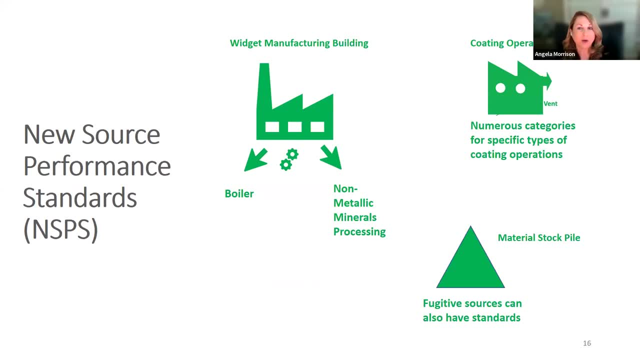 building. you look under the tent and what's in that building? There's a boiler that might be subject to one NSPS. There's a non-metallic mineral processing that might be subject to a different NSPS. Then you go over to another building. the coding operations there could be. 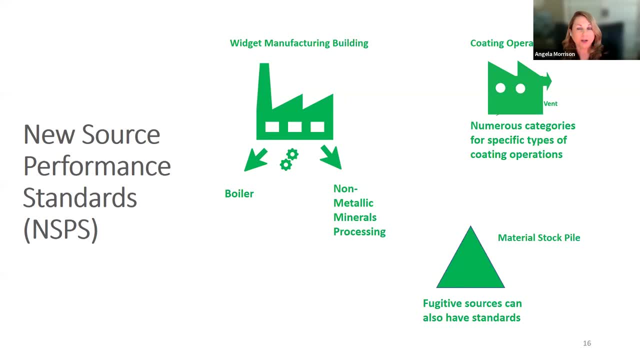 a half dozen different standards that apply to different coding operations within that building And, interestingly, fugitive sources can also be covered by a new source performance standard. And, as Suma mentioned, these are technology forcing, meant to make sure that, if you're 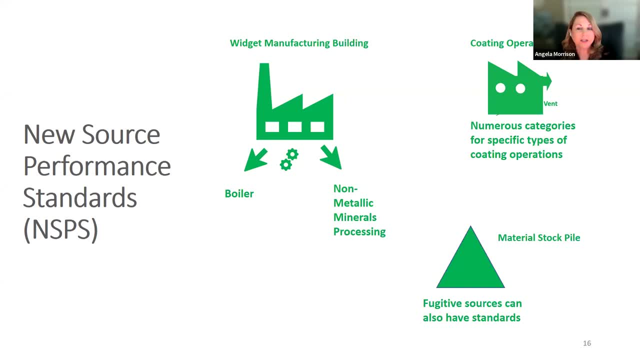 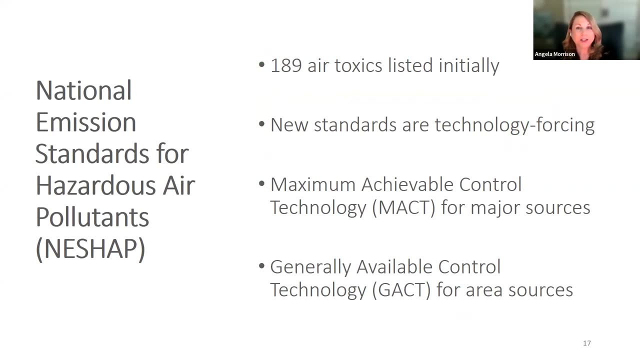 investing in equipment, putting in a new facility that you're using, state-of-the-art equipment. Next, slide Switch gears to hazardous air pollutants. As I mentioned there, there originally were 189, there are 187 now, And before the 90 amendments, EPA had established HAP regulations. 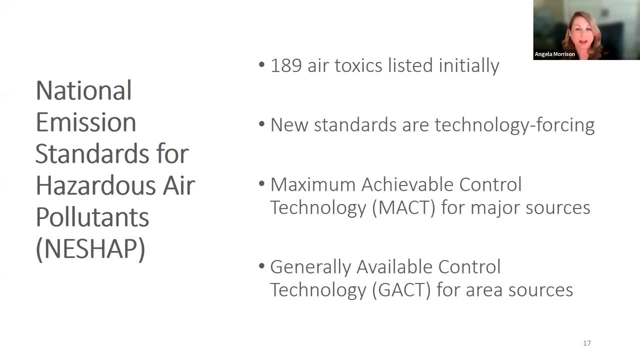 based on human health effects, going pollutant by pollutant, And they had only managed to come up with a handful of standards by the time it was approved. And so you know, it's a, it's a, it's a 90 amendments. So the 90 amendments changed things significantly, changed the process to be. 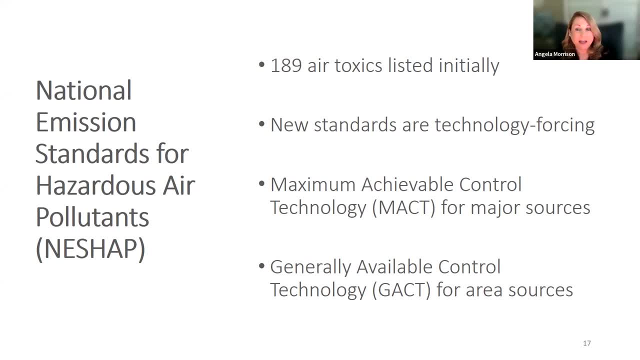 technology forcing, and EPA set about to establish standards, category by category. Now I counted at least 144 source categories that have been regulated, And it's not just for new facilities or new sources, it's for existing sources And even- and they have different thresholds to be. 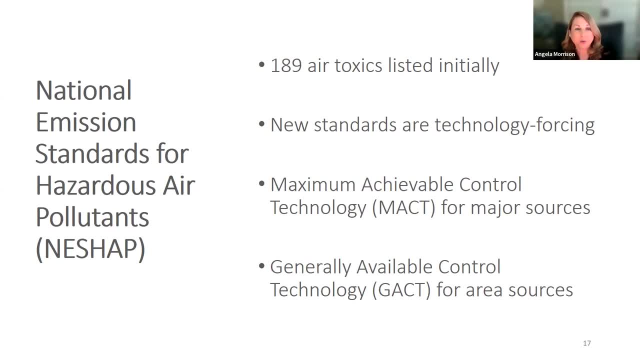 regulated, but they're the same level of emission control if they function. in the HAP area There are standard that apply to the area non-major sources as well, usually less restricted but sometimes the same level of emission control depending on the source category. So a lot has. 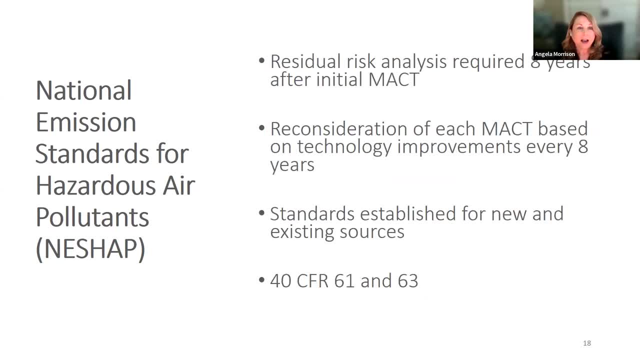 changed. with regard to HAP emissions- Next slide- And it hasn't stopped. While it took about 20 years to get the first round of MAC standards on the books- next slide- It didn't stop until about 20 years, And you know it probably stopped because we don't have an Mills and Sommers' country right now. but it hasn't stopped. While it took about 20 years to get the first round of MAC standards on the books, Next slide Now. the main factors for that are: there's information from the city management that might have had an impact. 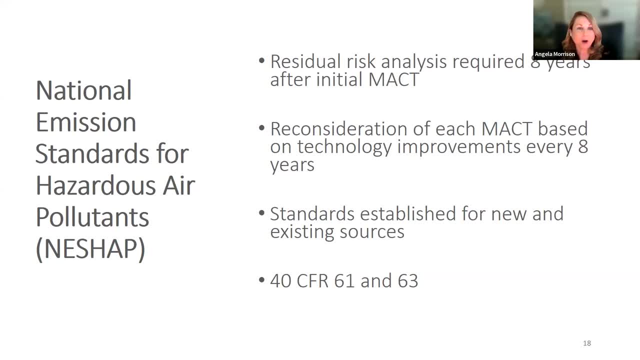 Now it's time for the residual risk analysis that's required only one time, apparently, after the first eight years after a MACT has been established, And that's to take a look at now that you've forced the technology and you've basically. 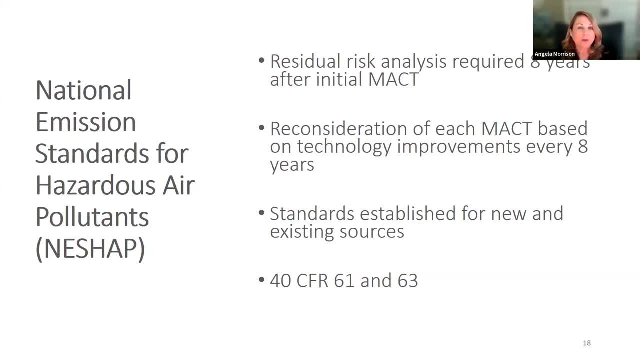 looked at the best controlling sources around. are you protecting human health from these hazardous air pollutant emissions from a stationary source that's applied the MACT control requirements? You know they're meeting the MACT emission standards. Is there still a risk to human health? 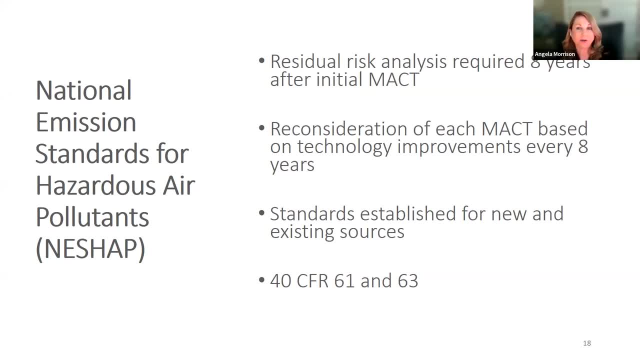 And sometimes that has been the case, And so they've lowered the standards every eight years, not just a one-time deal. They have to look at whether technology has changed and whether the technology has improved so that they need to lower the standards even more. 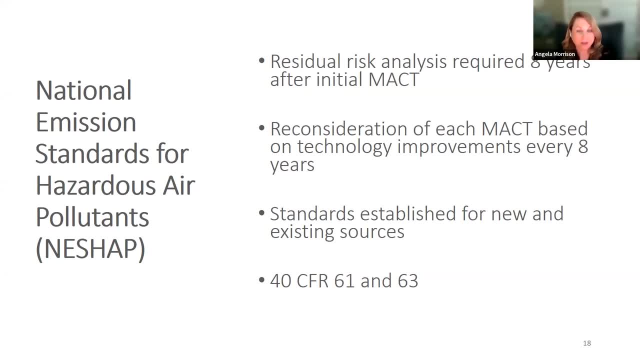 And that's supposed to be recurring every eight years. They're behind on some source categories, Running a foul- Some of the NGOs who are taking issue with that, But this is a way to keep these standards current and state-of-the-art. Next slide. 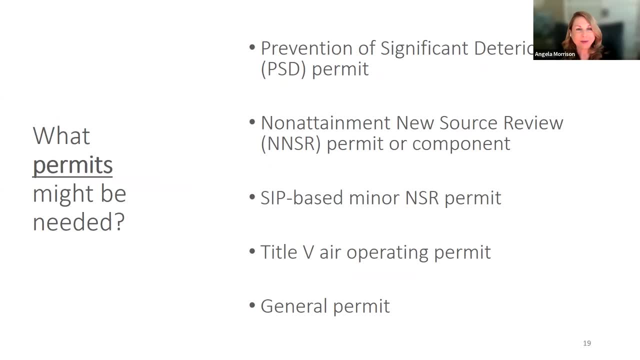 So, in addition to all the standards that apply, you might need some additional permitting for your stationary source. There are a number of different permitting programs out there. There are very few air emissions sources that aren't subject to some kind of permitting, And one of the important distinctions as to what kind 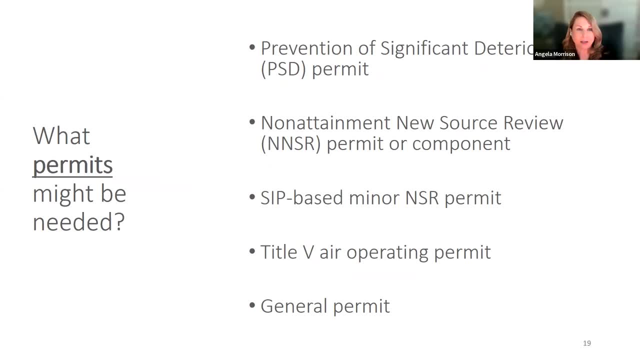 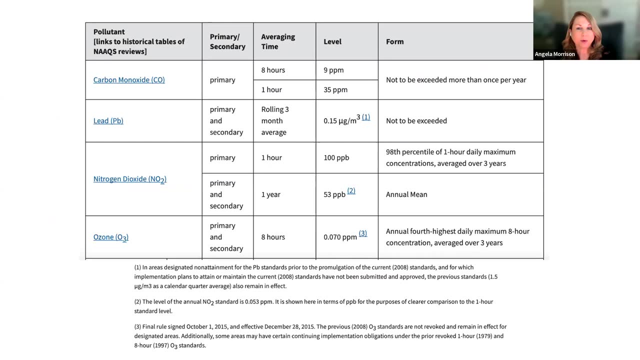 of permit you'll need is based on whether the area is in attainment or not in attainment, And SUMA set this up for us. Next slide, There are ambient air quality standards for the criteria pollutant And if an area And these are health-based standards based on this list of six criteria pollutants. 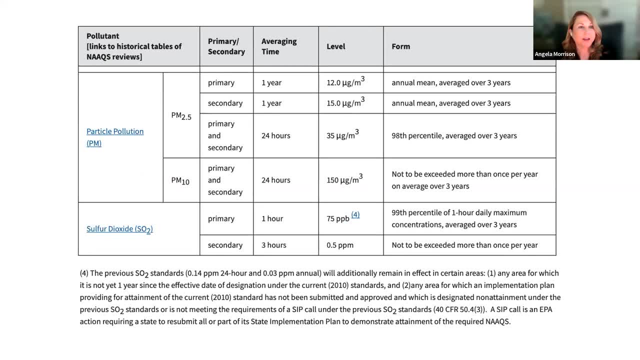 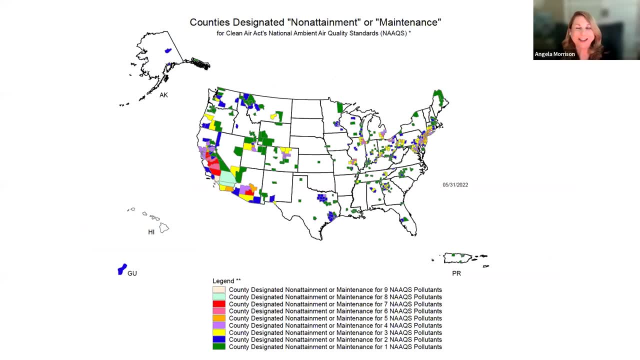 Next slide. This is the remaining two, I think. Next slide: Oops, Anyway, there is a list- You'll You'll see if you get the slides- that goes into all six of the criteria pollutants, And this map shows the areas of the United States that are not in attainment with one. 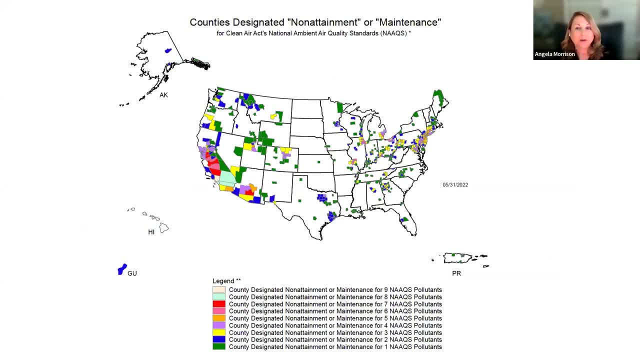 or more of the ambient standards And it also shows the areas that are maintenance areas, where it has been in non-attainment in the past and they need to pay attention to make sure they don't go back into non-attainment. If an area is in non-attainment, different non-attainment, new source review rather than PSD. 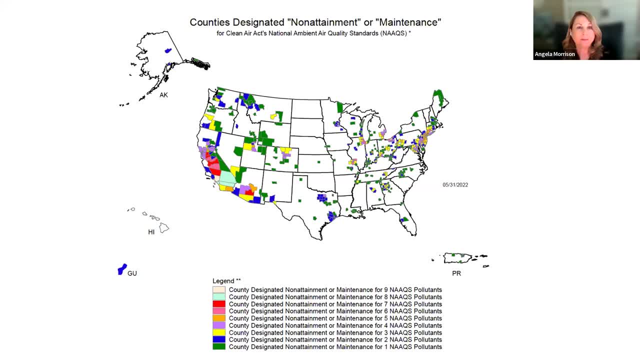 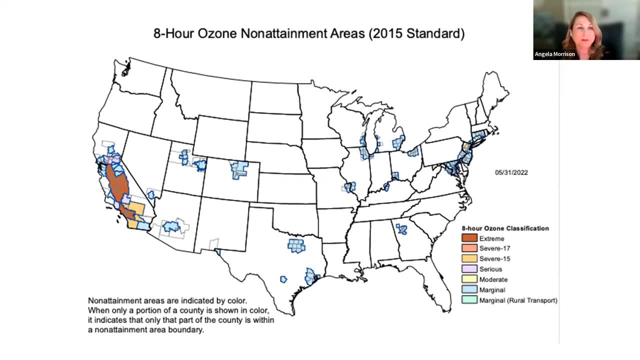 review can be required for that pollutant Next slide. Ozone is one of the most common types of non-attainment areas And so much so that there are different levels of non-attainment, ranging from marginal to extreme, to identify that every non-attainment area for ozone is not the same. 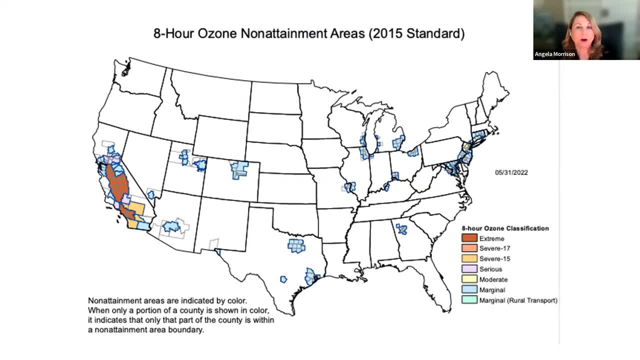 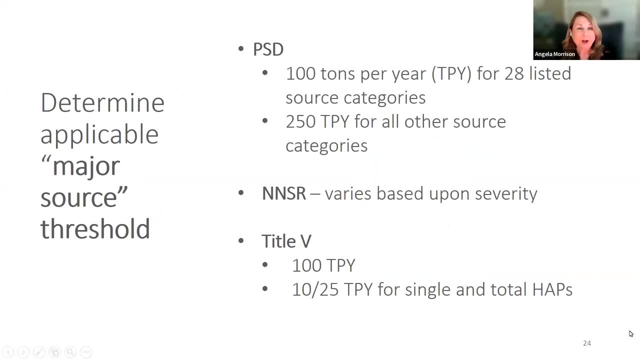 Some are Will take longer to get into attainment And the requirements are less stringent than the ones that are only marginal. Next slide. And of course you know there's a variety of different major source thresholds under PSD. Sometimes it's 100 tons per year and it's for 28 listed source categories. 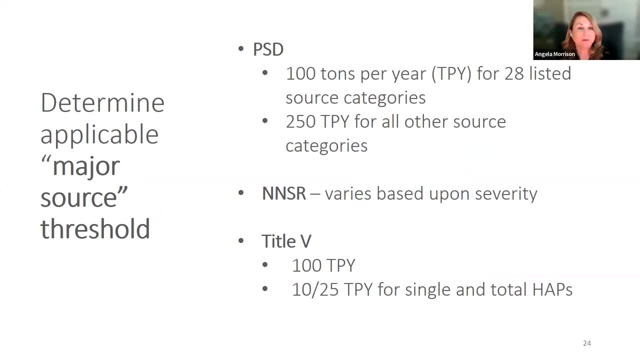 Sometimes it's 250.. For non-attainment, it might be 25 for an extreme non-attainment area. for ozone And, by the way, for ozone they regulate the precursors, which are VOCs and nitrogen oxides. 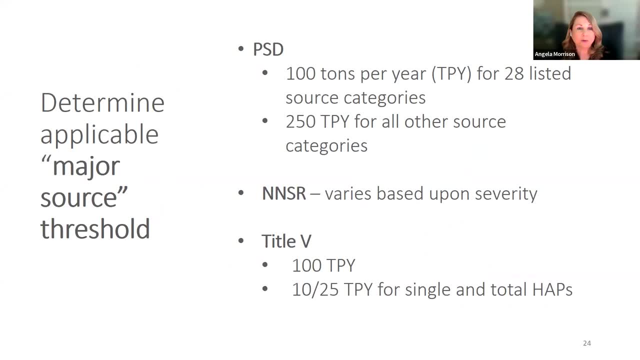 But non-attainment new source review have pollutants over 25 tons per year Could trigger major source status. and for title five permitting, which I'll touch on toward the end, There's no 250- 10 threshold, It's 100 for criteria pollutants and most regulated non-hat pollutants and then 10 to 25 tons for single and total hops for title five. 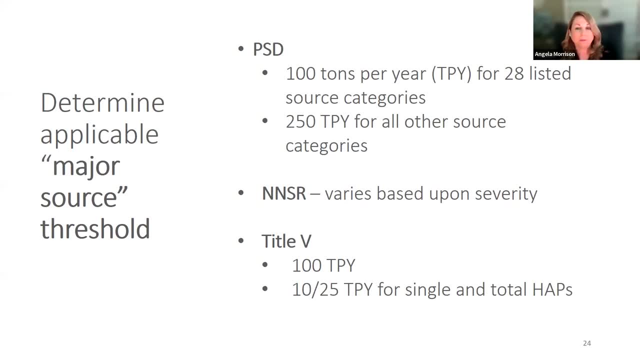 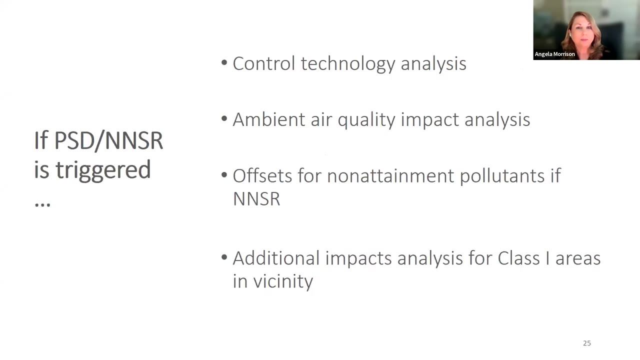 And most are. all of these definitions are site-wide contiguous: common control, and sometimes fugitives count And sometimes they don't, So you'd have to look into that in more detail. Next slide: If PSD or non-attainment new source review is triggered, a fairly extensive analysis is required, with a number of components listed here. 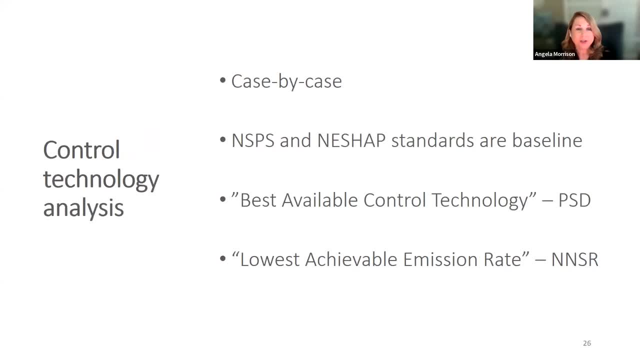 Next slide For those stationary sources that you might have already identified are subject to a NESHAP or NSPS. they still might be subject to this control technology forcing case-by-case analysis, And sometimes they don't, So you'd have to look into that in more detail. 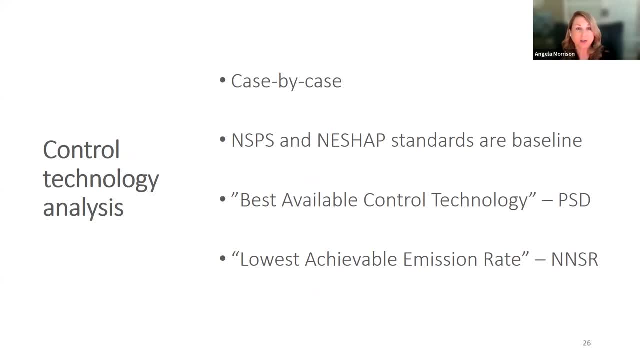 Next slide. Next slide For those stationary sources: either best available control technology, where costs are taken into account, or lowest achievable emission rate, where they're not necessarily taken into account, And at a minimum you have to meet the NSPS. but it's usually a one-way ratchet to lower the emissions based on the newer technology that's out there. 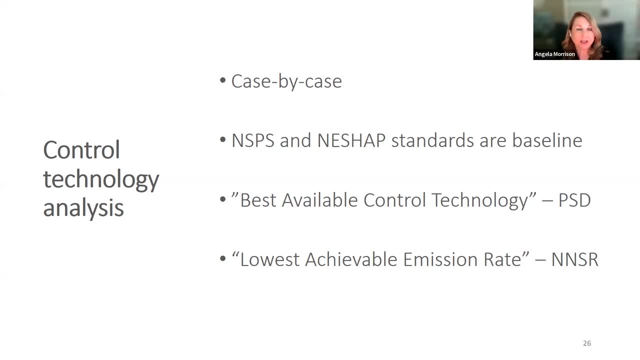 Mainly because it takes so long for EPA to do a rulemaking that the NSPS and NESHAP standards can't keep up with the newest technology. So they have, at least for criteria pollutants This way, to require case-by-case before you spend those capital dollars to make sure you're getting state-of-the-art equipment to minimize emissions. 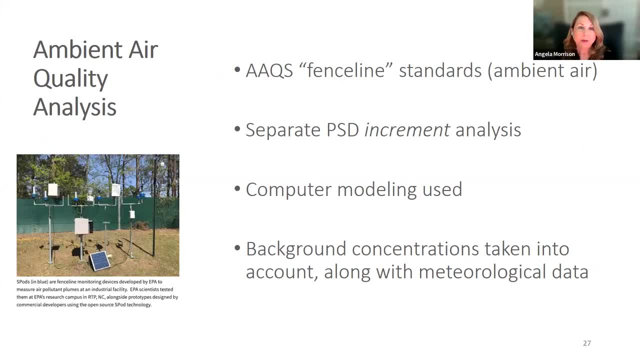 Next slide. So, regarding the ambient air quality standard analysis, this is at the fence line and there's one for the ambient standards themselves, another for PSD increments, which I'll get into- I'll show you a slide on that- And this is done through computer modeling and the models change all the time and there are different ones for different pollutants. 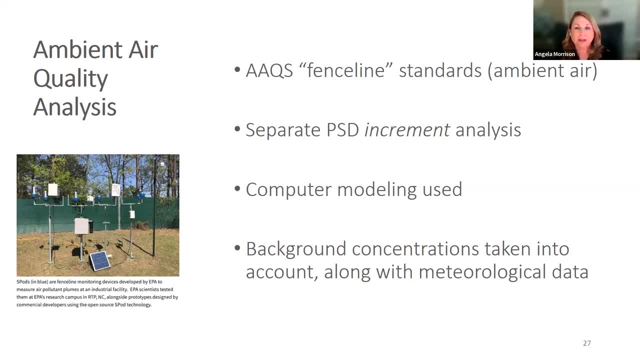 And different transportation links and things like that, And they do take into account local meteorological conditions and background concentrations. In the photo on- well, I don't guess you're necessarily seeing the photo, but I had a photo of an ambient monitoring station. 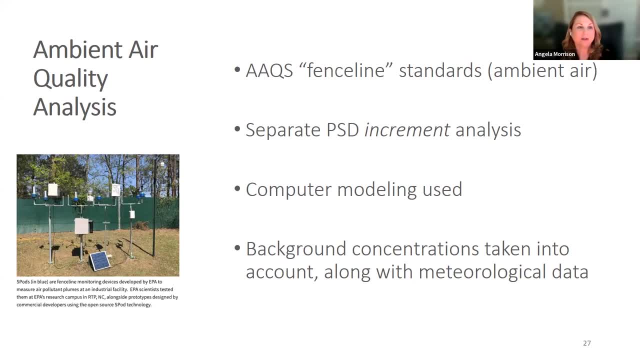 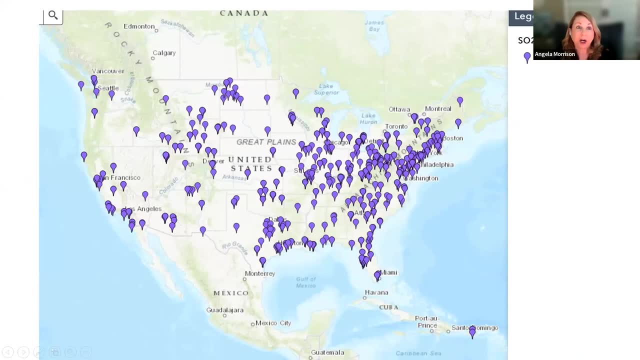 And the next slide shows the monitoring stations all across the United States. And this is for SO2 and you can see that there are a lot of monitoring stations, but there are some areas you know whole states. And this is for SO2 and you can see that there are a lot of monitoring stations, but there are some areas you know whole states. 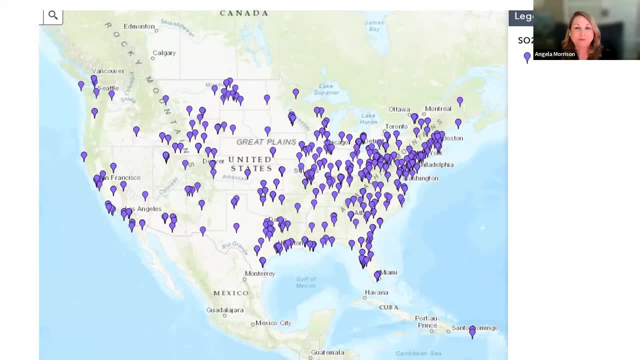 That don't seem to have any monitors, And so if you're placing a facility in one of those areas, you might have to go take your own background readings. This is also why some areas of the country will be unclassifiable for a pollutant like SO2, because there's no monitoring data to know whether it's in or out of compliance with the ambient standard. 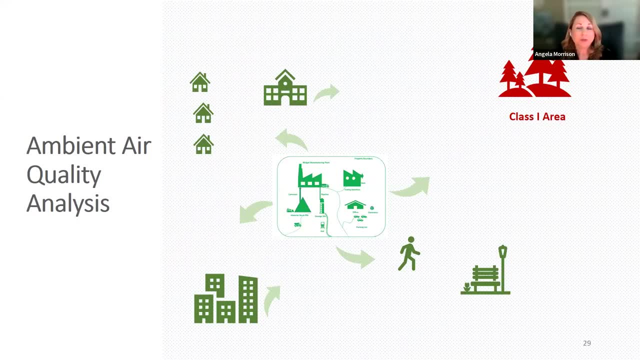 Next slide. So this is really where you take your source, which I have, you know, our little widget facility there in the center And taking a look at its emissions, And taking a look at its emissions Under different meteorological conditions and impact. on the nearest neighborhood there might be an industrial facility like I have here to the north. it's also has air emissions that might need to be taken into account. 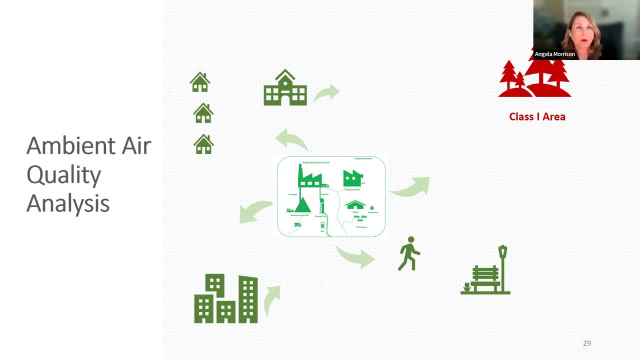 And you have to look at your fence line and even though it might be a road that no one could actually live on, so they're not exposed on an annual basis 24 seven, you have to assume that that's a possibility You could also have. 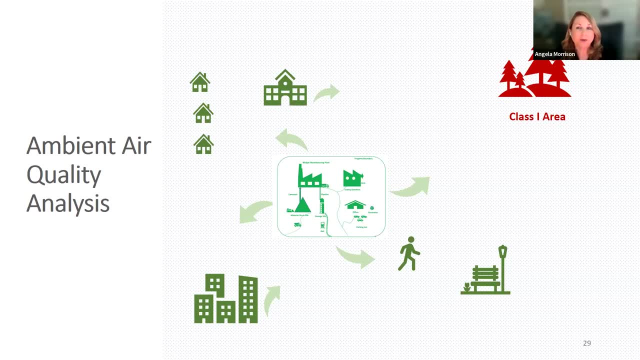 A class one area that's nearby that you need to take a look at and, as I'll show you the PSC increments, they are lower and they're also different ambient standards that you need to take into account, so the modeling will be different for class one areas. 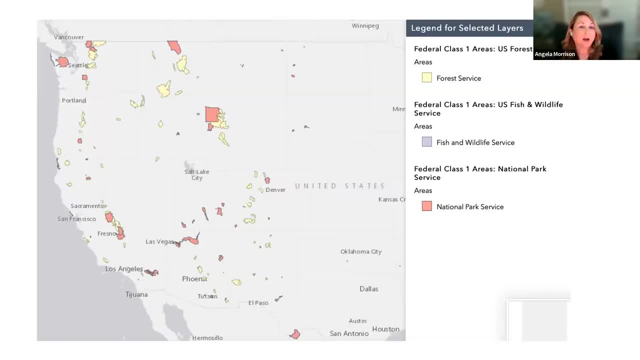 Next slide. This map shows some of the class one areas in the western part of the United States, so wherever your facility is, you need to take a look and see what's on that list. These are, These are. These are national wildlife refuges and national parks of significance where we want the air to maintain a more pristine quality. 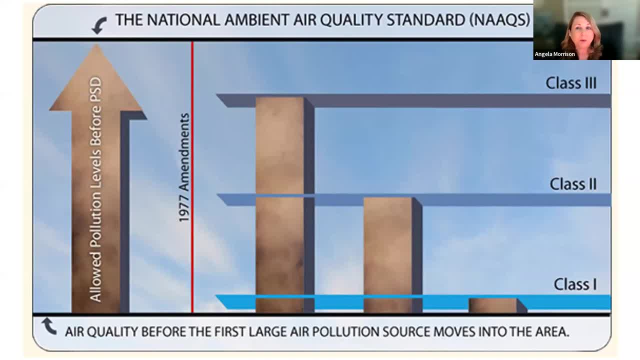 Next slide, And some of this is done through the PSC increment program that was set up in 77, where Congress wanted to make sure that all of the air quality in the United States- and I'll go all the way up to that borderline- of healthy, unhealthy 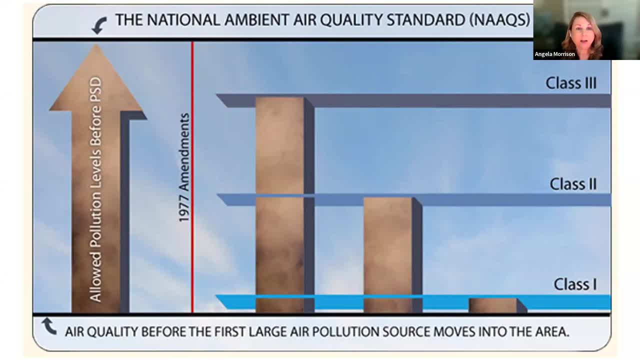 If it, if an area had fairly good air quality, They wanted to allow some margin for economic growth. but they didn't want that group to take the air quality all the way to near unhealthy levels. So it shows here the ambient standard is based on that arrow on the far left. They're really no class three areas. so you know it's on the books, so it's on this EPA slide but it's not. 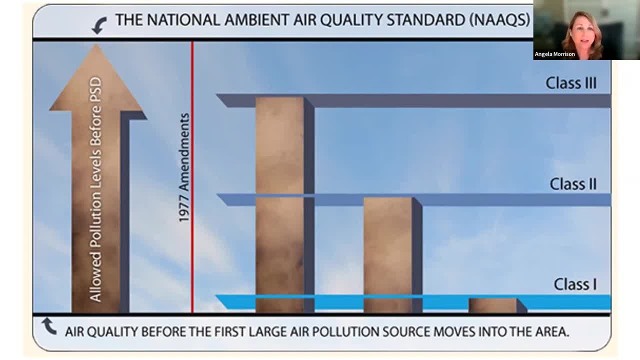 It's not really relevant. most of the countries a class considered a class two area. And then we have the national parks and wilderness areas that have been set aside as the class one areas. So in a class two area you take your baseline air quality and you add an increment above that, but you don't get to go all the way to the unhealthy level. 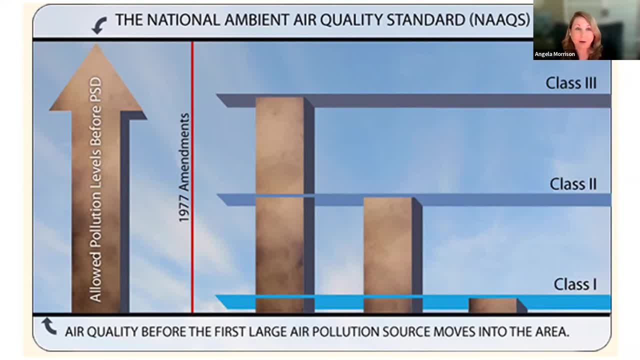 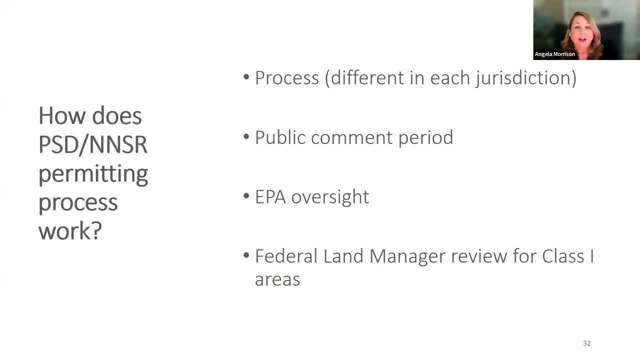 And then for the class one areas, you can have a little bit of growth, but not very much That impacts that class one area. Next slide: So how does this PSD, non attainment, new source review permitting process work? Next slide: So how does this PSD, non attainment, new source review permitting process work? Well, there's no easy answer because a lot of times it's in a state implementation plan. sometimes the programs are delegated, sometimes they're approved, meaning the state uses its own process and that 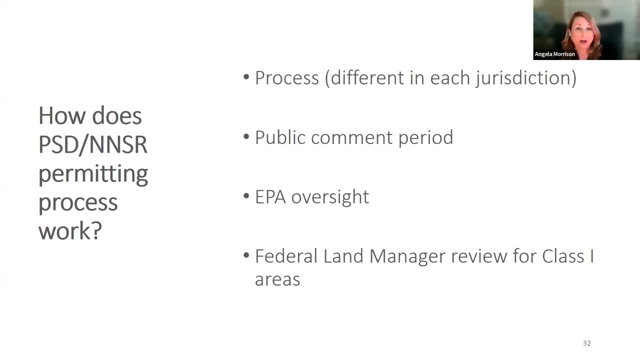 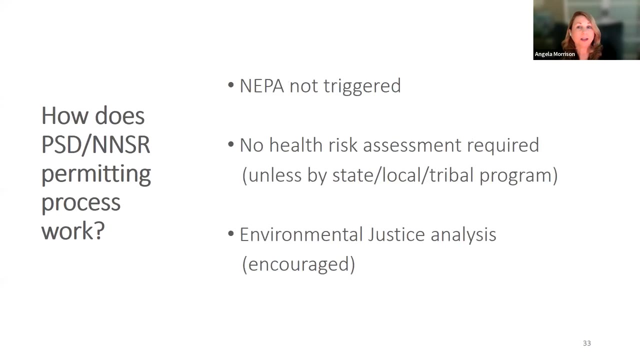 would be different in every jurisdiction, but there's always a public comment period, there's always EPA oversight And if you are impacting a class one area, you'll also get federal land manager review of that application and proposed permit. Next slide. Next slide. 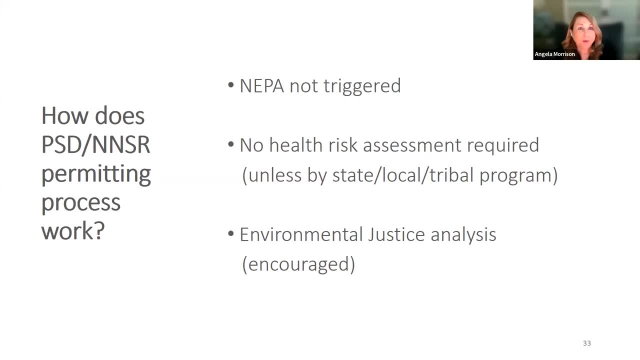 And then a little bit of information about the process. So, in terms of the process and how we address it, I'm not sick. Interestingly, and something to keep in the back of your mind, if you've just gone through law school and you know all about NEPA, well, NEPA, it's not triggered by a Clean Air Act permit. so if you scratch your head and wonder why are we not talking about me? but it's not triggered and there's no health. 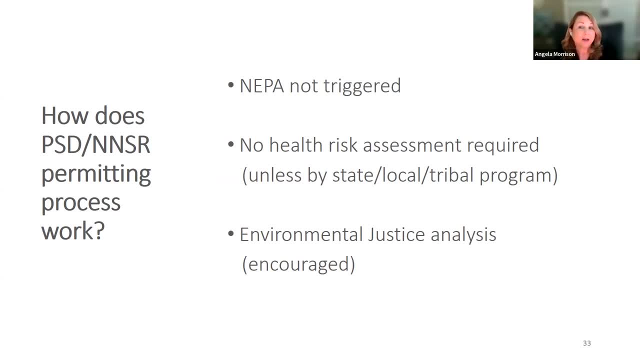 risk assessment required, except that is a requirement in some state and local jurisdictions and some even some tribes. and environmental justice analysis is encouraged but not required, and EPA has recognized that. you know they may not have all the tools, but there's always. some is encouraged but not required, and EPA has recognized that. you know they may not have all the tools, but there's always some good practice and sometimes people will just get stuck in one of the shortcomings. 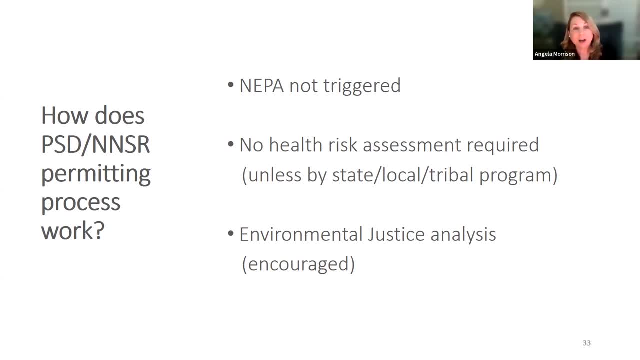 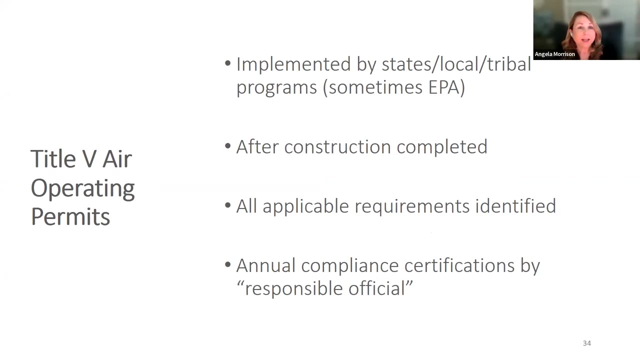 they may not have all the tools but they're leaning on states and tribes and local programs to fill in that gap, to maybe take a look at environmental justice concerns, especially with the new greenfield site next slide. so once you get your facility permitted and it's all up and 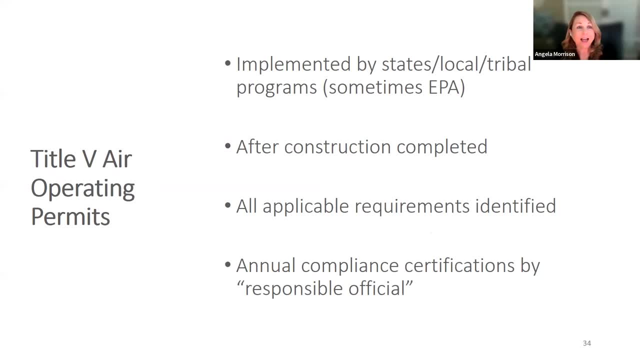 operating you'll need a title vi, their operating permit, and these are. this is a fairly mature program. it started with the 90 amendments because previously you just had your psd permit that might be issued and you operate for 30 years and there was no requirement to put that in an operating. 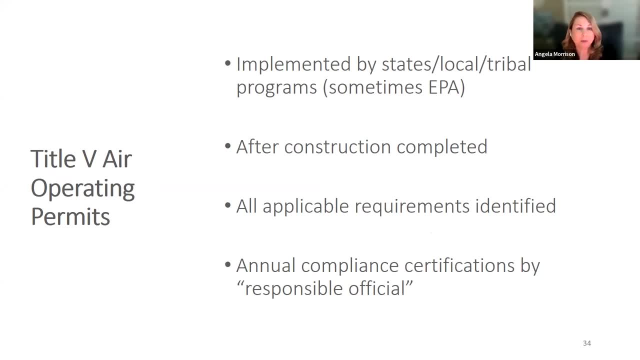 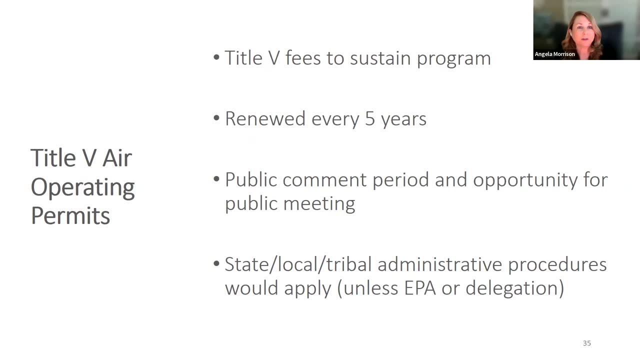 permit. there is now, and the thought was to have all the applicable requirements in one place to make it easier for compliance. and it's next slide: it's self-funded. you have to pay title fight fees based on your emissions. these are renewed every five years, so there's always a title v. 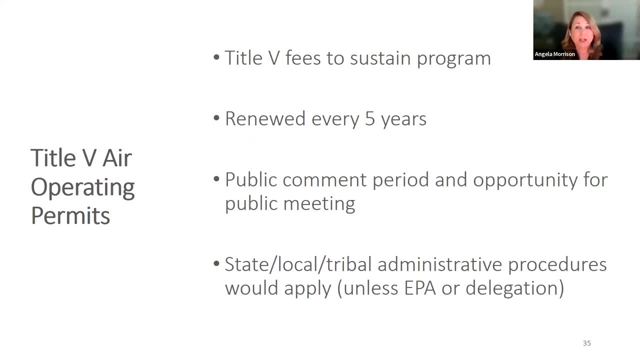 permit for the major sources. there's also an opportunity for comment and an opportunity to request a public meeting, and the title v operating permits are primarily implemented by the states. there are a few situations and tribal areas and for outer continental shelf, or it might be issued by epa, but for the most part it's it's done by state. 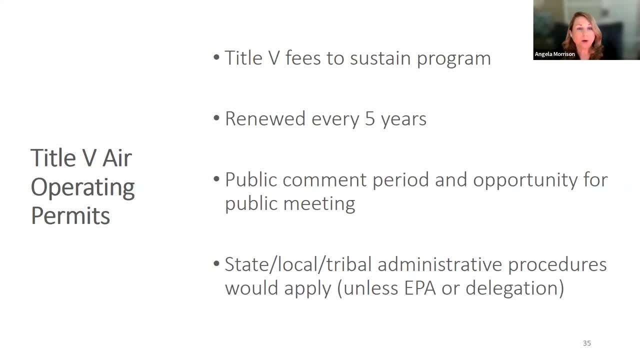 local and tribal governments, and so they'll use their own uh procedures and and these programs can also be approved or delegated. for the most part, approval uh was already established before. the delegation was an option, and most recently these have been. there have been, there's an opportunity if epa- epa has oversight here too and they have a 45-day objection period, and if 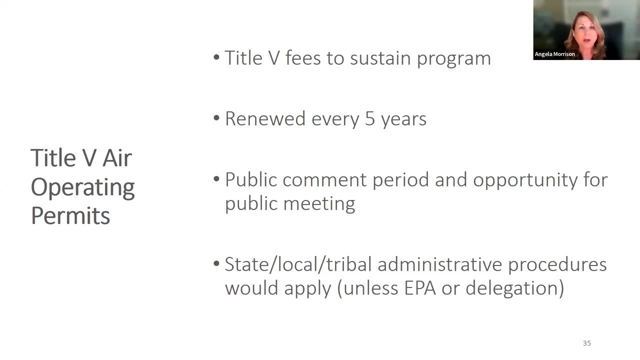 they don't object within their 45-day period. within 60 days, an interested party can request a file petition with epa, requesting that epa object, and there have been almost a dozen of those petitions this year. most of most- all of them, i believe- have been filed by non-governmental organizations or citizen groups. 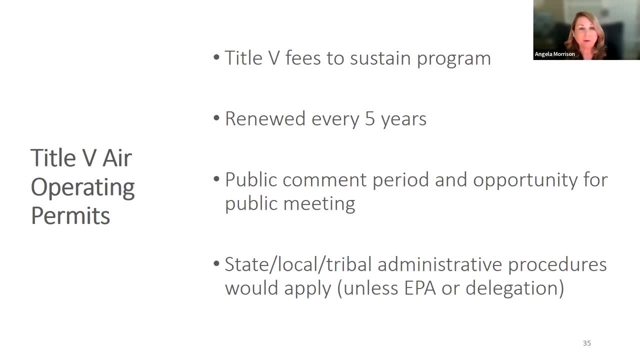 requesting and petitioning epa to object to these title v renewals based on environmental, justice or other local concerns like that, and so this remains a very interesting program and a way for the public to continue to have an opportunity, uh, to participate in in what's going on with the facility in their area. next slide: 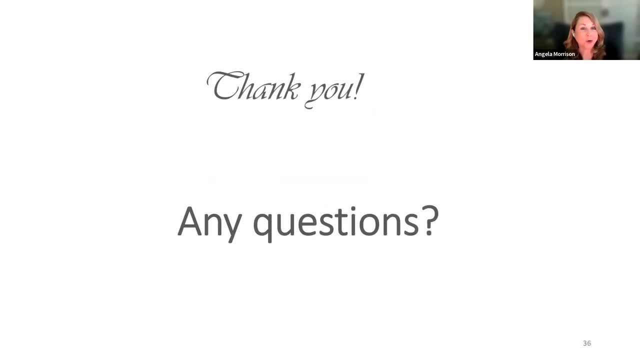 i think that's it, so i don't know, assuming how you want to handle it. yeah, questions now. yeah, let's, if you don't mind, angela, let's hold off on audience questions to the very end. thank you for that wonderful uh presentation just to, and thank you for highlighting the ways in which 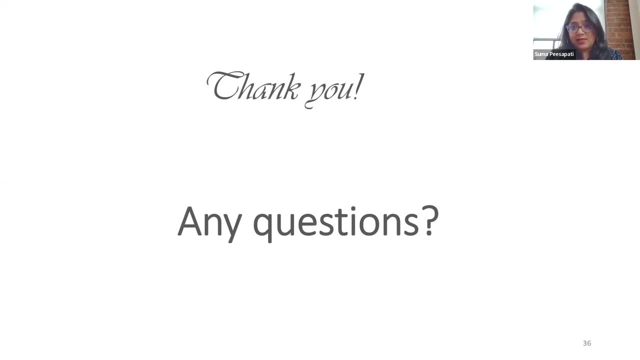 the clean air act does address um existing sources. in fact, you know the the hazardous air pollutant provisions and protection of class one areas under the regional haze provisions of the clean air key strategies and reducing pollution from the coal fire power plant sector have been key strategies. 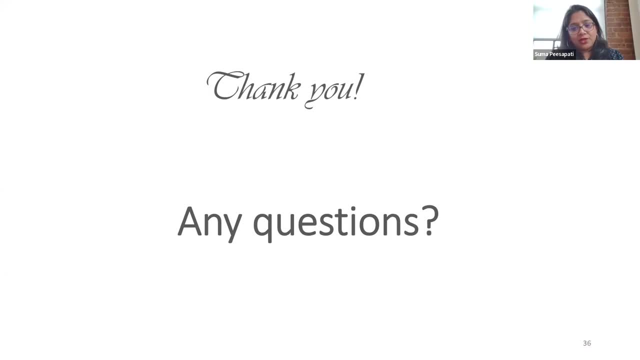 and also the risk management plans in terms of um addressing uh potential risks from accidents, upsets at industrial sources and the requirement that there be a root cause analysis when in in the wake of a of a upset. um, those are all really critical provisions and thank you for uh that. 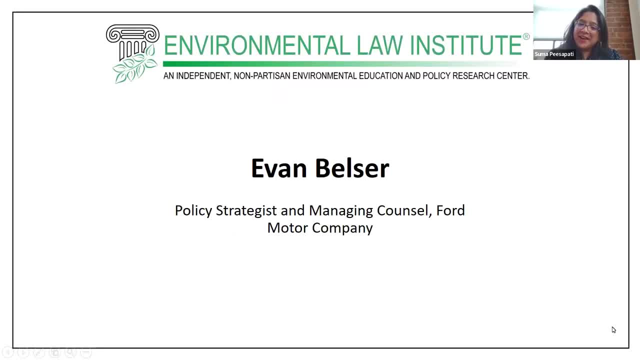 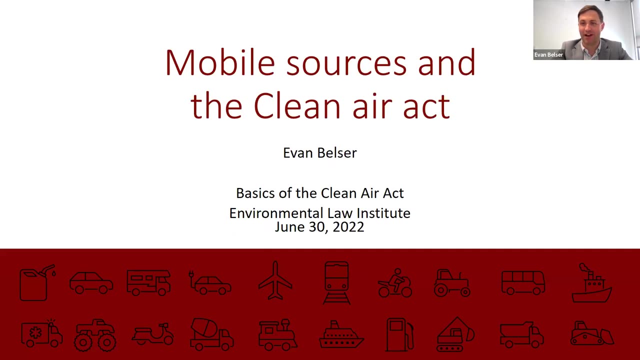 deeper dive and with that i will turn it to evan to talk about um half of the equation, uh, mobile sources. thank you very much. uh. next slide, angela. hats off to you. uh, that was a tremendous amount of content that you you got through in in quick order. um people. 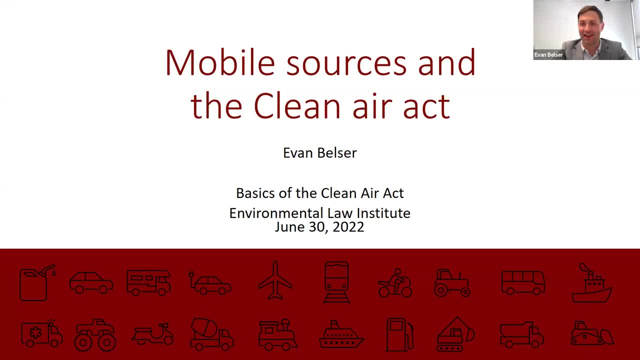 have spent their entire careers on just this or that slide. uh, in your, in your presentation, i just want to underscore the breadth of the act, um, and so i'm going to focus on mobile sources and it actually i'm going to give you a couple of slides, um, so, uh, it's a really interesting slide, i think. 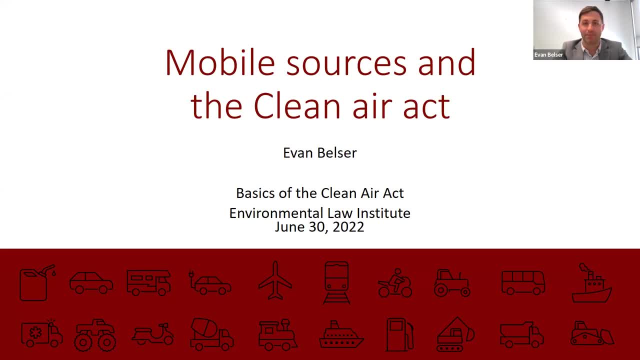 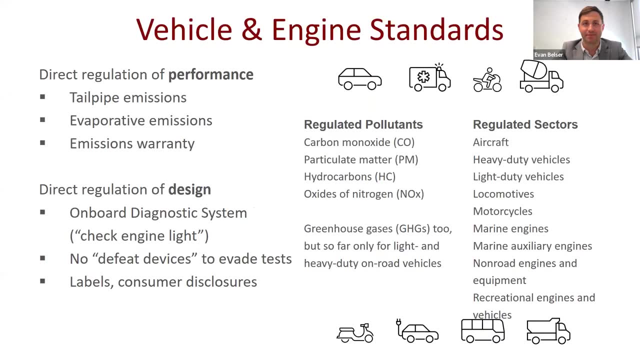 that you will see more of it in the next slide, but i'll just start with the, the um, the uh uh common principles of the clean air act, and i'm going to go ahead and start with the clean air act. um so, um. more specifically, i'm talking about the clean air act and there are some real 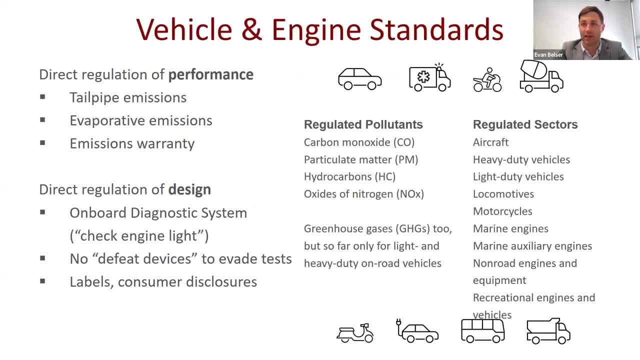 similarities. there are some real differences to the stationary setting and so i'll be touching on those throughout. but it's in title two of the clean air act and concerns vehicles, engines and fuels. next slide for evaporative emissions. Fuel, literally evaporating off vehicles, does contribute It. 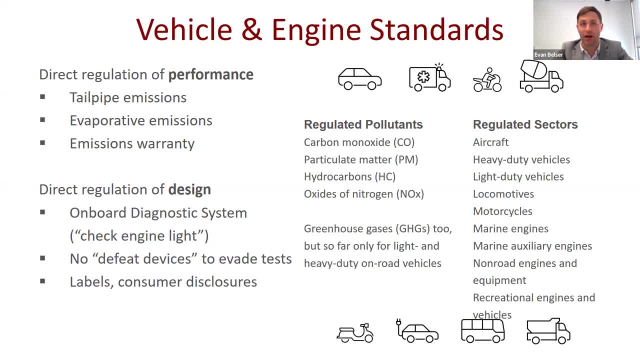 adds up, And so there's standards there as well, Also on performance. it's not about just being a new clean car. It needs to remain clean, And so there's emissions warranty and other in-use requirements to be sure that the vehicles remain clean for a regulatory period of time. 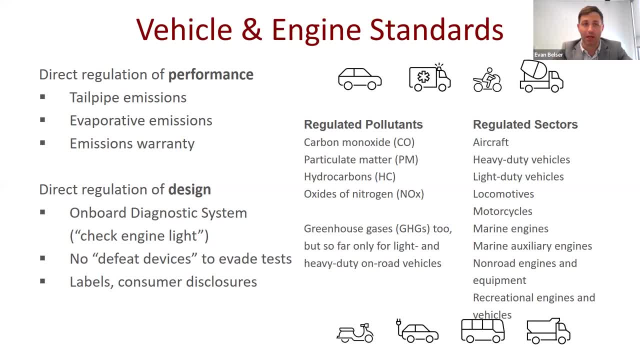 There's also direct regulation of design. So the Clean Air Act doesn't say just exactly how to build, and the regulations don't say how to build your vehicle or engine. Rather, there's a lot of deference to the manufacturers: how to meet the numeric. 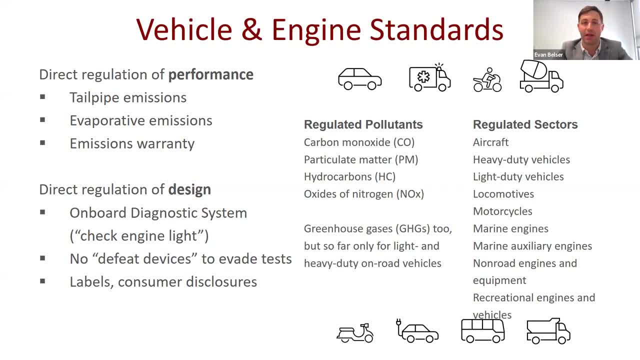 standards, how to meet the performance standards, But there are some aspects that are specifically stated in terms of design, So there needs to be, for example, an onboard diagnostic system. This is an extremely complex system That has sensors all over your vehicle and ensures that there's proper information on 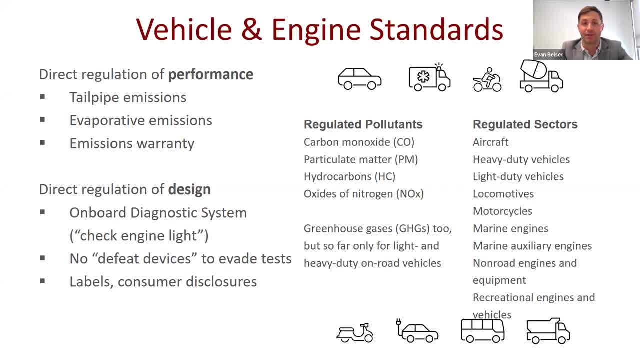 the operation of the vehicle and its emissions control system. That's useful for a lot of reasons, but ultimately to keep gross emitters off the road. Another design requirement is that the vehicle needs to be built like you said it was. There can't be defeat devices. We'll talk. 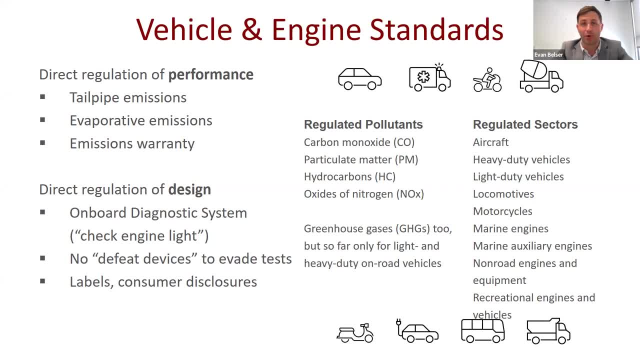 a little bit about that. And there's other elements of the program, including labels to help technicians or anybody understand What technology is on that vehicle for maintenance, for repair, things like that. And there's also consumer disclosures, which are important as well, including fuel economy. 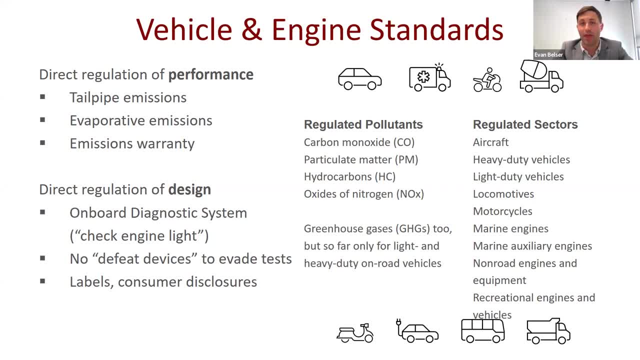 And so what are the pollutants? Many of the same that we've already heard about: Carbon monoxide, particulate matter, that's especially for diesel, hydrocarbons and NOx. Greenhouse gases are regulated, just like these other pollutants, in mobile source context and have been since 2011.. 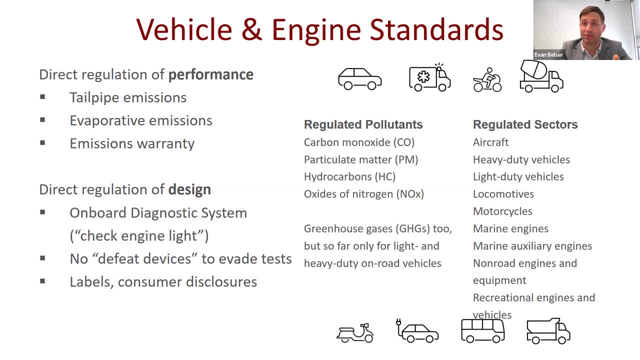 Literally the exact, the just another on the list of regulated pollutants. And they show up in the same way in getting your vehicle certified for sale, But so far only for light and heavy duty on road vehicles. Lots of sectors that all use internal combustion engines for mobile sources, And so, bit by bit, 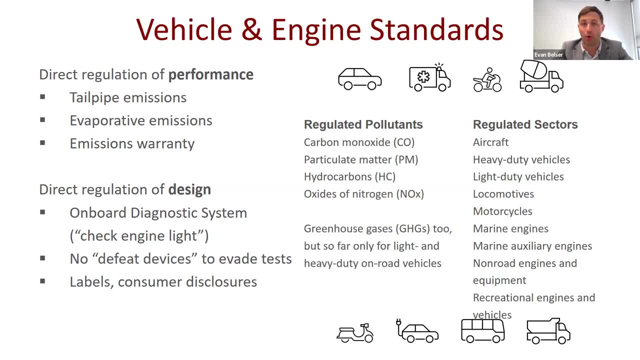 Congress directed and EPA implemented standards for each of these. You'll see that they all have the same basic framework but it ranges from. the original act said everything on the road- cars, trucks, buses, motorcycles. And then in 1990, Clean Air Act said: go EPA, study non-road sources and see whether they contribute. 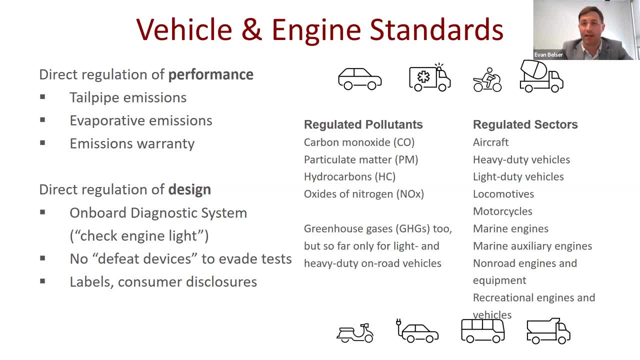 to human health or environmental risk And, if so, regulate those two. And there have, since the 1990 amendments, been bit by bit additional regulatory requirements, certification requirements and tightening of standards on things like marine engines, locomotives, lawn and garden equipment, ATVs- all of those things are also under Title II. 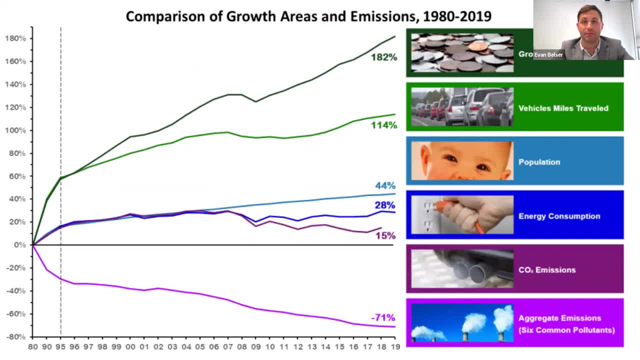 the Clean Air Act. Next slide: Michael Y, Harvard Law Institute and the Senior Answering ró buttonции u France. I like this from the EPA. It helps to show in one slide a lot of different things, including how far the pollution control has come on mobile sources. 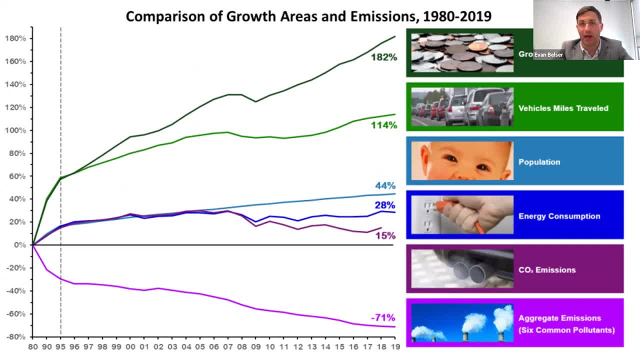 And so in the- you know this is transportation only. So, as a GDP has gone up a whole ton on the 182%, and vehicle miles traveled has also increased dramatically. since the 1980s We've seen overall significant reductions in criteria. emissions, particulate matter, NOx, CO, HC. 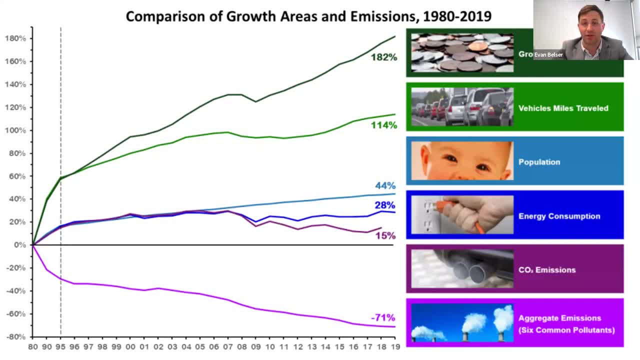 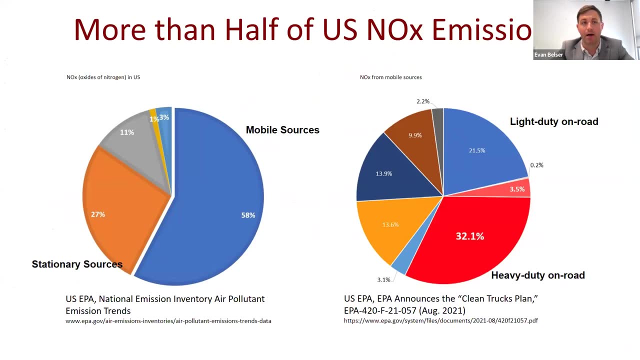 And that's due to a lot of modern controls on these vehicles and diligent oversight of vehicles in use to be sure they stay clean. Next slide, A lot of attention is paid to stationary sources. appropriately, Stationary sources present, as Angela described, a range of potential risks to people and the environment, including hazardous air pollution that can be acutely dangerous to people. 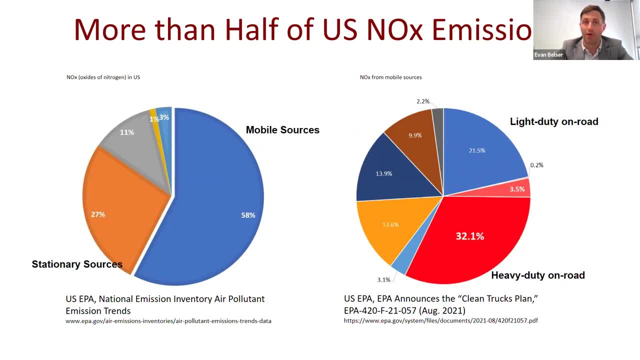 Mobile sources not that way so much. There are fewer pollutants at issue, but they add up, And so, when it comes to NOx emissions, which are a major precursor For ozone- ground-level ozone, which is bad for people, takes years off their lives- mobile sources are most. they make most of the NOx in the country as compared to all other sources under the Clean Air Act. 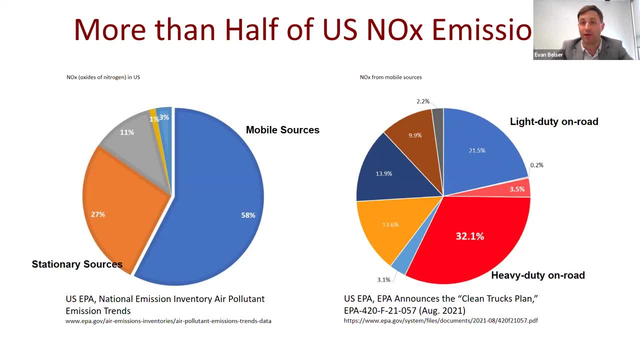 And when you break, that's on the left side. there On the right side, you'll see where the NOx comes from: primarily heavy duty on road and light duty is a second place And there's a lot of other sectors there that are other regulated sources like marine, like non-road. 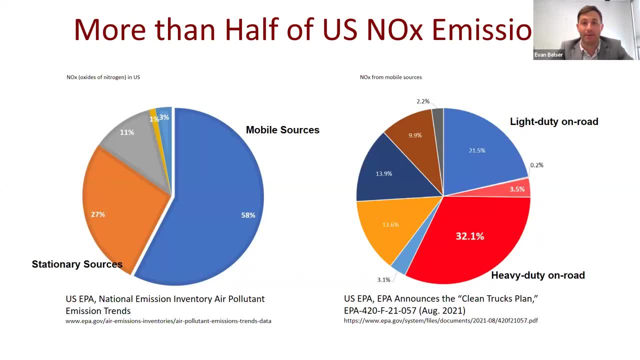 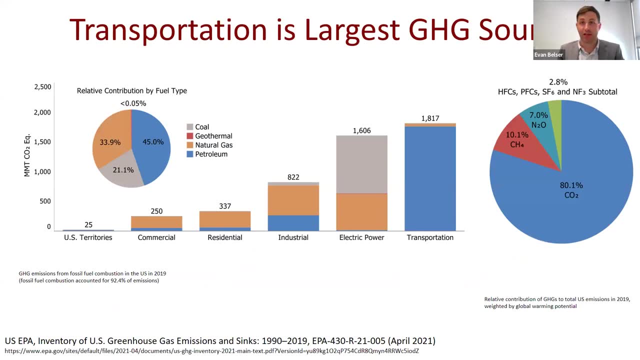 So it adds up. It matters for people's health, And so that's why it's been the subject of regulation for decades. Next slide: GHGs. likewise, transportation is the largest source of GHGs among all the different sectors. This is a on the left bar graph showing emissions from fossil fuel combustion in 2019 in the United States. 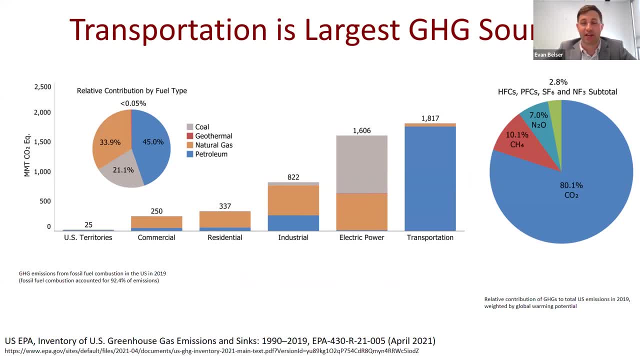 And so it's not all sources of GHG, but over 90% of our GHG emissions are from combustion of fossil fuels And there are different types of GHGs. We talk about CO2 a lot because they have about 80% of the impact of GHGs, but methane and hydrofluorocarbons, things like that, are also GHGs and are regulated just the same for mobile sources. 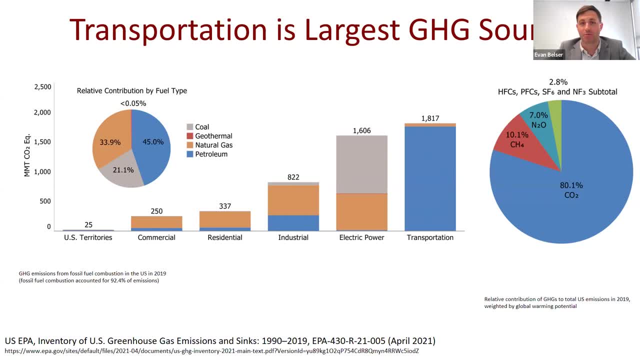 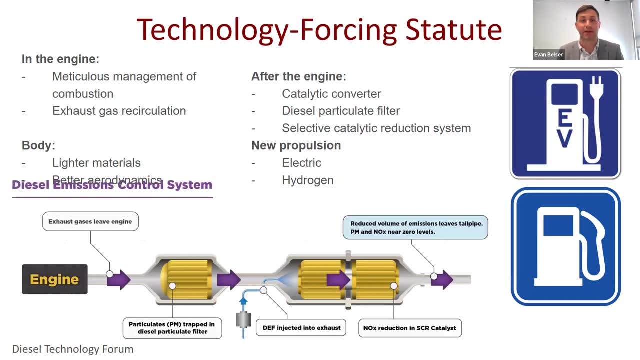 But really it's about CO2 when it comes down to actual contributions. Next slide: A very similar aspect in mobile sources to stationary sources is that it's about CO2.. Next slide: And so it's about CO2 when it comes down to actual contributions. 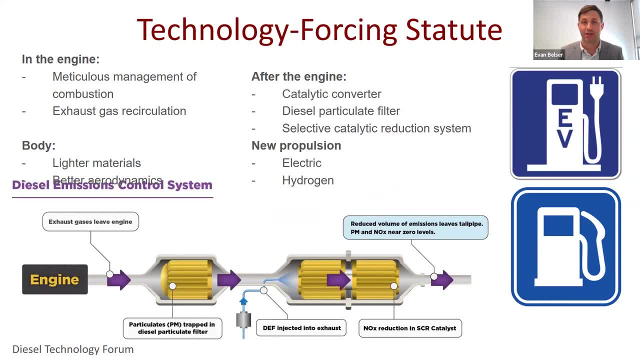 And so, as technology allows for cleaner vehicles and engines, eventually the standards then require that those technologies be used. It doesn't anywhere in the act where its regulations dictate specific types of catalysts or filters, but overwhelmingly over the years, industry has chosen to use certain types of technologies- with differences between manufacturers, of course- in order to meet the newest standards. 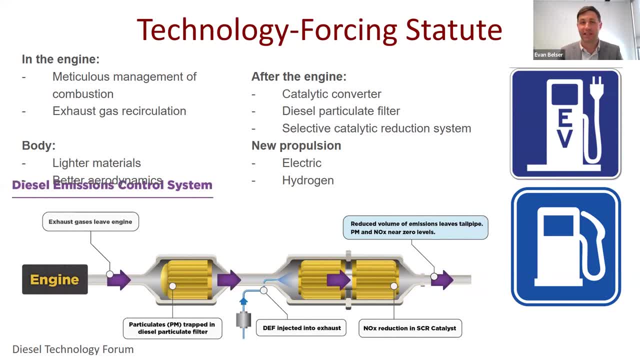 So what does that mean? In the engine itself, meticulous management of combustion has led to dramatic reductions, even without any kind of filter or catalyst after the engine. Just careful choice of parts, careful management of the actual moment of combustion can cause tremendous amounts of reduction in pollution, but also increase in power. 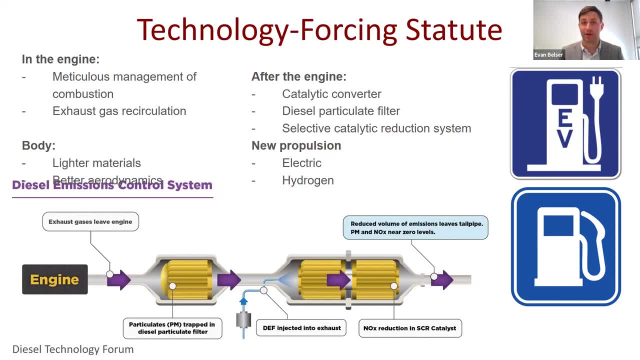 So, like a pickup truck, the emissions have dropped dramatically Over the last several decades, but power and torque have doubled over the same time period, and a lot of that is due to very careful management of the engine. And in the engine, managing combustion is all about trade-offs. 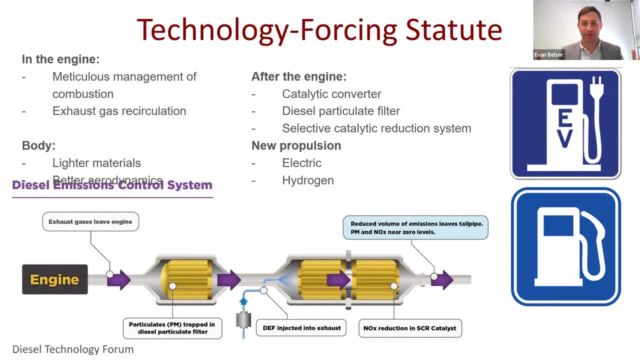 Imagine being in front of a very large, you know soundboard, essentially of dials, and you turn it one way and you compromise fuel economy but you get better NOx control and particulate matter and all these different things are important. 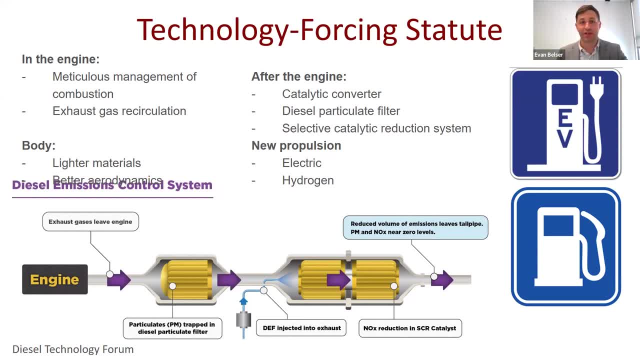 In the engine also. Next, slide In the engine also exhaust gas recirculation. this takes some portion of the exhaust and puts it back through the engine and that reduces and suppresses NOx formation. The vehicle itself is getting lighter with better aerodynamics. 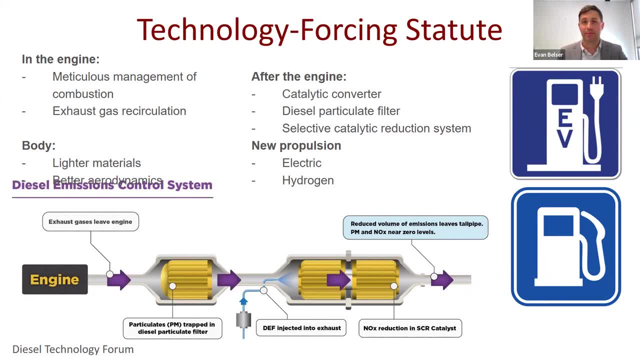 That's a highly effective way to reduce emissions- all types of emissions In. you know, when it comes to criteria emissions, what does most of the work is after the engine, in the exhaust. You've got catalytic converters, which have been standard in gasoline cars for a very long time. 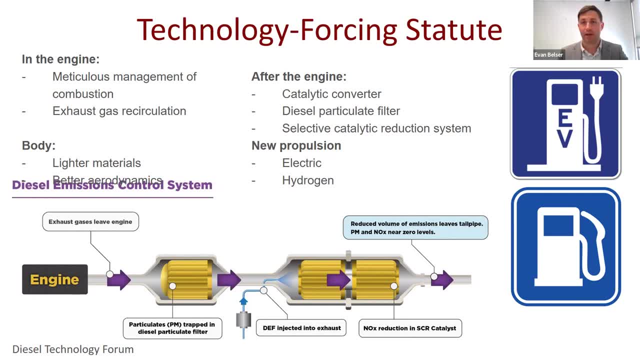 They're now the most popular at producing NOx and HC and CO In diesel engines. there's also a catalyst. nowadays it's a selective catalytic reduction system And before that there's a diesel particulate filter. So I've got a little schematic there to give you a sense of what it is that makes the tailpipe standards achievable. 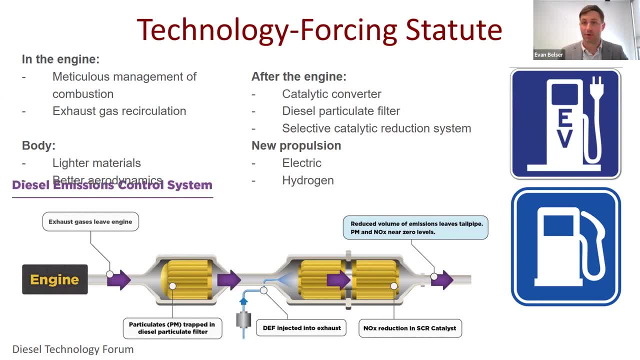 And of course you know big picture we're talking about also technology forcing means new types of technology entirely, And right now in light duty in particular. it's all about electric vehicles. It's all about electric And there are significant goals in place to move us to mostly electric vehicles and then eventually entirely electric vehicles in North America, Europe and major markets around the world. 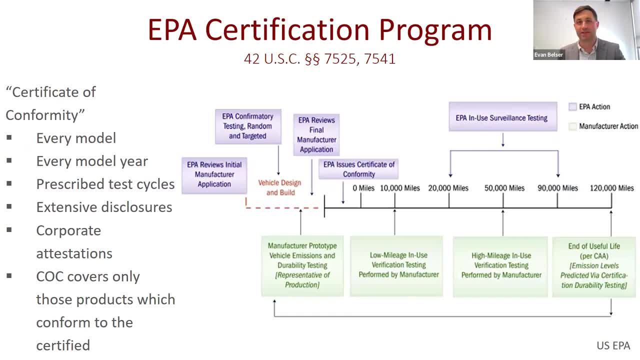 Next slide. So getting into the details a little bit. there's by the act requires that vehicles be certified, And so this is not unlike a license or a permit, And for every model of vehicle and for every model year, the manufacturer of that vehicle needs to come in with an application to the EPA and get a certificate. 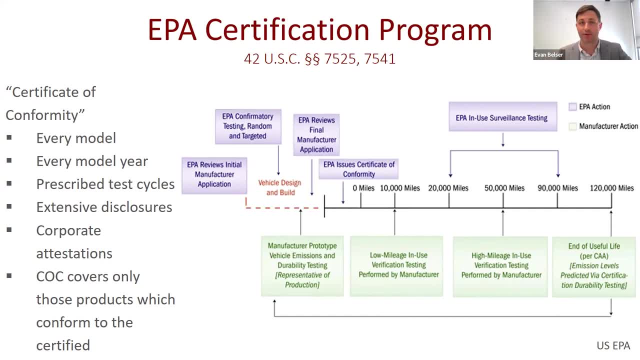 They need that certificate in their hand before they can introduce the vehicle into commerce, And so this is about new vehicle certification. They need to show that their vehicle complies and is clean with all the different emission standards. The way you do that is you test it in a lab. 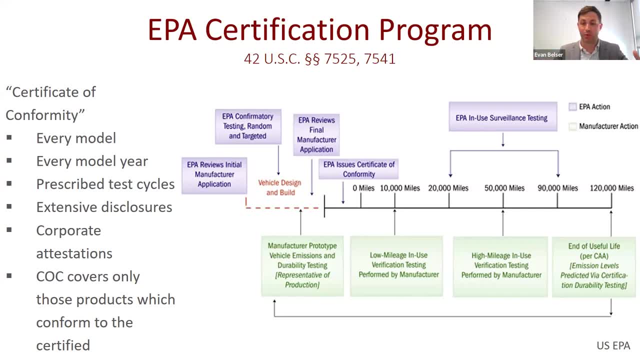 You actually drive the vehicle on equipment that allows the wheels to turn and simulates the experience of the vehicle in the real world And you catch all the emissions coming out of the tailpipe And you measure it And you see whether, over that exact prescribed test cycle cycles that are averaged together, the vehicle is below standard for all the different pollutants. 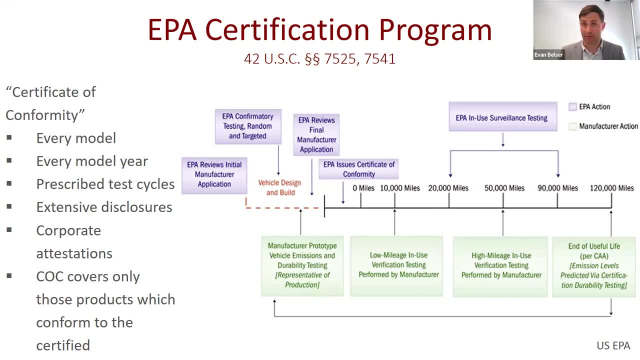 There's also requirements to put miles on the vehicle- a lot of miles- and then test it again to see whether the vehicle is durable. Its emissions control system continues to work. There's extensive disclosures in addition to the test results: Attestations from the company. 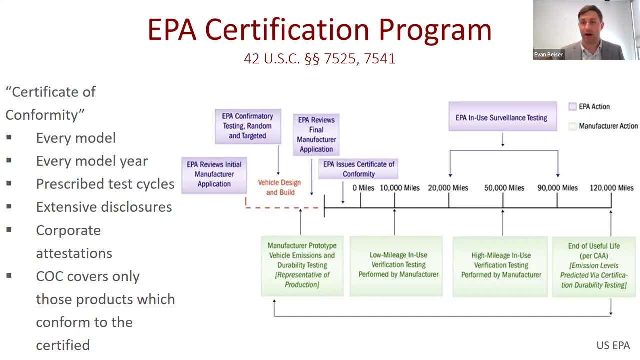 And the certificate, once issued, doesn't allow the company to do anything they want. They can only sell vehicles that conform exactly to the certified configuration. I'm not going to walk through all the details, but this timeline is very helpful to show the different steps that manufacturers and EPA do in the course of the certification program, including all the way out to the end of useful life. 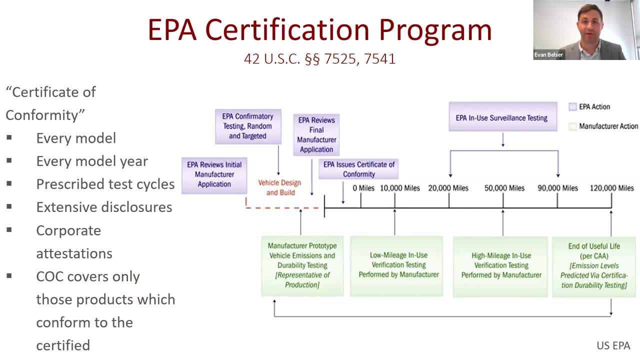 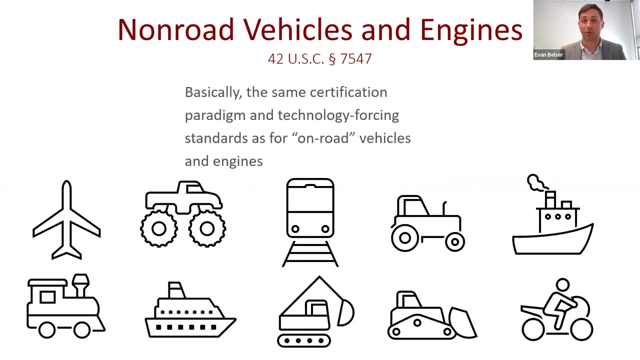 This is a light-duty scheme. It's different for heavy duty And now modern vehicles. the 150,000 miles is different. This is the regulatory useful life, where the original manufacturer of that vehicle is responsible for it. Next slide: Okay. 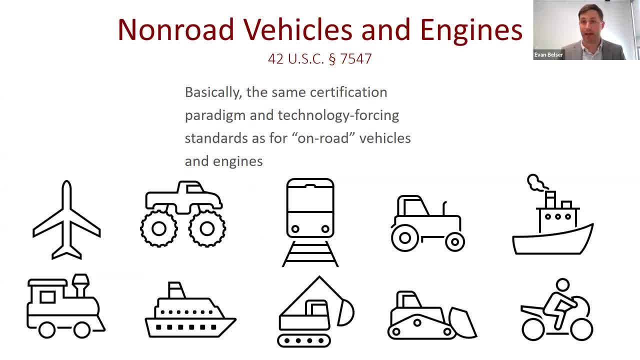 So non-road vehicles and engines are subject to the same certification program. And again in 1990, Congress said: study non-road vehicles and engines, construction equipment, lawn and garden equipment, marine locomotive, aircraft and, where there is cause to do so for the sake of human health, of the environment, set emission standards. 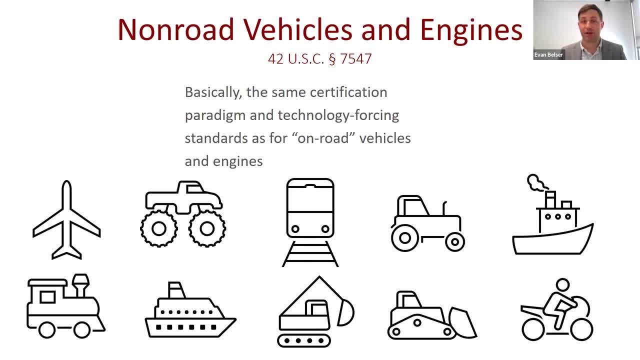 There are now certificates of conformity being issued for all these different types of things. Anything you own with an internal combustion engine in it, provided it's all modern, it's going to have a label that will tell you exactly when it was certified. It's going to have some sort of a serial number that says, if you decode it, who made it, when it was made, what the family is, what its displacement is. 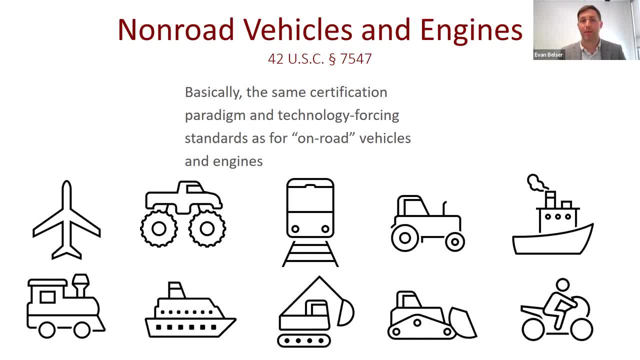 And that has been through a similar certification program as I just covered in the previous slide for light-duty vehicles. It's still a little bit simpler, The standards are a little bit different, It's less strict, But it's the same basic legal scenario. 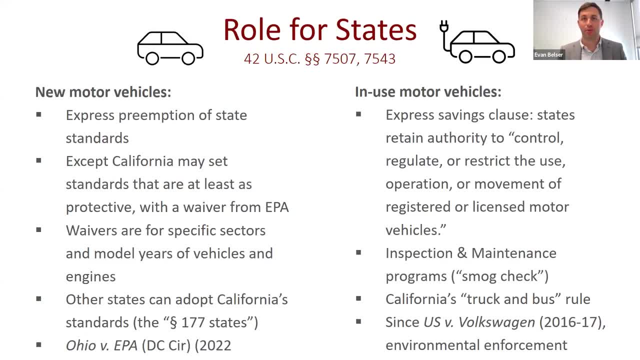 Next slide. So roles for states. So this is unlike. this is a place where it's quite different in many ways from stationary context When it comes to new vehicle standards and many aspects of everything I've talked about so far. really, it's about EPA at the federal level. 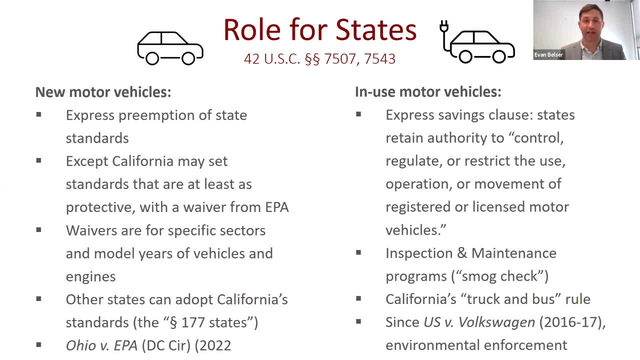 And so for new motor vehicles, this is Section 209 in particular of the Clean Air Act. It talks about the balance between federal and state. So new motor vehicles: there's an express preemption of state standards, Except big, except California. 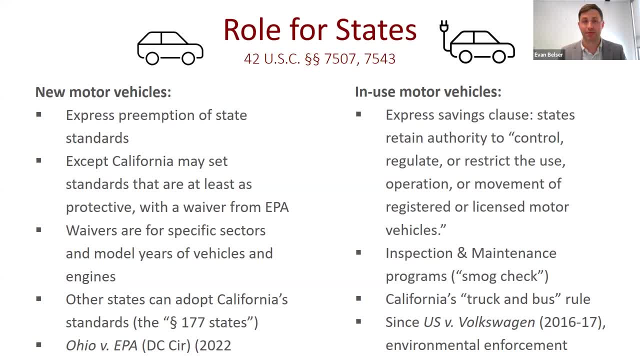 California was regulating vehicle emission standards, new vehicle emission standards, before the Clean Air Act and was essentially grandfathered in, And there was a role, there continues to be a role for California And they are allowed, with a waiver from EPA, to set standards that are at least as protective as the federal standards in place, as they are. 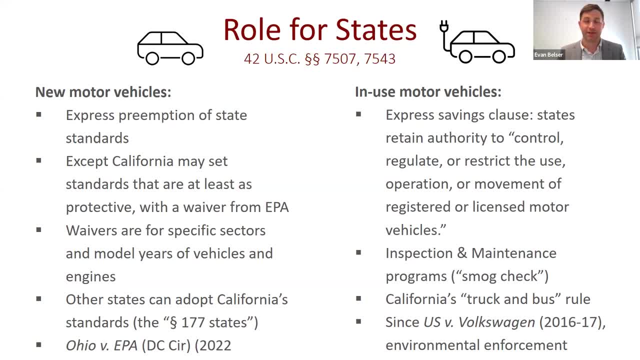 Next slide. So California has a lot of standards in place at that time. This is often talked about as like a waiver, like one big thing. It's not. It's a waiver that waivers that are for specific sectors of vehicles and engines, specific model years. 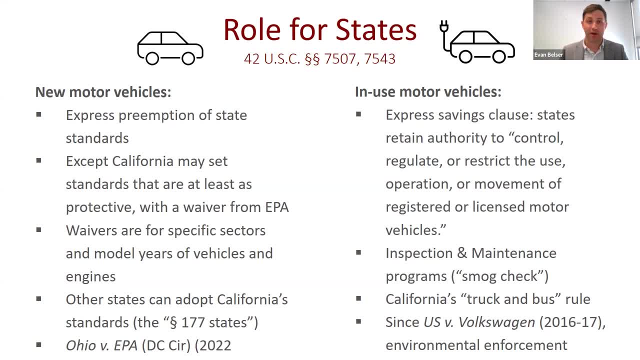 And once California has standards in place, other states can adopt California standards under Section 177.. And so it's a very interesting balance over the years about when California has essentially stepped forward and had tougher standards And then the federal standards have changed And then the federal standards often align for some amount of time. 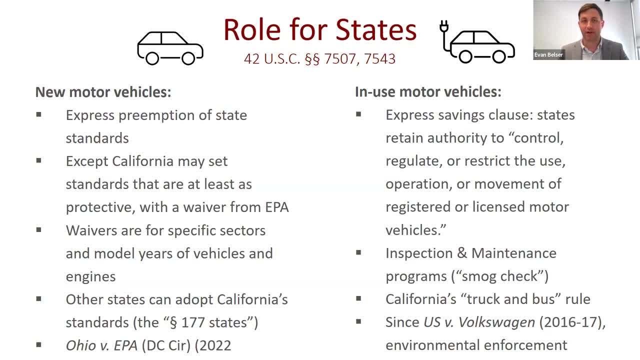 And the other states. right now for light duty, for example, I believe it's 15 states have adopted California standards And that means that about 30% of the new vehicle market needs to meet tougher standards than is otherwise required by EPA. 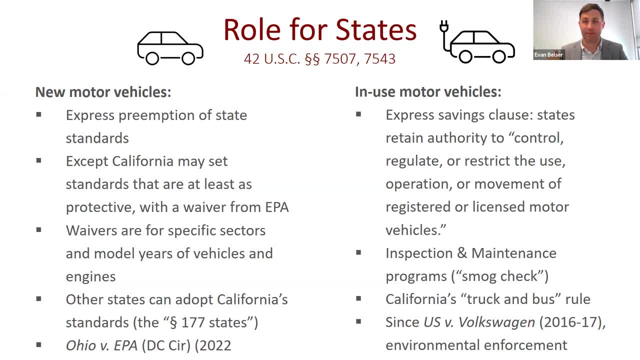 And so it's a balance over time that has seen steady march toward tougher standards. There's an interesting- I'm not getting into a lot of case law in this presentation, but there's an interesting case- Ohio versus EPA- That was just filed this year. 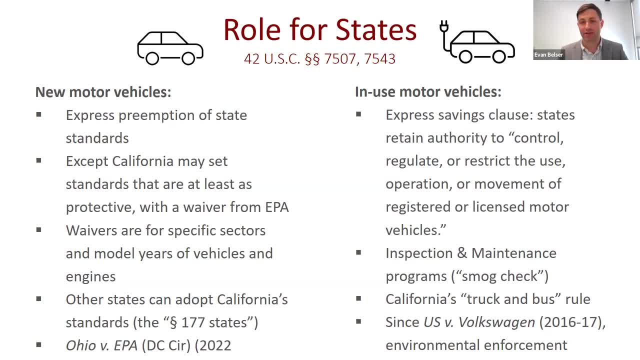 It's a direct challenge to EPA's decision to give a waiver to California to set GHG standards and zero emission vehicle targets, And so that's a very interesting state, a case that raises constitutional arguments that Ohio and others are making that California should not have this ability at all. 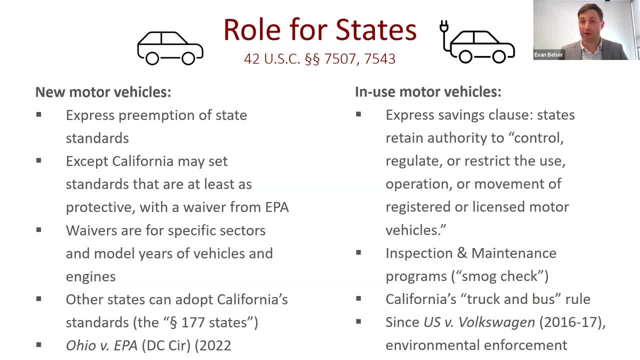 One to watch. Now, that's new motor vehicles. When it comes to in use motor vehicles, it's very different story. Right Manufacturers have to make at most two cars for federal or California, and ideally just one that meets everybody. 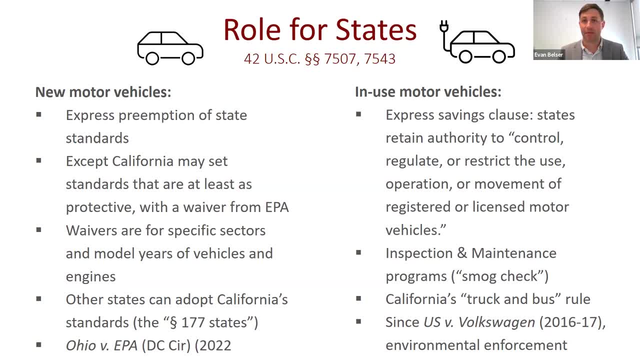 But when it comes to in use, states have a lot of express authority retained by the statute right there: Control, regulate or restrict the use, operation or movement of registered or licensed motor vehicles, And so there's many ways that states, you know, use this authority, including inspection and maintenance programs. 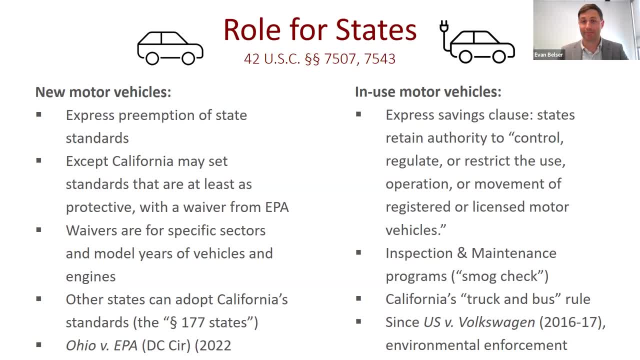 Not everywhere, Not every state, Not every county, Not every city, Not every state, And so you need to make sure that your vehicle is clean before you can even get it registered again. Highly effective to sort out gross emitting vehicles. California is a leader, has always been, in mobile source enforcement and regulation, and they have a truck and bus rule. 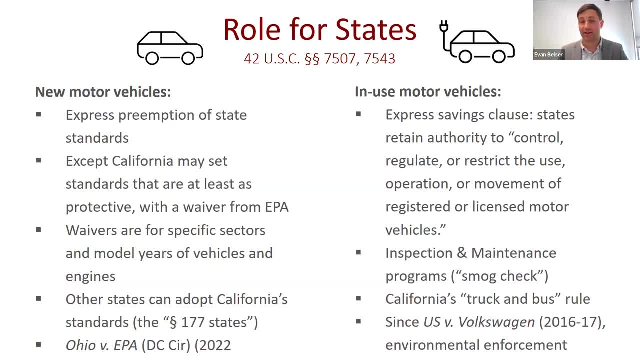 Which is it's not about a vehicle being maintained or tampered or anything. If it's old enough, according to a certain schedule, the vehicle needs to be retrofitted or replaced, And so that helps to keep prior tier, older-type vehicles off the road. 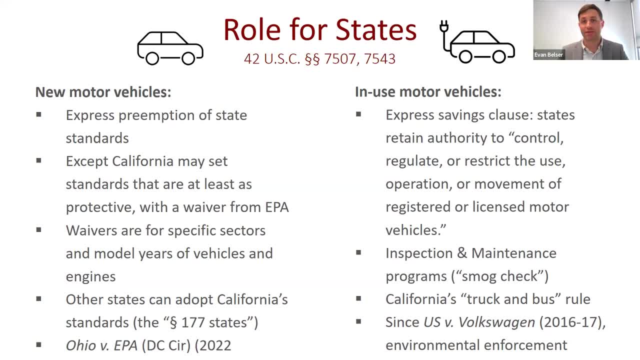 All right, vehicles off the road And as far as in-use vehicles go, since the United States versus Volkswagen case there's enforcement. States except California have generally not been involved in enforcement against manufacturers, but there has been quite a lot of that since the. 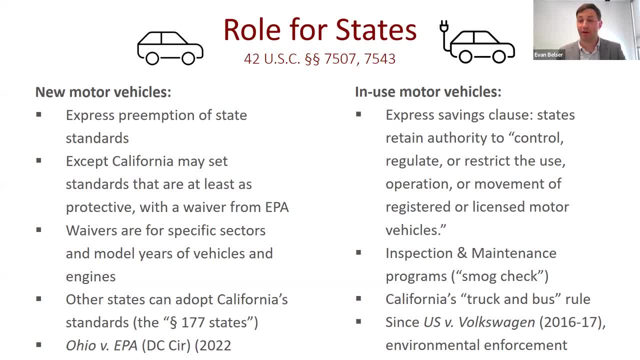 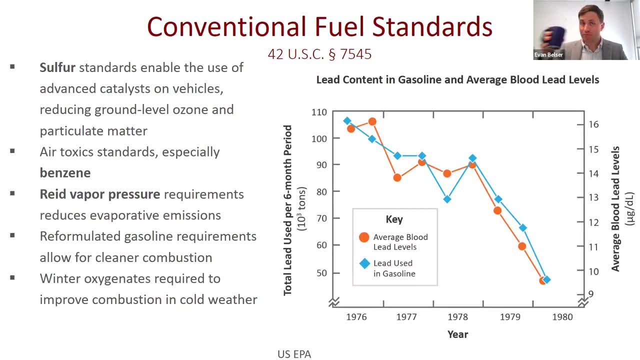 EPA's case against Volkswagen. So that's just a bit on the balance between federal and state. Next slide: Vehicles and engines are the sources themselves under Title II, and so they are rightfully the focus of this presentation. But in order to allow for the types of tight emission, 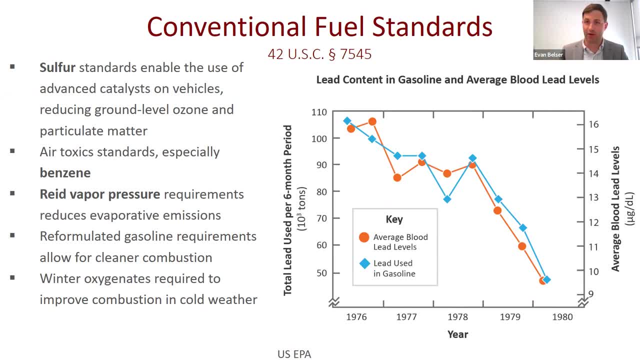 standards that vehicles need to meet. the fuel likewise needs to be regulated in order to be compatible with the emissions control systems on a lot of modern motor vehicles, And the fuel itself is controlled so that it can be controlled by the emissions control systems. So that's. 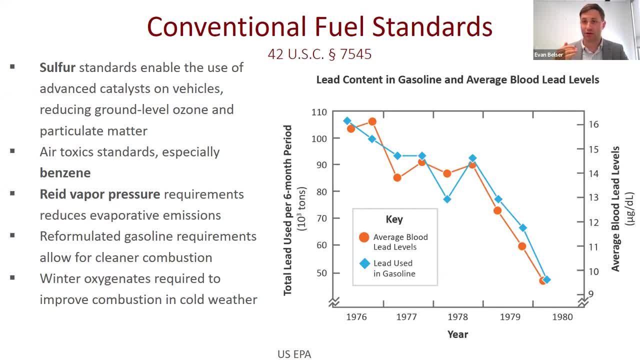 it doesn't have levels of sulfur and benzene that actually could pass right through emissions controls and be a source of harmful air for people, And so this is a list of the different conventional fuel standards for sulfur, air toxics, especially benzene, read vapor pressure. 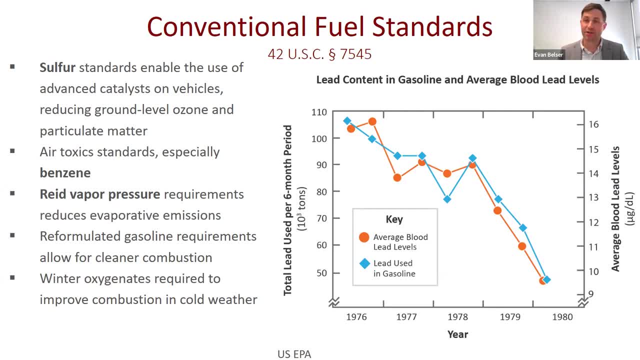 requirements, RVP requirements that reduce evaporative emissions. That is seasonal, So that changes based on what time of year it is And reforming of the gasoline requirements and oxygenates are other things that are important. There are a number of things that help improve combustion and just make for cleaner combustion. 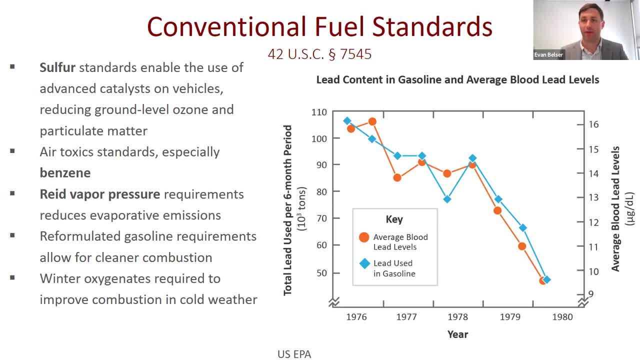 And I won't get into it. but can't talk about fuels without talking about major environmental victory. that was not that long ago. We had lead in gasoline and EPA got lead out of gasoline, And this is a fascinating, I think, powerful line graph here, which is data about the amount of 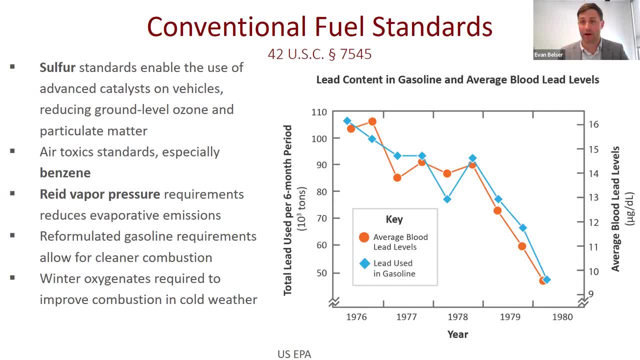 lead using gasoline and the amount of blood lead in people's blood in America, And you see they just fell right together and so it's a very important lead obviously is bad news for people's health and it shows the the importance of fuel quality and the importance of regulation in in cases. 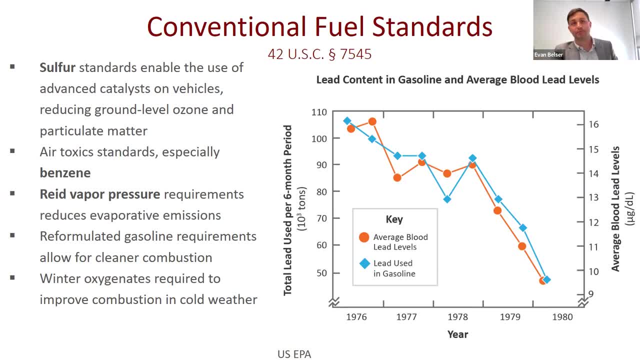 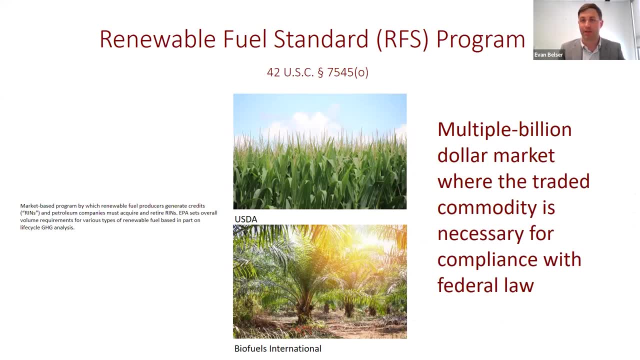 where people's health is at risk. next slide: um. so there's also another major element of title ii. that is not about people's health directly. it is about reducing our dependence on imported oil, it's about reducing climate emissions and it's about growing renewable fuel sector in the united. 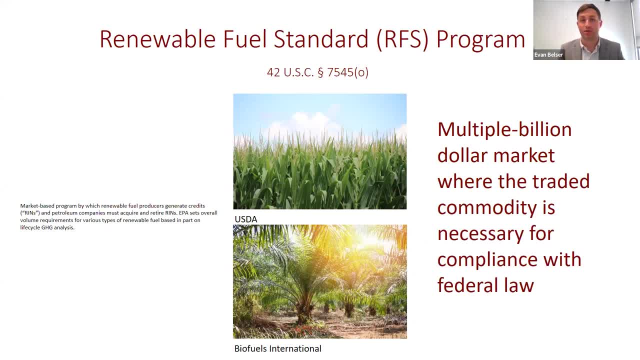 states. those are the three expressed written goals of congress when they wrote the rfs program in 2005 and then updated in 2007.. and this is a market-based program where renewable fuel producers are able to generate credits, provided their fuel meets certain requirements. and then petroleum. 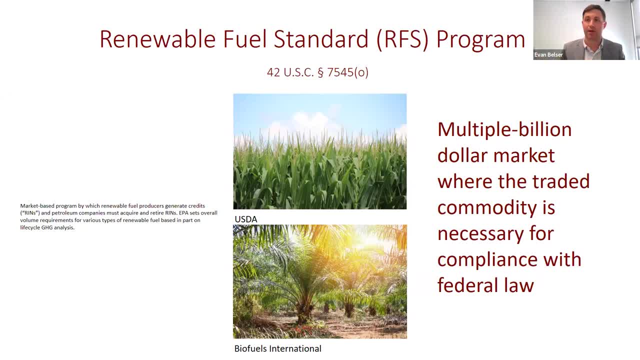 companies need to obtain those credits and retire them in proportion to the amount of petroleum they deal in. and that's one of the things that i think is really important, and that's one of the things that i think is really important, and that's one of the things that i think is really important. 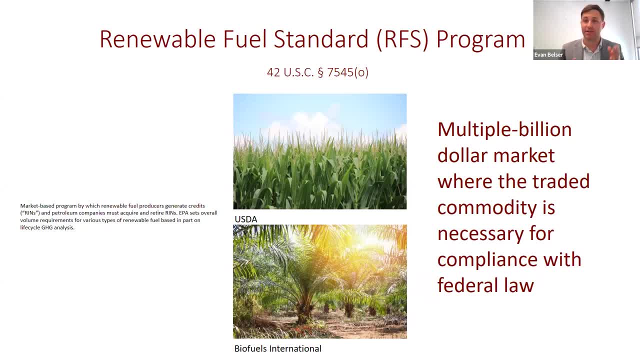 that creates a market. it's a multi-billion dollar market. the commodity is a credit that comes from renewable fuel companies and that drives uh and affects the market for liquid fuel, and so this is just about transportation. but it is one of the earliest ghg programs on the books and it's a 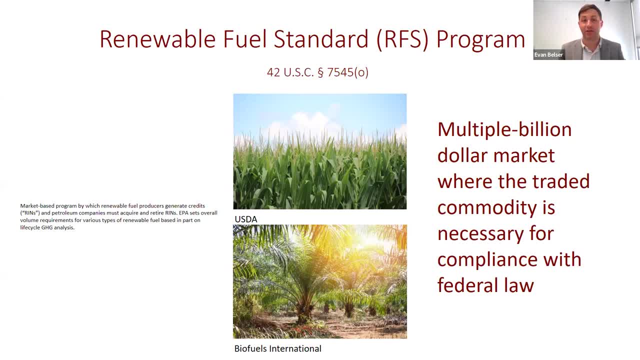 very complex and contentious area that is likely to grow a widespread. you know rumor that the epa will propose standards soon to expand the rfp program including to include electric vehicles, where the electricity used for those vehicles is from, for example, a landfill that is capturing methane and producing electricity from that methane. 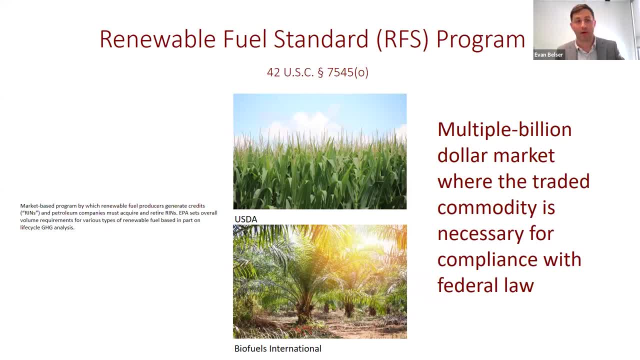 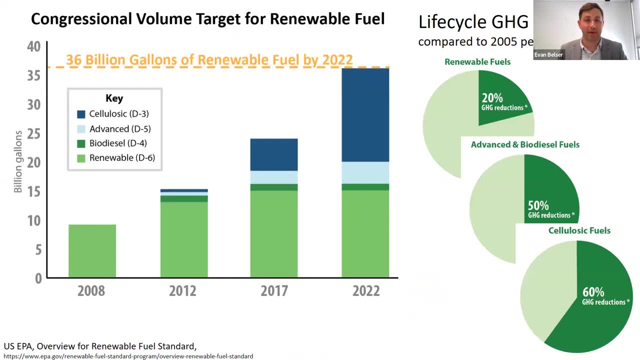 so it's a complex area that ultimately, is about reducing carbon from transportation. next slide- this is the last, i think my last slide- and it's about the goals of the rfs program to increase the the amount of renewable fuel or hydrogen that's being produced in the rfs program. 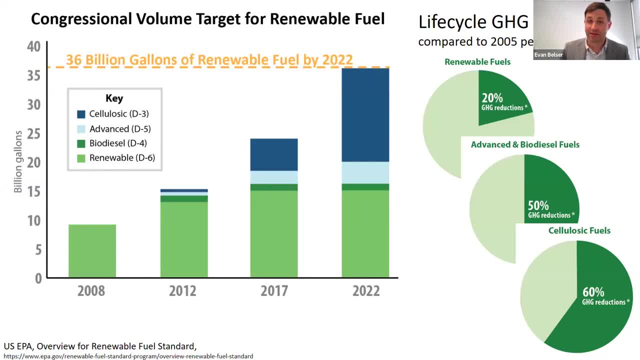 over time, and so there's different types of life cycle analyses done and different and based on those life cycle analyses for renewable fuels or advanced biofuels or cellulosic fuels. there's different sort of credit available within the program, and so this is definitely an interesting 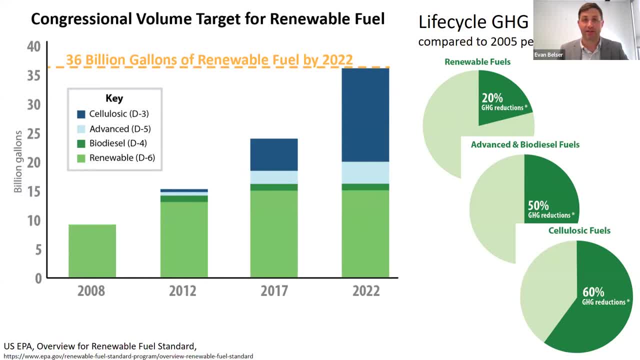 area that is likely to grow with uh with time and is likely to see a lot of attention, especially next year. and so that is, in a nutshell, title ii of the clean air act and how it is that, at federal level at least, we regulate mobile sources in the rfs program, and that's what we're looking at right now. 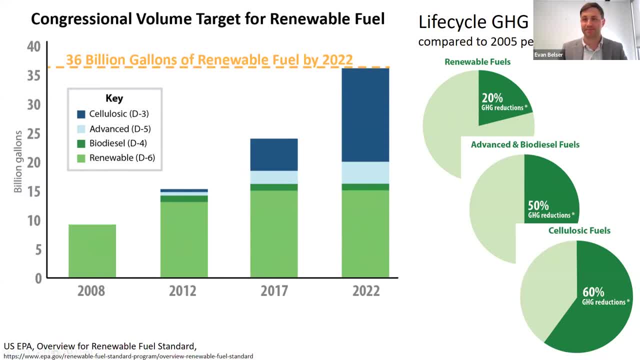 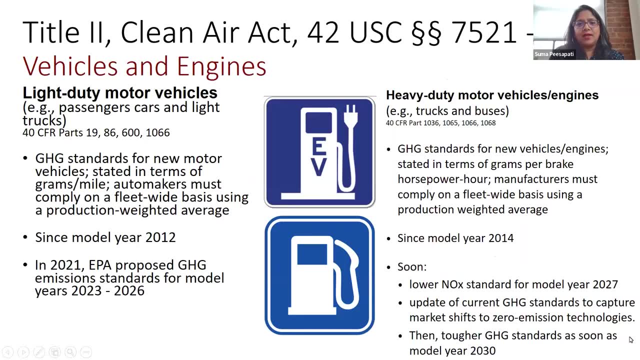 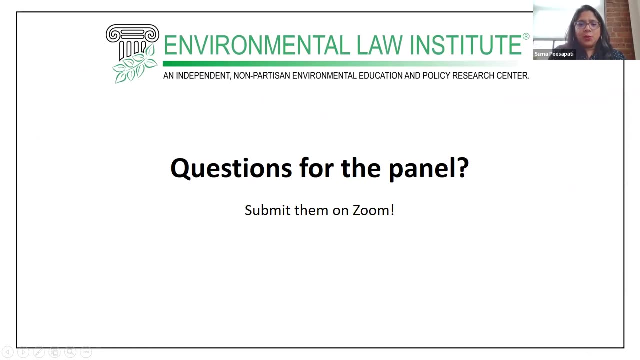 with the rfs program, and that's what we're looking at right now: air pollution, thanks. thank you, evan. that was a wonderful presentation. i learned a ton um obviously a rapidly evolving area of law um, and a very interesting one um. so i think at this point um it. 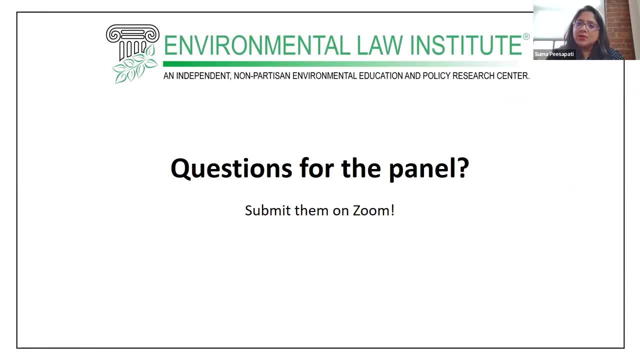 would be good to move to the question and answer uh, just the the round table, rather um among us. um, you know, obviously the big news today, um, as of just a few hours ago, is, um, the supreme court's decision in west virginia versus epa. um, you know, just to be uh transparent with the audience, it is so new we haven't had a. 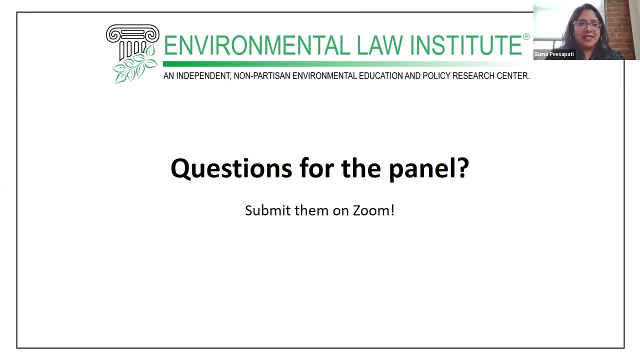 chance to read the decision. that being said, we were expecting it, um, this week, um, hopefully a little earlier than today, but it is what it is, and so, um i i wanted to at least uh pro acknowledge the decision and uh gather angela and evan's thoughts. 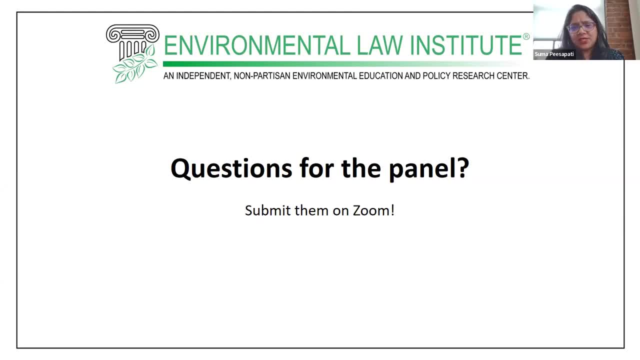 um on the in its uh, on its implications, um. so let me start with a very brief kind of background: um on what the dispute was about. um. so this case um, involves the, the trump administration's affordable clean energy rule. it's not a clean energy rule. it's not a clean energy rule. it's not a clean energy rule. 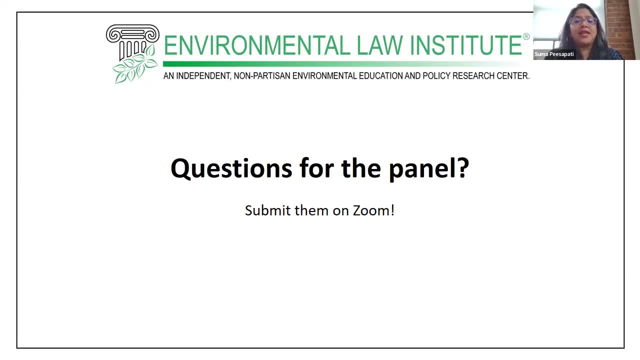 it's one more and it's part of the eu, as像跟 um. so, coming back to the, the ace rule, the dc circuit rejected uh, this weaker rule, but it's important to understand that the biden administration has signaled that it wants to take an entirely new approach, um to regulating greenhouse gases from the power plant sector. 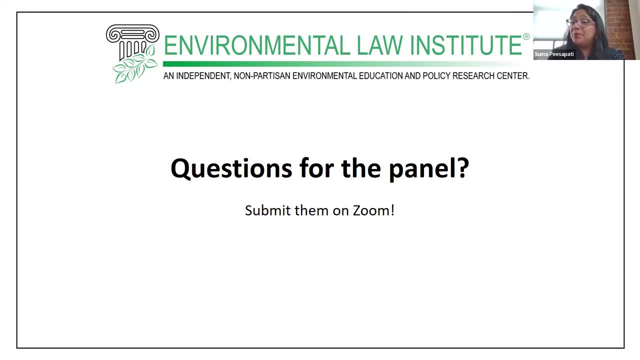 um and, you know, effectively taking both the clean power plan and the ace rule out of play. nonetheless, the supreme court still decided to review the dc circuit's ruling on the ace rule, um and took the opportunity- the high court took the opportunity- to rule, to opine on whether um 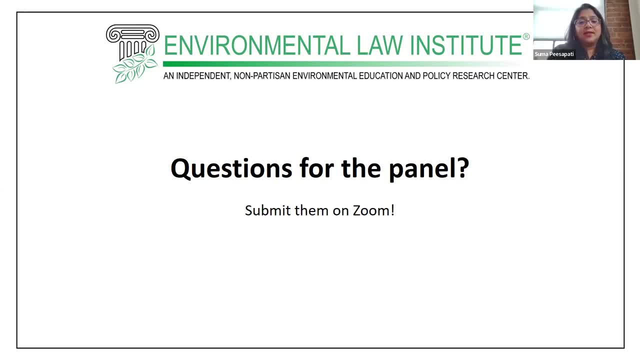 epa has the authority under the clean air act regulate ghg's from industrial operations, so, um. so i would like to ask our panelists, you know, what was the, what was the, what were the major takeaways, what was the outcome of the case? um, and maybe, evan, if you wouldn't mind starting, sure it's. uh, yeah, it's funny timing, um. 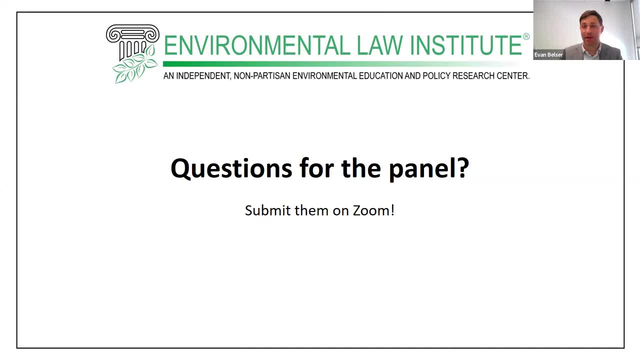 so yes, it's 89 page opinion six, three to six um and the i i saw three basic holdings: one they held. yeah, you know, this is justiciable. this is still something the court can review, despite the court's history of not issuing advisory opinions. to me it looks like an advisory opinion. it looks like an advisory opinion to the dissent as well. 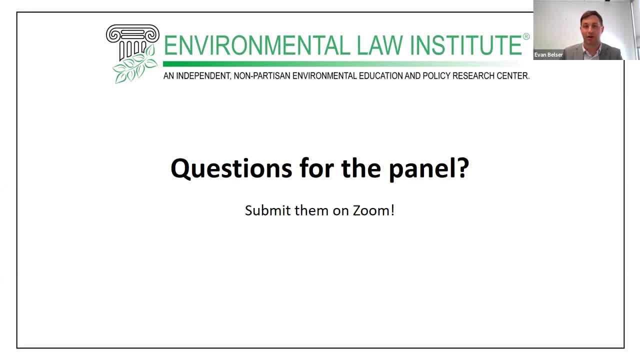 um, the main opinion is that the court is not issuing advisory opinions to the dissent as well. the merits are: there's two holdings there. one is looking at the clean air act and it and 111b in particular, and the court held that 111b does not give epa the authority. 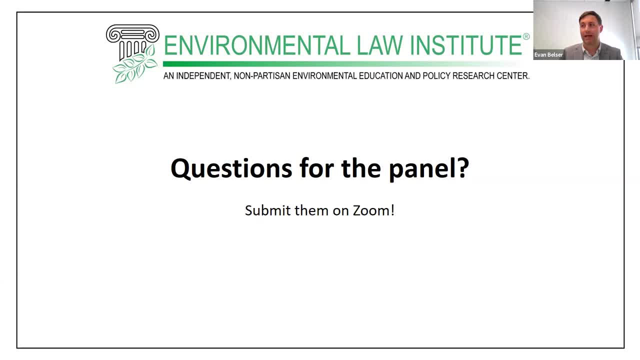 to regulate the power sector the way that it did in the clean power plant. it does not give epa the authority the court said to require that regulated entities to regulate the power sector, because it does. it appears in fact in the ihnp parl rinse, or whatever the company a bill is. 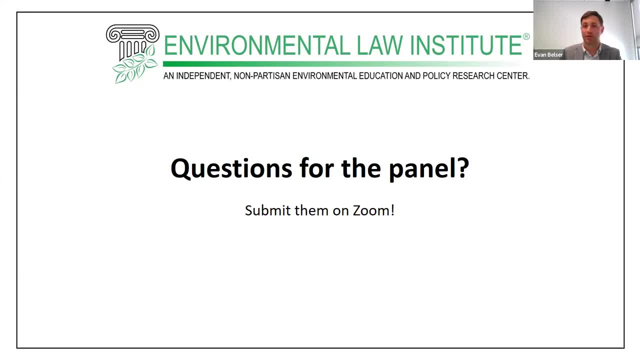 gauge. it obviously dates back to garage sale claim that was possibly listed in the news that was it flyer. i don't even realize that it's there, but it looks like it was and i do think that this is based on the point brent was making for this. 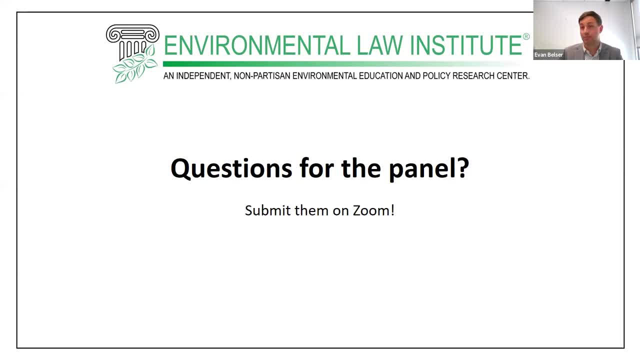 that the court is making a rule that it probably has the authority to regulate this- the court. i'm interested in the review because i agree that this is under the 01 and so there's an issue there if it's smell. anyway, if the court is initiallyகவ Richard. 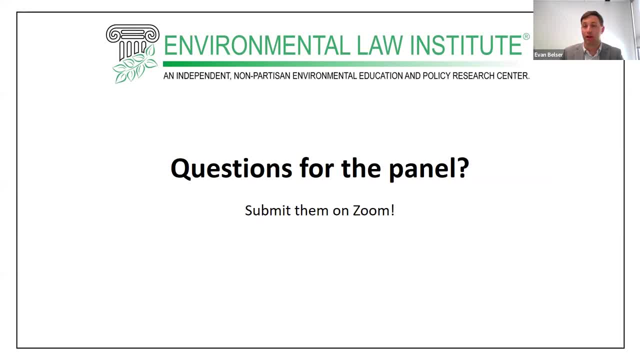 knows that. it's not that this is under the linux of service or something. patience is needed, no matter, and we're we're talking to carpentry is there's three days and they haven't been admitted. does it mean system more broadly, Like the grid is a system and the grid has many sources of? 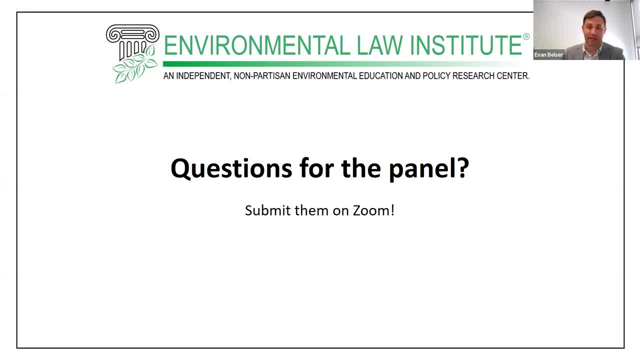 electricity that get onto it. And the last piece that I saw was that the court made a pronouncement that this is a major question- whether to regulate GHGs from the power sector, And under the major questions doctrine they're calling it, this is something the agency can't do, unless and until. 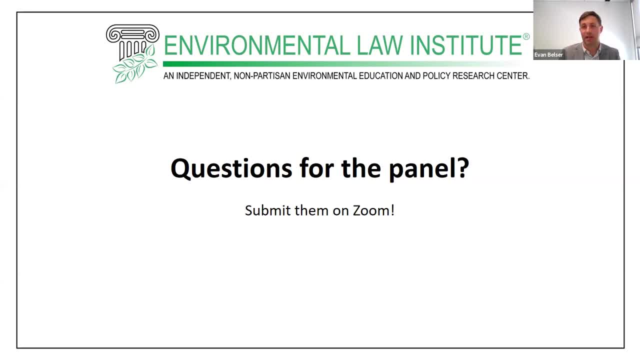 Congress explicitly speaks to it and gives EPA that authority. And I saw that the 111D interpretation and the major questions doctrine is smeared together. I don't really know whether they're the same or if they're somehow independently. you know, until I get into the 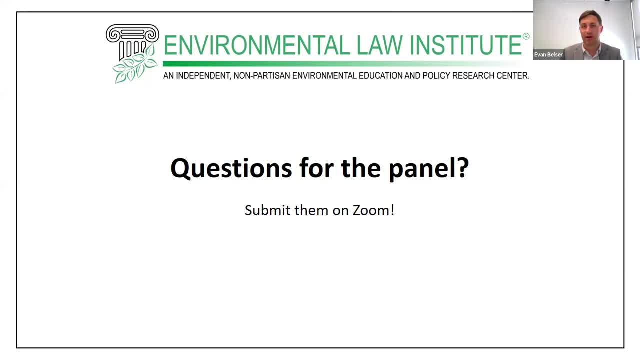 opinion independently adequate to reach the decision the court did, But by all accounts it appears to be a total loss for the EPA. Thanks, Evan. Angela, do you have anything to add to that? Yes, I haven't read the opinion. 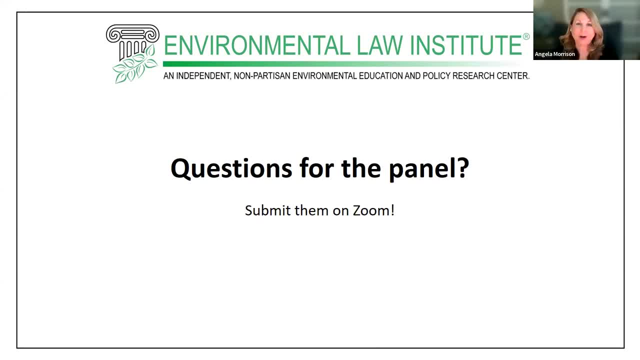 but I did listen to the Supreme Court oral argument And I would highly recommend that if you want to nerd out and listen to the Supreme Court justices talk about inside and outside the fence line. So, if you recall, I was talking about the 111 definition of a stationary source, which 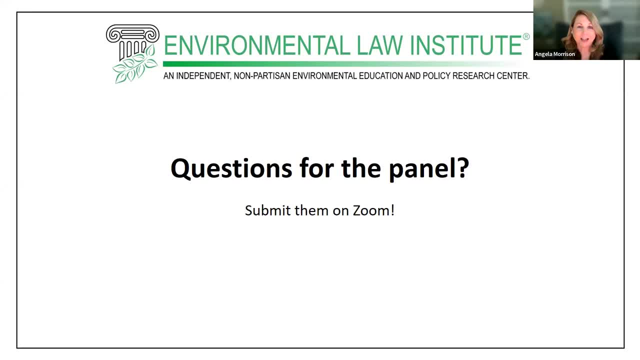 is the basically the unit. It's not the entire contiguous property under common control. It's the unit And so that's generally how, under NSPS 111, standards have been developed And there was no challenge to the NSPS 111 standard for new power plants. that that's on the books remains. 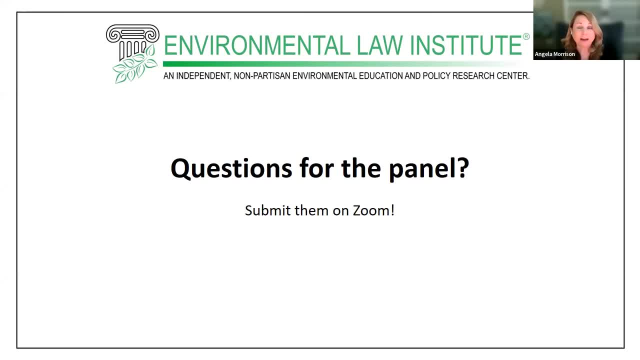 unchanged, Basically all the combined cycle natural gas plants can meet the standard. they'll even be lower than the NSPS under a BACT determination for greenhouse gases. So it was only the 111.. D program for existing power plants that was subject to this appeal. And what Congress when? 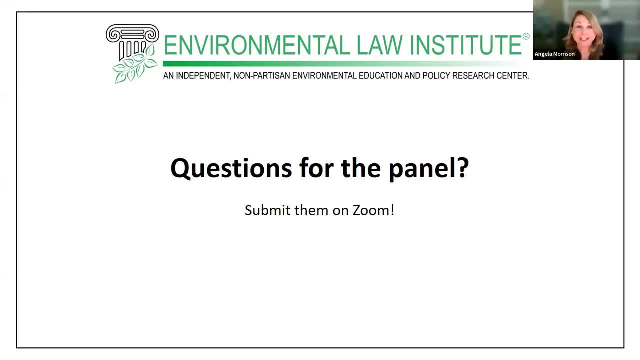 Congress did the 90 amendments. they didn't really change the 1970 111 program for new source performance standards. So that's been on the books for 50 years. you know NSPS has been around. In the 90 amendments Congress established the acid rain trading program. 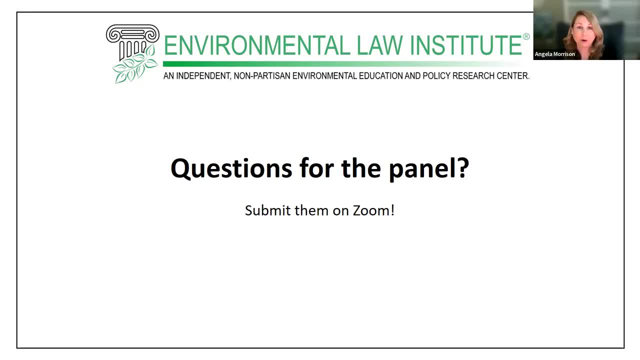 where so two emissions were traded- highly successful program And and power plants were, you know, resistant at first, got on board highly successful, And so that's what they were looking at. here is a source of emissions trading outside the fence line under a 111 D program, where it's 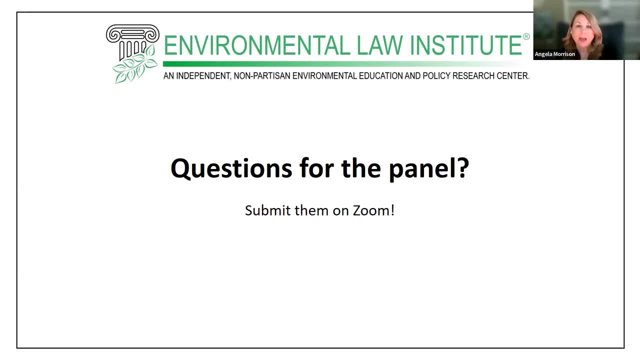 really implemented by the states. the guidelines are set up by EPA, and then the states would have their own program how to figure out how to meet certain greenhouse gas caps with within their state And maybe allowing emission trading even outside of the state, And so it might have been a little bit. 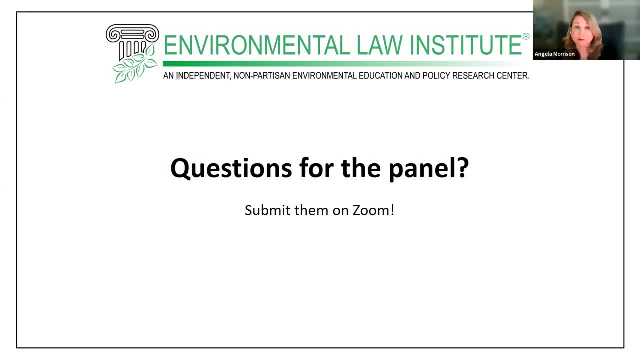 of a square peg round hole issue here of trying to use this 50 year old rule, that or the statute and the implementing rules that talked about best system of emission reduction, which those of us in the industry and have been, you know, looking at how the Clean Air Act has been implemented over 50. 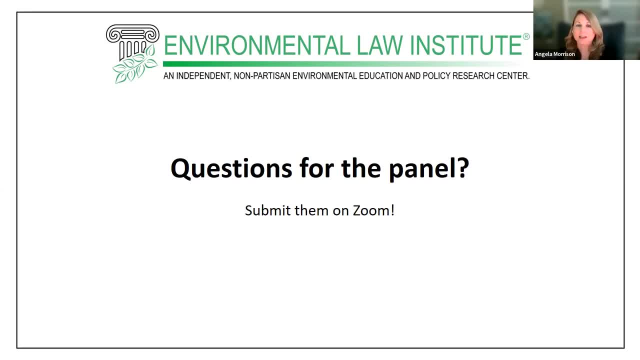 years. it's really talking about a pollution control device. it's not talking about emissions trading. So, even though it's a good idea, industry was on board it. you know, it was maybe a stretch to use the one 11 D program to do it. 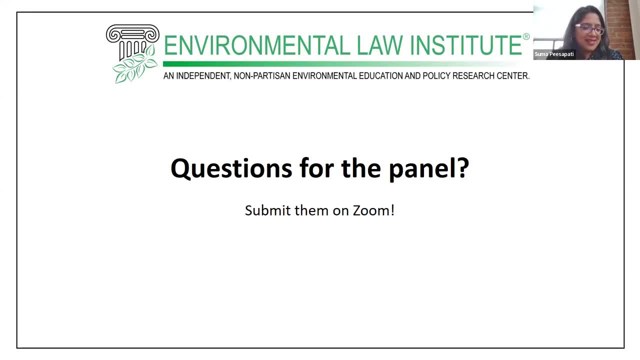 Interesting. Yeah, I mean, I think it's, it's a decision that represents, I think, some new direction in the jurisprudence And you know, as ever mentioned on the case and controversy front, traditional notions, you know what types of cases that the court will take up. also, on this question of the powers of 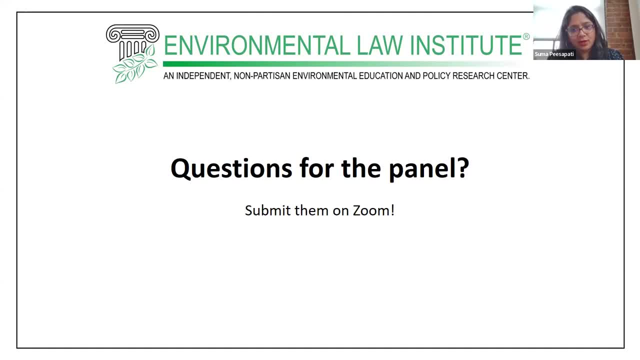 administrative agencies, um, and you know, how does this affect, i think a lot remains to be seen right on um the administrative state and um, you know the- i think it's fair to say- expansion of this doctrine, of this major questions doctrine, um, you know, you know at some level, what is it? uh, what you? 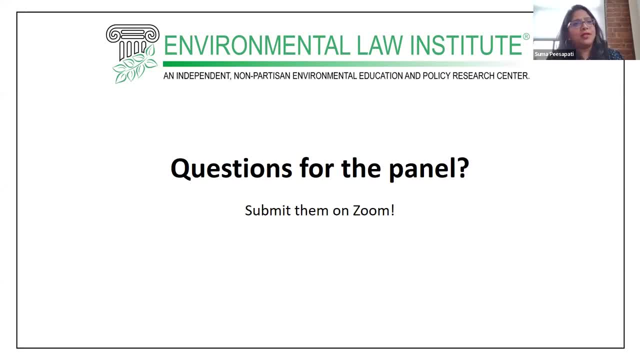 know, kind of big sweeping um regulatory uh initiative isn't doesn't raise a major question, and so i think that remains how this, how this grows, how this evolves, um this decision, um, or how it does or does not, i guess remains to be seen um, but it's, it's a big one, this is a huge decision. 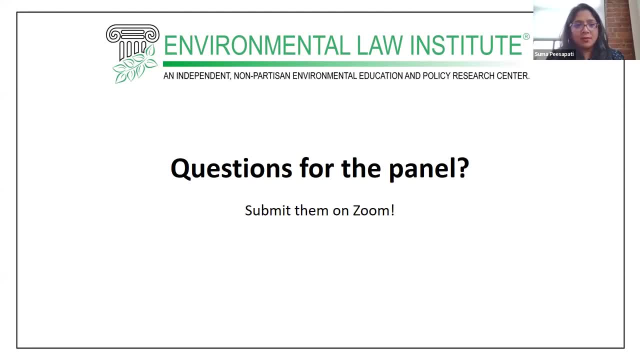 out of the out of the court and, um, i think we're all just beginning to learn its implications. we, you know this is to regulate existing coal-fired power plants and they're- they're aren't new coal power plants being built. coal plants continue to be taken out of service. 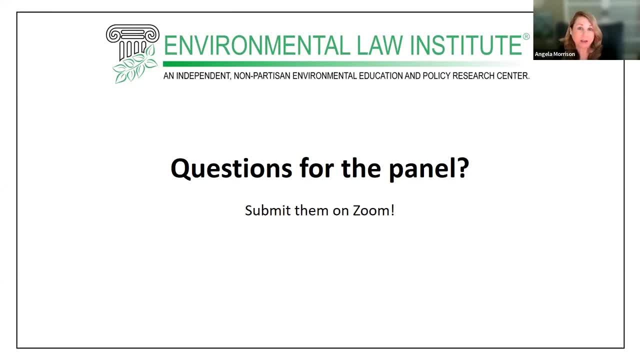 we've seen greenhouse gas emissions go down even without this trading program in place and neither the clean power plan nor the ace rule coming into effect. and epa does have authority to regulate methane emissions and cfcs and hcfcs, which are big in addition to CO2, to greenhouse gas. 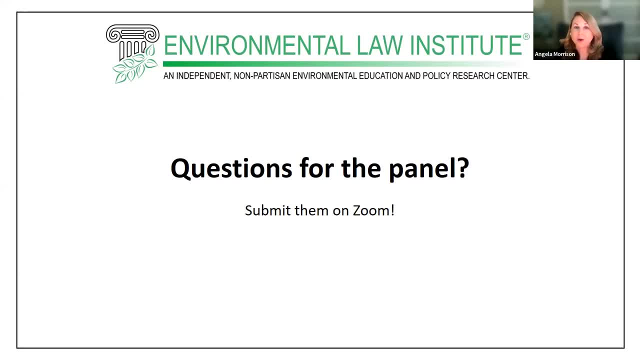 they have a higher greenhouse gas warming potential. So I would say, you know, for anyone worried like, oh no, EPA won't be able to do anything about greenhouse gases, that's not the case, Thank you. Yeah, I'm seeing a couple of good questions in the chat. 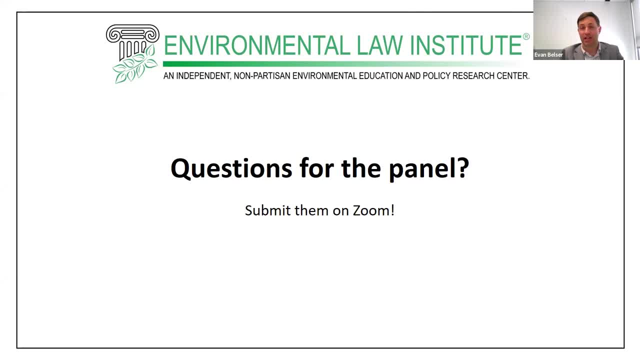 but before we move off of the West Virginia case, I can say that I don't see any impact on electrification of cars and trucks and just mobile sources generally. to further Angela's point, The case doesn't cite Massachusetts. It doesn't discuss the endangerment finding. 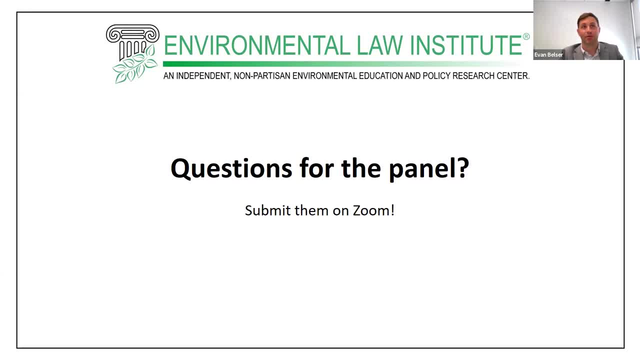 It's not about that, And so you know. the other question raised is about major questions, doctrine I: it doesn't. I have again I need to spend more time with the case to be sure, but it doesn't appear to be about affecting. 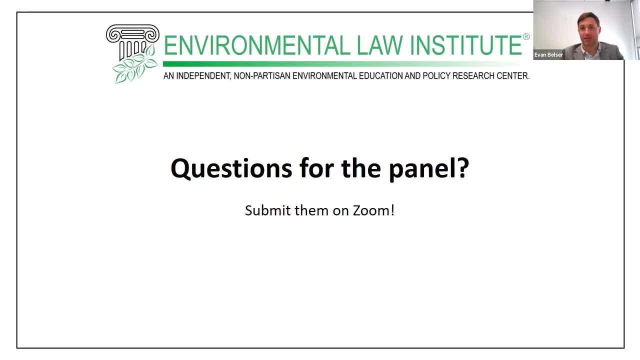 the jurisprudence around deference to agencies. It's something different than that. I don't think the majority even cites Chevron, So I'm not entirely sure, And that leaves me a little anxious about what does constitute a major question, because I'm not sure what it is that people go. 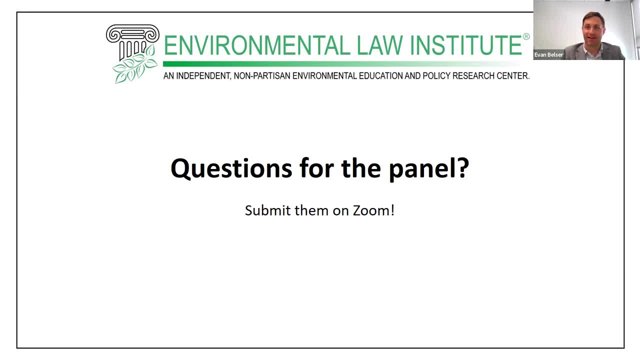 to federal court about. that, to them, isn't major right And it couldn't fairly be characterized as a major question, So it does, I think, create fodder for challenges to any federal action going forward, And it's not clear to me just what the threshold is. 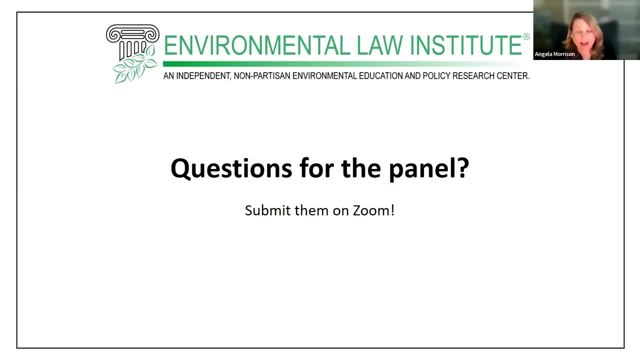 Or maybe any federal action that's not clearly outlined in a statute. Well, I appreciate the ending on a hopeful note on that topic, But, switching gears a little bit, I was hoping to turn to the topic of enforcement under the Clean Air Act. 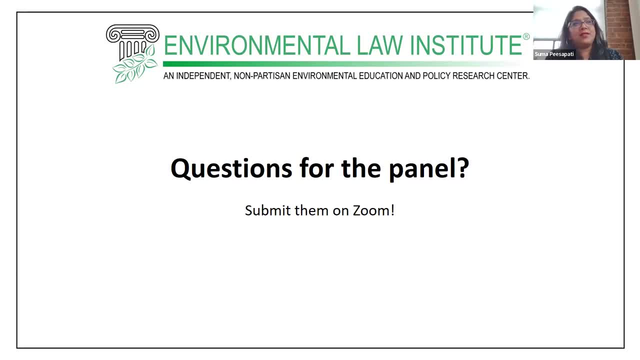 So I was hoping that you both might be able to illuminate the audience a little bit about what enforcement tools exist under the Clean Air Act, yeah, and how they're used, And maybe this time we can start with Angela Sure. What's impacted my clients the most is starting. 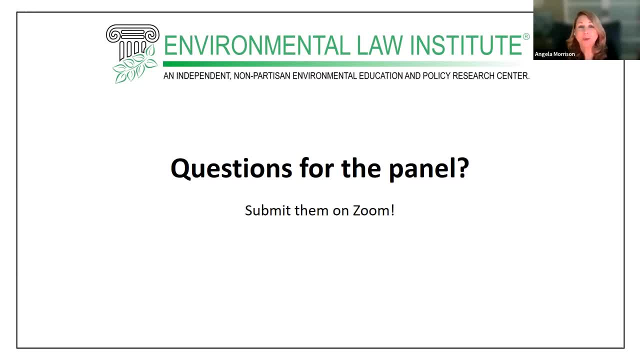 with informal discovery under section 114 of the Clean Air Act, where EPA can just come in and request a ton, boxes, boxes, literally tons of documents to take a look And and take a look at, you know, on their own at. 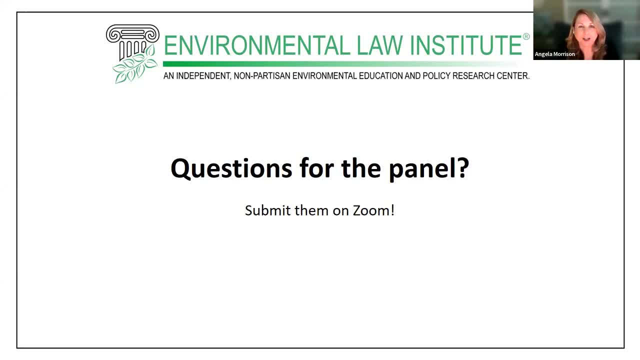 without you know, waiting for formal discovery and litigation or anything like that. There are also a lot of self-reporting requirements there under Title V- their annual and semiannual compliance certification. So you're kind of handing the agency what they need to enforce sometimes. 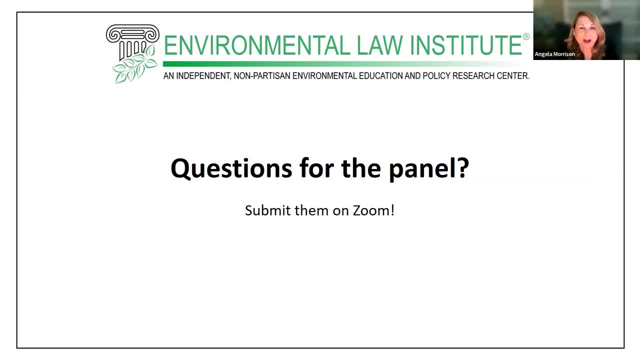 And there are also quarterly and semiannual monitoring reports. If you have air emission monitors on your stack or you're required to take, you know, temperature readings or whatever you're supposed to submit those. So you're giving the agency a lot. 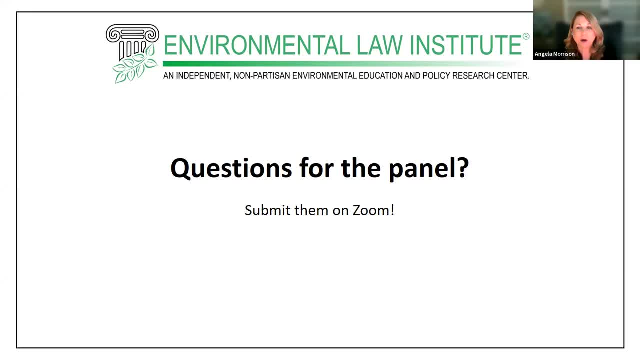 So I think that usually there's not a lot of mystery in what's been going on at a plant when it comes to enforcement, And the state and local programs usually have the lead in enforcement, And so as long as a facility has a good relationship, 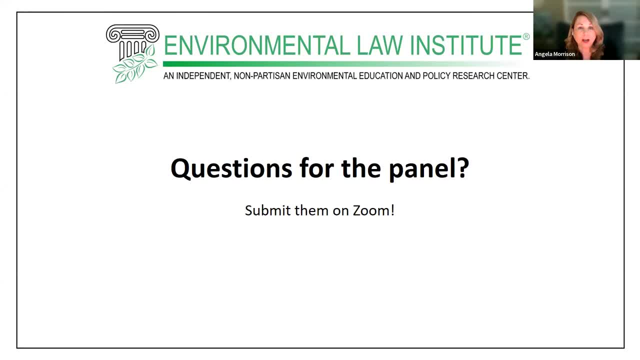 with their, the enforcement personnel. you know, keep those lines of communication open. hopefully you won't wind up. you know very rarely with criminal, unless it's most of the criminal I've seen, and Evan can get into this. 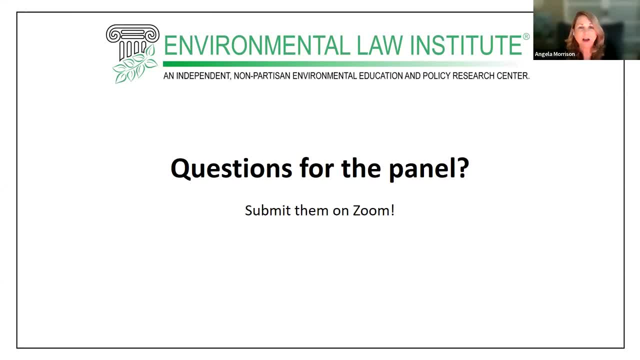 other than the defeat devices is in asbestos or something like that. But for the industrial facilities they try to stay in compliance and that's why they will utilize attorneys like myself to make sure they stay in compliance. The biggest enforcement cases came under: 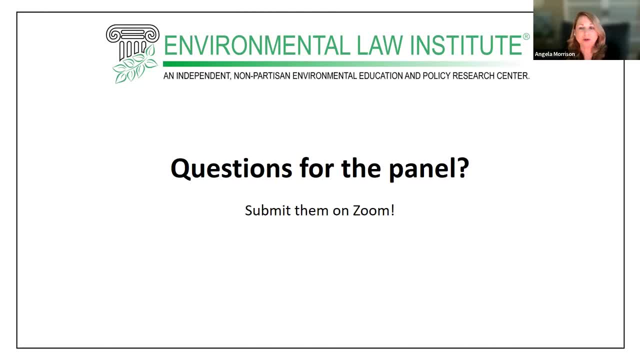 when Carol Browner was the administrator for EPA under the Clinton administration where they were looking at. you know when Carol Browner was the administrator for EPA under the Clinton administration where they were looking at. you know when Carol Browner was the administrator for EPA under the Clinton administration where they were looking at. 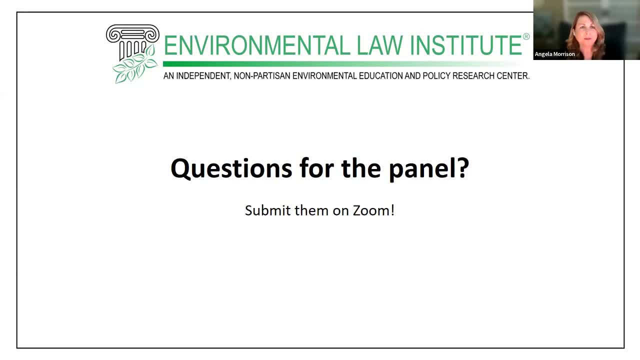 the history of modifications? and what should some facilities that have been operating for 30,, 40,, maybe 50 years and we're still grandfathered? And why haven't they undergone new source review and upgraded and applied the best available control technology? 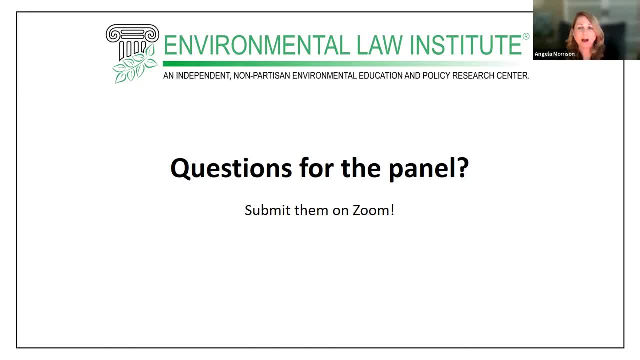 put on new source performance standard compliant equipment And that some of those cases have just you know, from that administration which started maybe in 2000 or so, you know all the way until we, you know, we just recently resolved some of these cases. 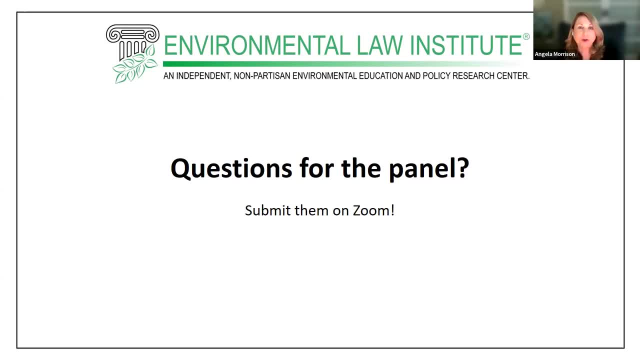 maybe within the last two or three years, So this is a new source review. Enforcement initiative was a big thing for a long time It was not a priority- I don't think for Trump and I don't think it's been a big, important issue for the. 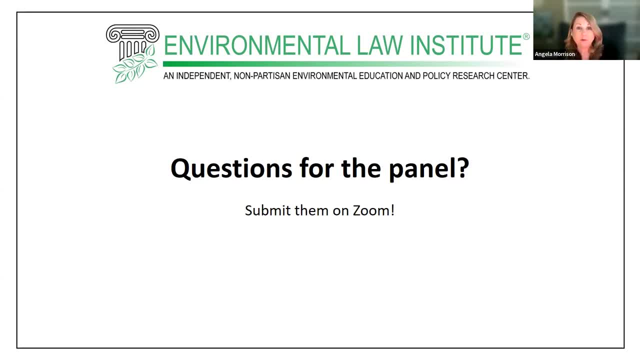 for the Biden administration either. So we're not really seeing a lot of that enforcement, but just know that big initiatives like that can't exist. And we didn't really see a lot of citizen suits, although, as I mentioned in my prior remarks, 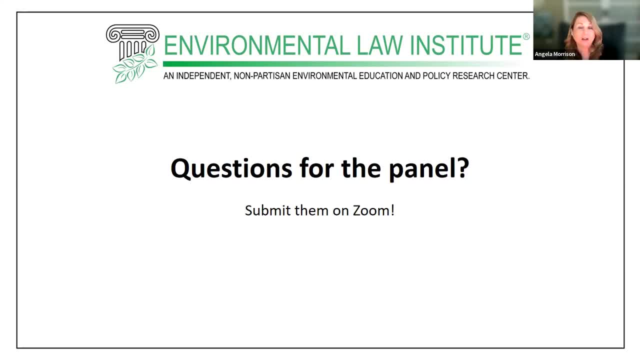 non-governmental organizations and neighbors can take advantage of challenging PSD and non-attainment, new source review and title five permits, either directly or urging EPA to object and appealing EPA's decision not to object. Evan, what you came from? the office of enforcement. 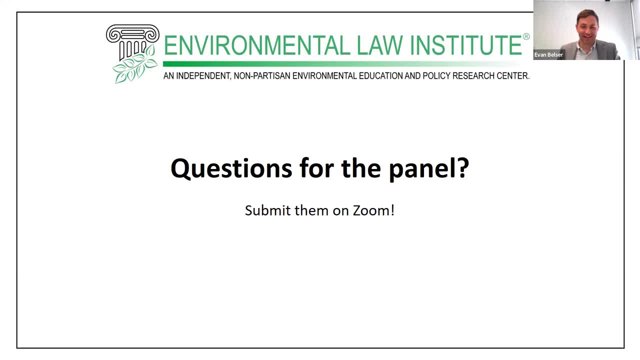 So you have the insights too. I did And I, I, I signed my fair share of 114s, Angela. So I never lightly, never took a lightly. but yeah, the the, as always, federal enforcement needs to have express authority from Congress. 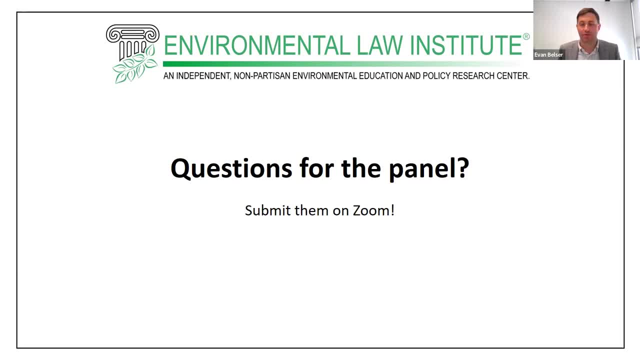 And so there's section one, 13 and section two of three, which are the primary sections that grant authority, civil and criminal enforcement, And so that's the playbook for federal enforcers They need. that's how they get jurisdiction at all in a court. 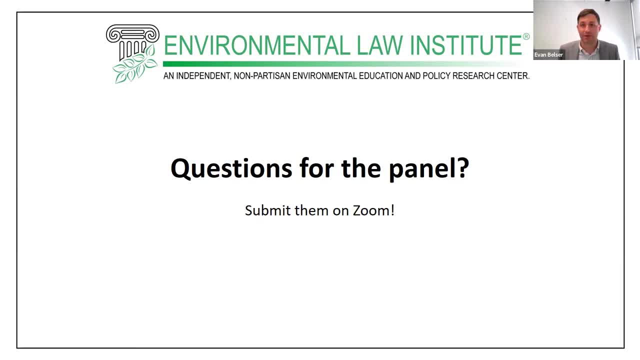 That's how they identify the elements of what it is that they need to prove with evidence to win a case. Angela's absolutely right. Mostly this is state enforcement and it comes in many different ways And I agree that information requests and reporting and all of that is sort. 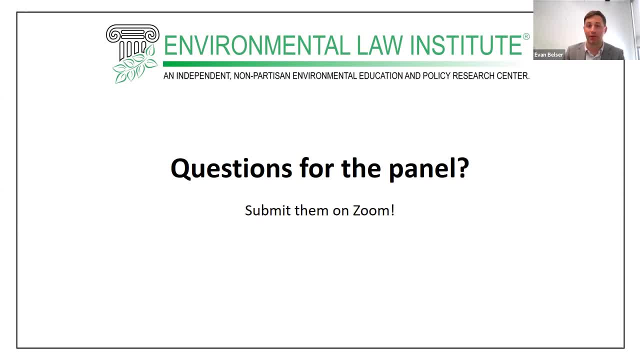 of the beginning side of enforcement or accountability at least. Enforcement in its purest form, of course, is enforcement case seeking remedies of some kind in court or a settlement with the threat of litigation for that, And so, as EPA enforcement goes, everything sort of works backwards. from that possibility I ran civil enforcement for the 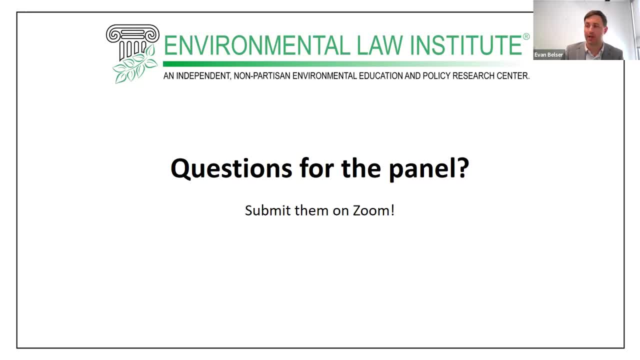 AIR group for a little while and ran mobile sources for a longer time, And I think one of the main points to share is that the agencies have a goal of compliance and not a goal of just catching. It's not a gotcha type of endeavor, but it's about securing the benefits of the program And 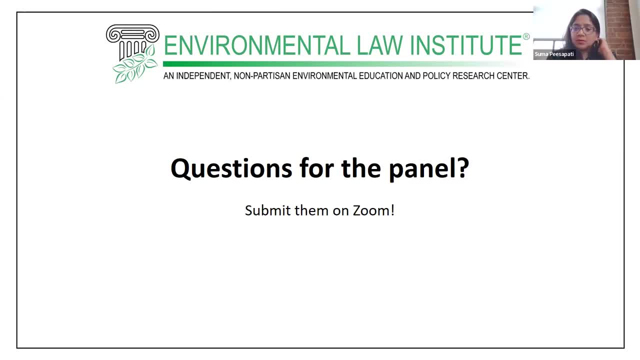 it's about ensuring a level playing field so that those companies that make the investments and hire excellent outside counsel, Angela, and do it right, are not at a disadvantage to those that are skirting the rules and are doing any number of things that are untoward. So enforcement also. 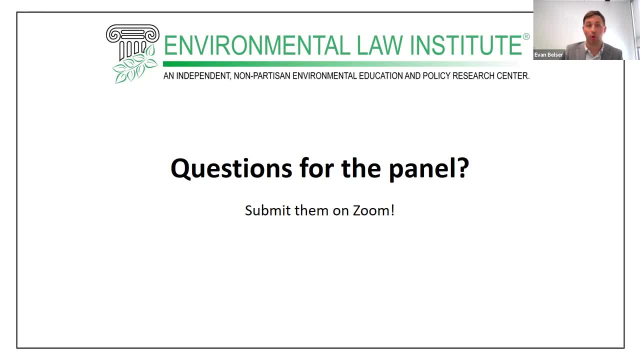 is a place where a lot of lawyers get employed, both within the agency, within state agencies, at the Department of Justice and, of course, in private practice, And so definitely an important area to focus. Largely, the cases don't go into extensive litigation or trial. 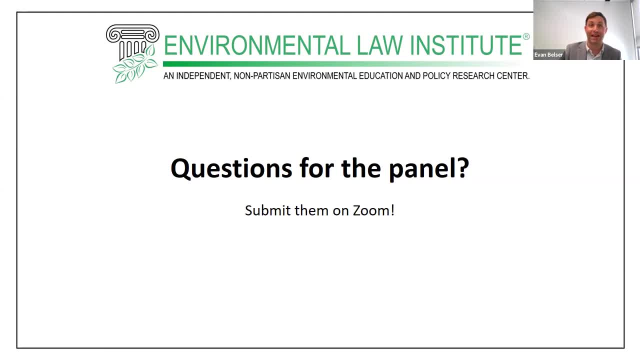 The nature of the disputes. even in the administrative context, where nine out of ten cases are taken under the Clean Air Act, mostly they're not with the Department of Justice, They're mostly with EPA. Primarily- it's overwhelmingly the cases are resolved. 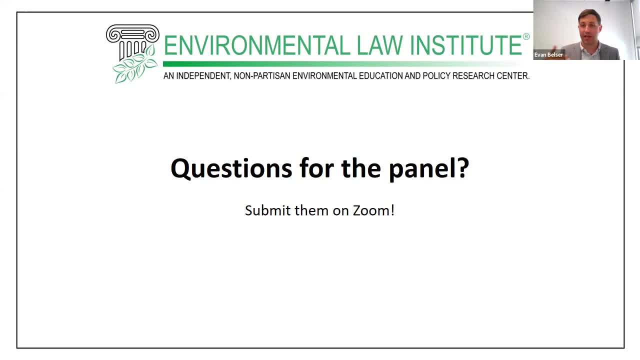 with a settlement concurrent with the complaint. So the agency would approach a company with a notice of violation or similar notice and have a regular back and forth, some regular cadence, to figure out to what extent the facts are complete, to what extent that establishes liability and what 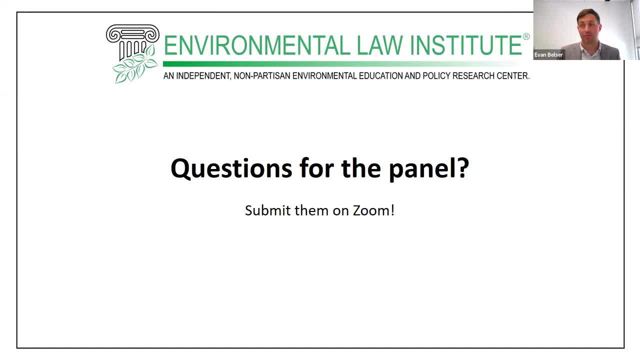 remedies you'd want to get from it. Many times, most times, there isn't actually an enforcement case. based on the early discussions. There's identified no violation at all or it's fixed. so there's no remedy to obtain anyway And there's no reason for the agency to come in seeking specific remedies. But where they do, 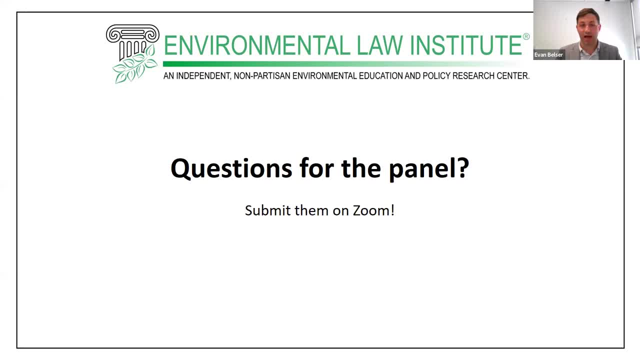 it's any number of things. The Clean Air Act has expressed authority for remedies at law to get civil penalties and remedies in equity, which are anything else that the court could conceivably order with its equitable jurisdiction, So civil penalties are often part of it. 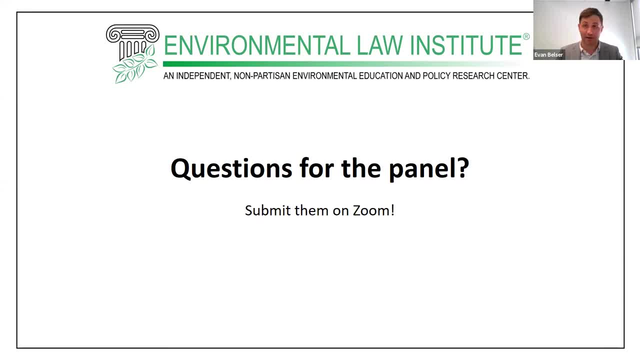 And that is the amount of money that the company arguably shouldn't have made a legal economic benefit, plus some additional amount. that's a gravity-based penalty. It's meant to sting and deter that company, specifically, deter the industry generally from committing the types of violations at issue. 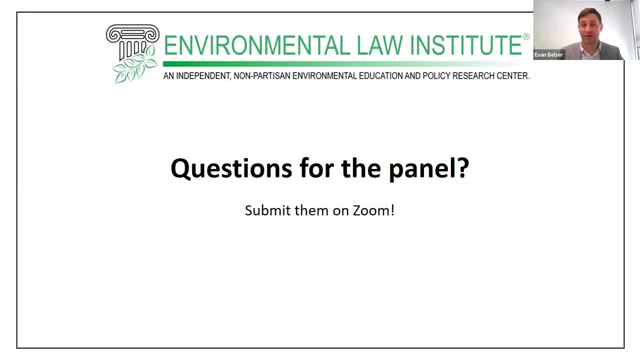 And besides civil penalties, often mitigation is common Where there has been excess pollution. what is it that can be done going forward to account for that? And it's in the air context. it's quite different. If you have a polluted wetland, in theory you can maybe clean up that wetland, But if the air 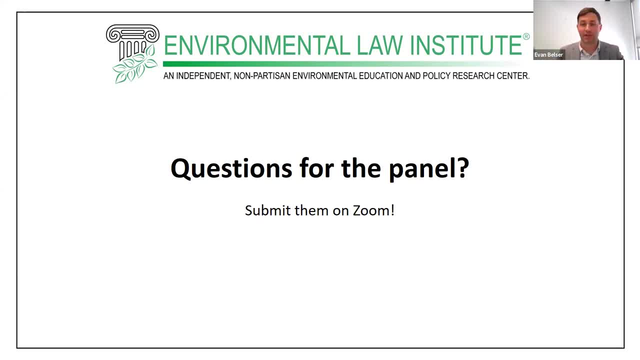 has already been polluted, the best that often can be done is a program to reduce emissions of the same type of pollution, maybe in the same area, going forward that would otherwise have occurred, even lawfully lawful pollution, And so, for example, buying up old, dirty diesel trucks. 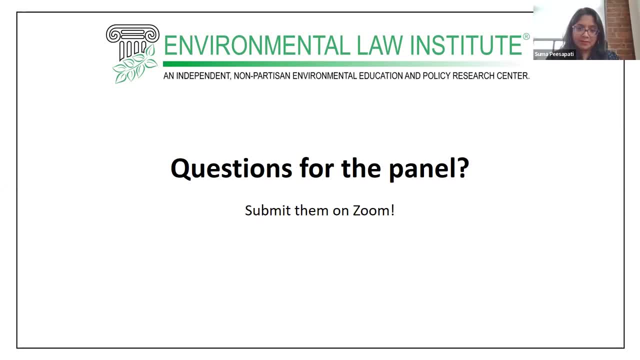 and scrapping them and recycling them and getting those out of the air And so, for example, buying up old, dirty diesel trucks and scrapping them and getting those out of the air And so, for example, off the road. that's a way. it's a type of example in a recent EPA case. Besides that, 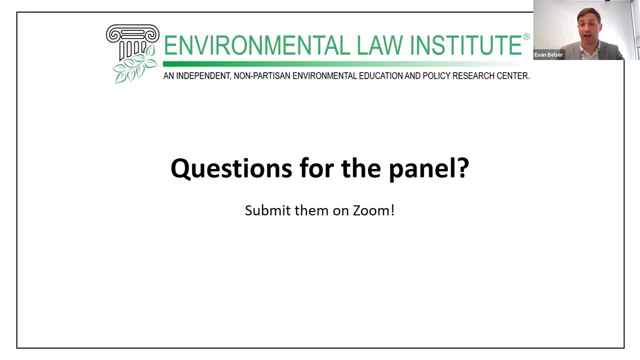 there's also injunctive relief just to prevent future violations. Sometimes there needs to be very prescriptive and intense plans with third-party oversight and all the rest to be sure that the project gets done. the controls get installed on the stationary source or the company. 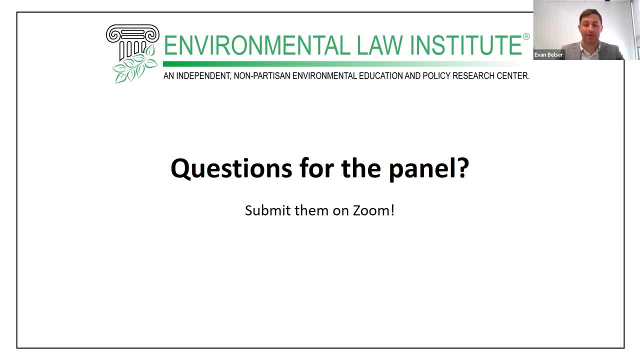 manages themselves to prevent future violations, And there's a few other types of regulations that are in place. There's a few other types of regulations that are in place. There's a few other types of remedies, like supplemental environmental projects, and a few one-off things like the zero emission vehicle requirement in the Volkswagen case that sometimes 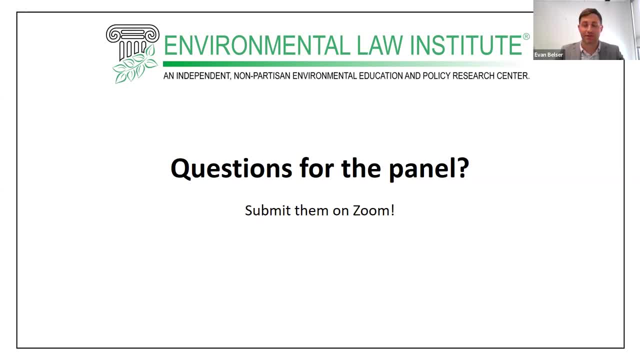 suit the facts and are parts of the ultimate resolutions of these cases. Criminal- absolutely right. I won't say much about criminal enforcement, but Angela's absolutely right. There's been a lot on asbestos. There's been some criminal cases against corporations or individuals at the. 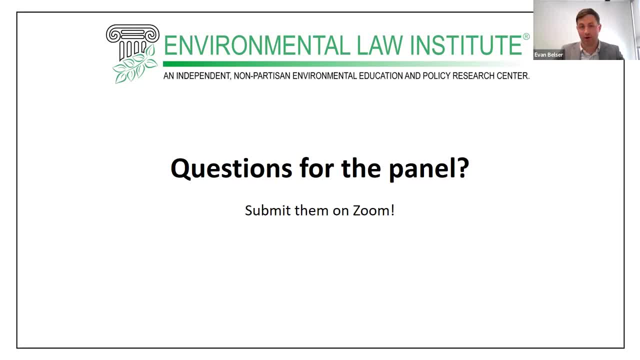 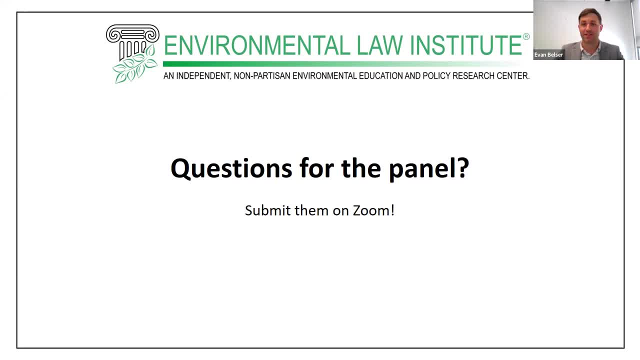 a lawyer for Hyundai who lied to the government in the course of responding to information requests. So, young lawyers, if anyone's going to go to jail, it's not going to be you. That's not worth it. So there's all kinds of examples where there's both a criminal and a civil enforcement effort. 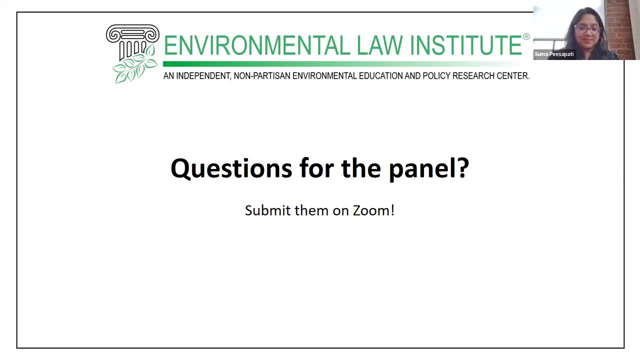 that are complementary and not necessarily overlapping. Thank you for all of that. I mean just to pick up on some of these themes, I think from the state level. you know, it's kind of a kind of interesting because when state rules are approved by the federal EPA, they're federalized. 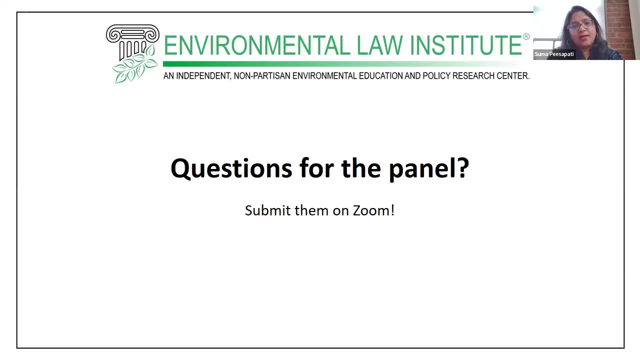 And so they're obviously enforceable under the Clean Air Act, but they're also enforceable under state law, So they preserve both this dual state and federal character, at least here in California, And so some of those same requirements can be enforced in state court using state causes of. 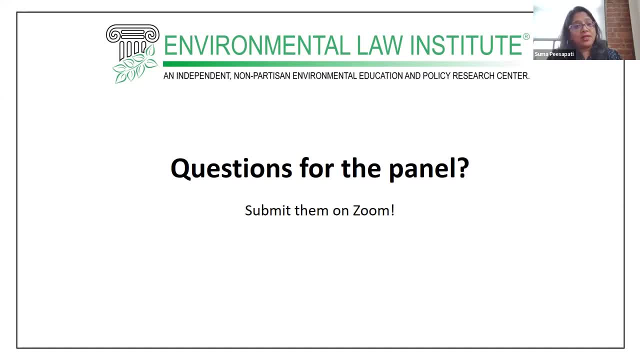 action, And so I think it's kind of interesting because when state rules are approved by the federal with respect to our air district, we actually have a quasi-judicial arm, a hearing board, administrative body that can also hear some of these disputes and issue rather swift. 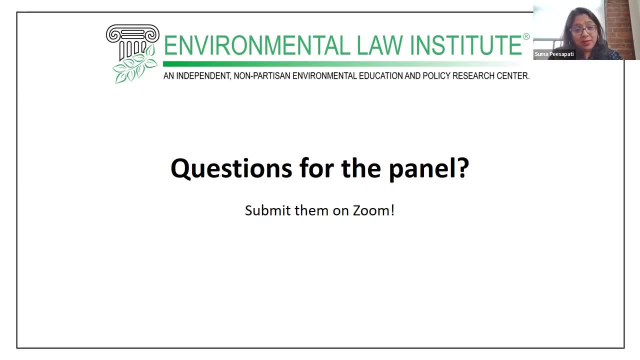 you know cessation, abatement orders to stop the violation. You know another important piece of EPA's authority and when it brings cases in federal court and there's a consent decree, as Evan mentioned, often there's like a complaint and a consent decree filed at the same. 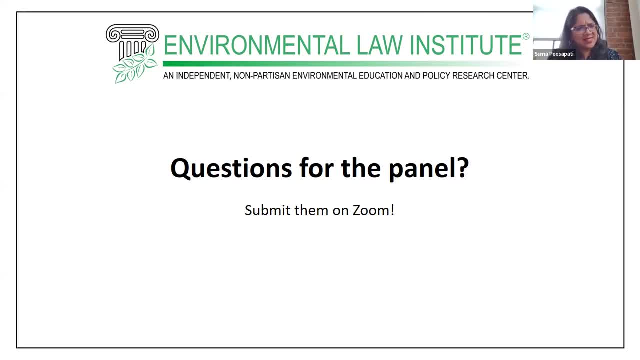 time the public has an opportunity- usually 30 to 60 day, I think, public comment period on that consent decree- to offer their views on whether the remedy for the violations you know serve the public interest. You know supplemental environmental projects are something I think. 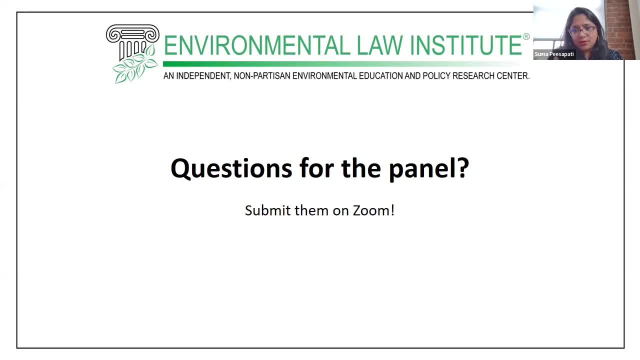 up to 50% of penalties can be directed to SEPs under federal law And you know we've seen some really interesting projects emerge from that opportunity, like an asthma clinic, for example, in a refinery community. So there's a lot of interesting work being done. 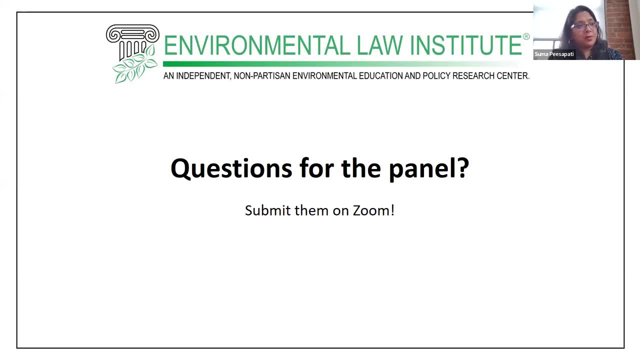 you know deterrence and when we talk about penalties, deterrence and you know ensuring that profits gained from the violation are removed are obviously kind of threshold questions in assessing penalties. So yeah, lots to say there. You know one question that came up that 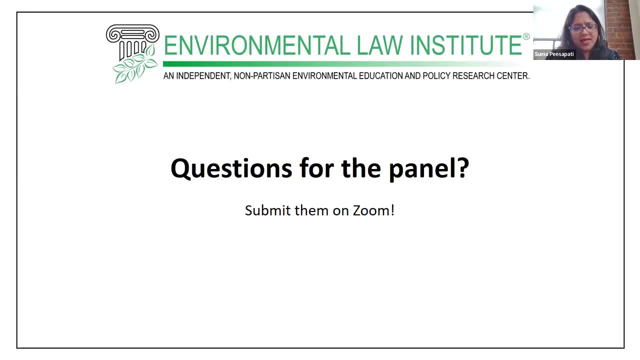 is just on my mind- and I'm sorry to kind of switch things up, Evan- is whether some of the mobile source reports you know are going to be, you know, are going to be, you know, required for citizens to wear a citizen suit, And are those requirements are enforceable by? 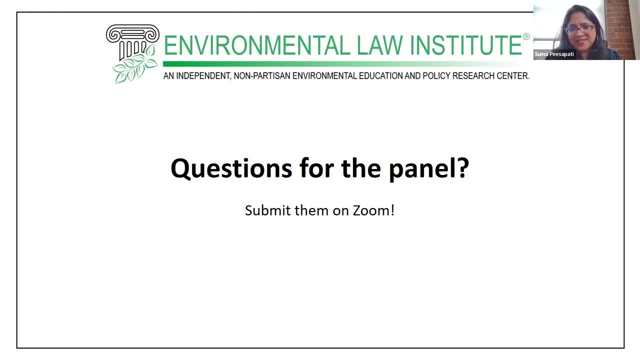 citizen suit And I've never confronted that question before And you know, I'm wondering if you happen to know the answer to it. It was an interesting one, that just kind of caught my attention. Yeah, that's a whole new area where there's not, I don't think there's- clarity there. 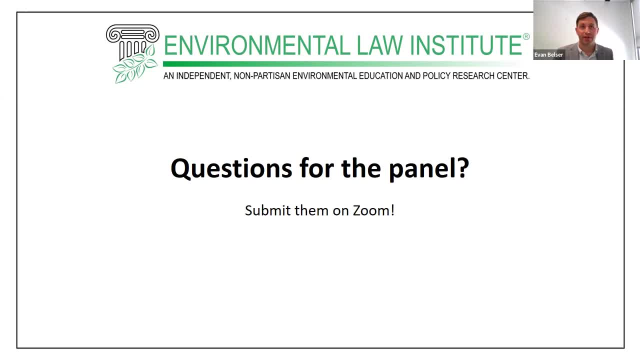 You know we have a case in the 10th circuit. That's one to watch. That's in the classic sense of citizen suit right. independent practitioner with deep experience doing citizen suits on the stationary side, partnered with the physicians group in utah and took the case against an aftermarket. 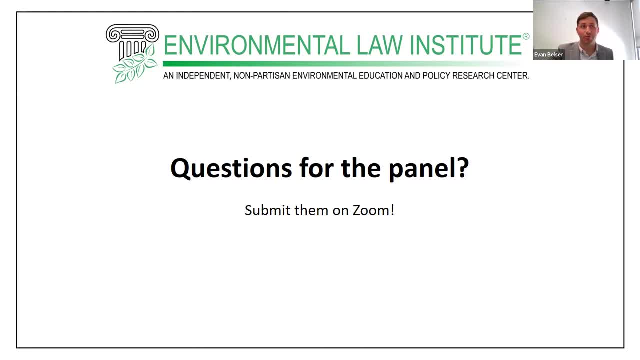 defeat device seller people who make and sell products specifically to remove emissions controls from trucks and uh. and there the uh chief judge for the district court said: yeah, that's, there's, there's, there's jurisdiction here, um, so that's, that's one example, there's some, i think. 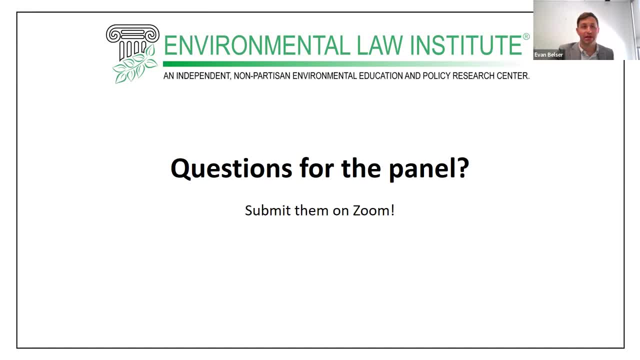 dicta and ninth circuit opinion in the volkswagen case. about the county's ability to take enforcement cases, there's very little. there's scant precedent on citizen suits under under title two. there's citizen enforcement of state programs- to further your point, suma, for example, i think. 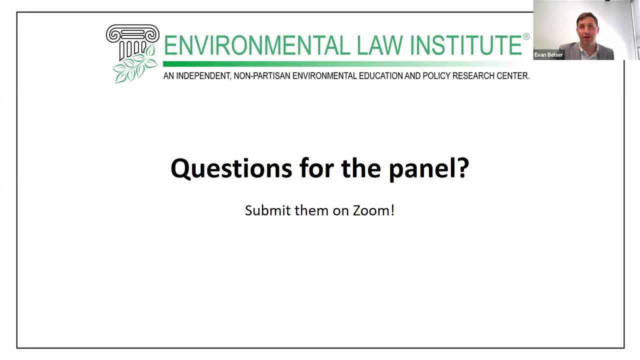 massachusetts and maybe new york, allow people to enforce anti-idling requirements and that's not necessarily under the federal law but it's under the sip and the state legislature made that a cause of action in state court, so that that's definitely an emerging area. there were a few rare uh situations with, for example, in in commercial. 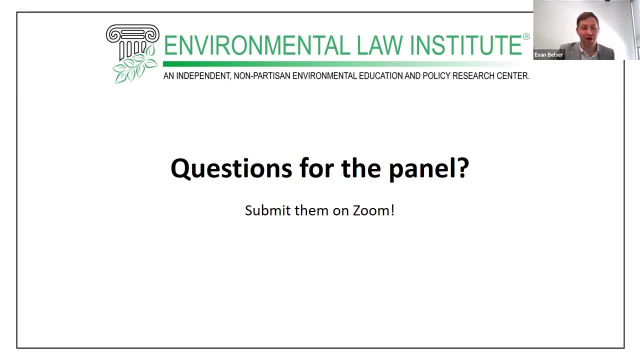 disputes in the renewable fuel standard program, uh, where a company was going against whoever sold them bad credits, they decided to to go get a declaratory judgment and they did that using a citizen suit provision and it was never really litigated, but they they invoked section 304 as a 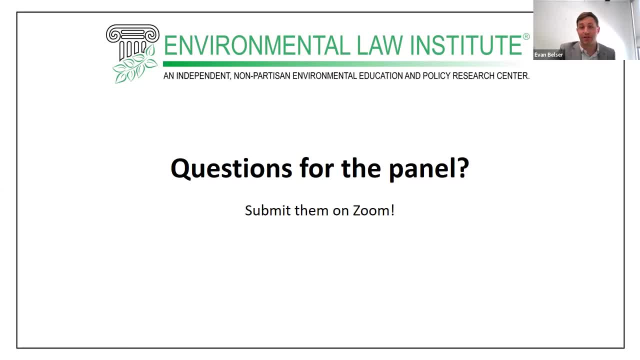 to to try to further their interests and and apparently that was because you can get fees if you win. so pretty clever lawyering there. but but um, and and yes, a citizen suit, i suppose. so that's yeah, that's, that's one that's still in my mind really up in the air. 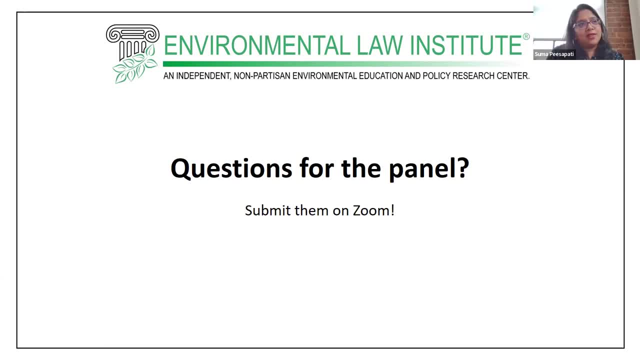 and i guess, on the subject of citizen suits for those states that don't have independent state law, uh right, a right of action. i i think i've seen a number of states um outside of california who have a lot of evidence that the state has an interest in the use of citizen supervision. 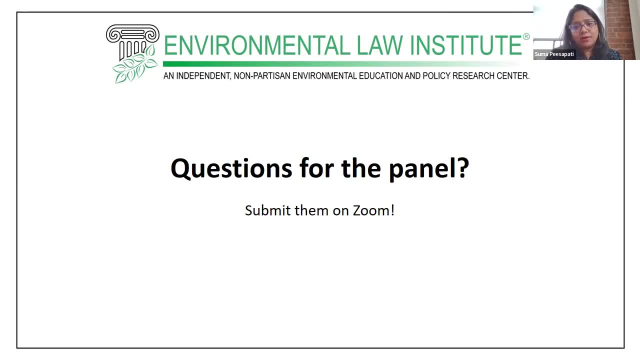 to bring cases in federal court- clean air act violations in federal court, if i'm not mistaken. so, um, it's a really powerful aspect of the statute. democratizes in many ways, uh, the enforcement capacity um great well, that was super interesting, um, but i'd like to um switch gears once more to 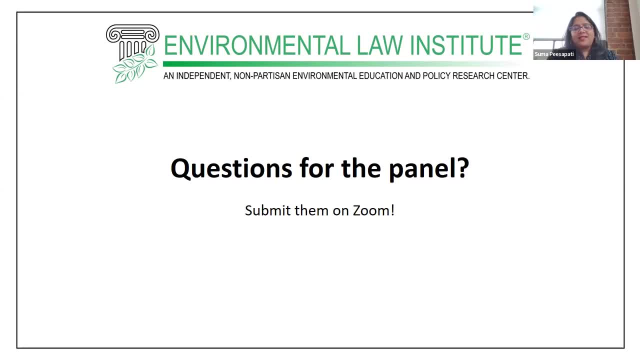 talk a little bit. come back to the topic of environmental justice. you know, obviously it's. it's an issue that is um starting to get some well-deserved recognition, recognition um more so, i would say in the past um pretty much at all levels of government, which is 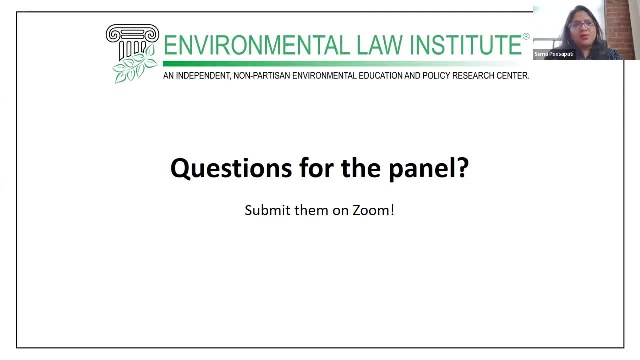 really exciting um to see um. so i thought i might start with um providing a bit of a summary of some basic ej concepts and then post some questions, if that's okay. so, um, so when we talk about environmental justice, we often talk about concepts of um, distributive justice and procedural justice. 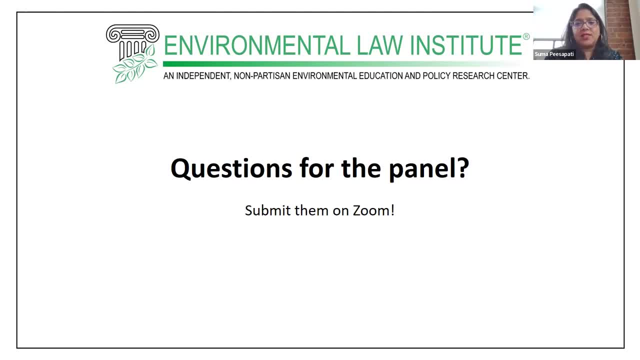 so what does that mean? so, with respect to distributive justice, you know there's this question about who carries um environmental burdens and benefits right um. i want to make clear that environmental justice isn't just about um pollution disparities, but also where desirable places reside right and um. the former mayor of of stockton, um, michael tubbs, um stated this. so 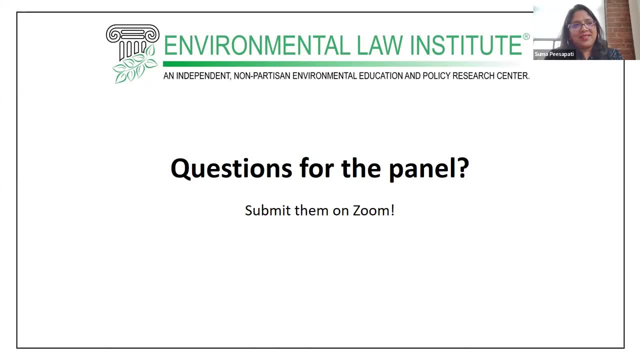 beautifully. when he explained um, he described his view of ej, of environmental justice, and he said: you know that to him it's a question of who in the city gets to enjoy, um, the basic dignity of things like shape a big beautiful tree on a hot summer day, right, and so i think often there's, and understandably, 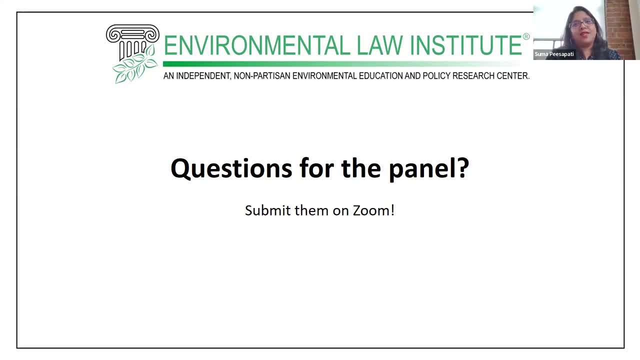 a lot of emphasis on um. you know the concentration of pollution of all sorts, including air pollution, but it's important to remember kind of the um. you know the other piece of the equation: who gets the benefits of um, um of of. you know um beneficial uses. basically, another is another concept i mentioned is procedural justice. so how's the process? 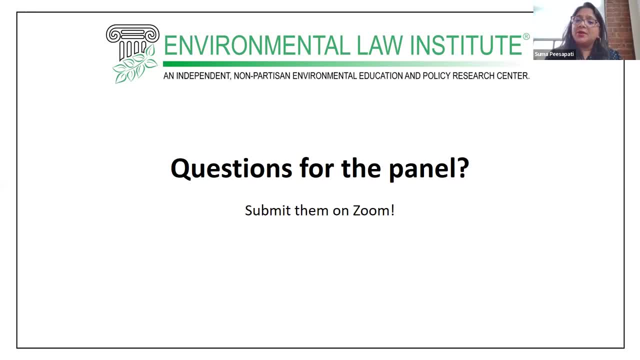 for government decision making? um, how does it occur? right, is there a meaningful and fair opportunity to participate in things like permitting, in enforcement, um, in the rulemaking process and other, you know, critical government decisions that impact uh communities? right, and so embedded in this notion of procedural justice, are things like: 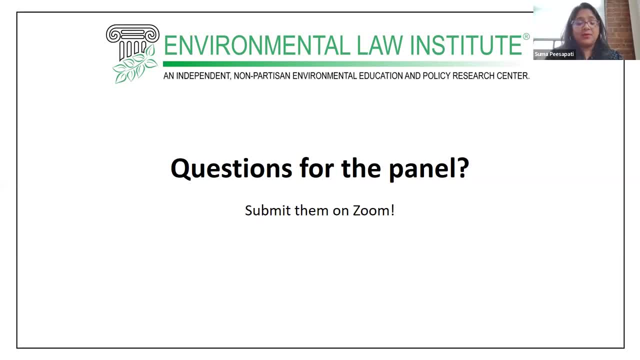 language access and translation right. um the timing and location of public hearings: um you know public hearings related to permit actions, rulemakings. you know government, government decision making. um whether the relevant background materials related to a decision are accessible to a lay audience right, both physically accessible, but also um just in the way that they're drafted. 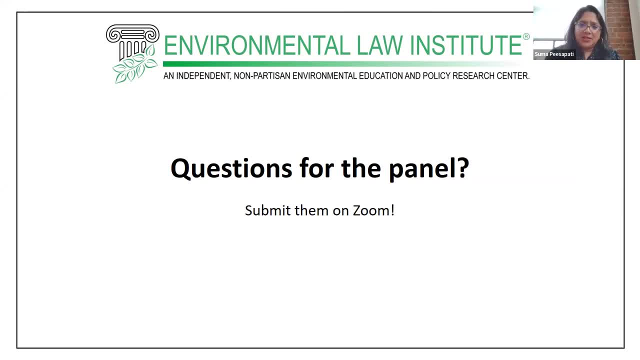 um is the information um catering to a lay audience? um and, of course you know, another key aspect to procedural justice is whether the public and affected communities actually have the ability to influence the outcome of the decision. so, once um feedback is taken from the public, how is it um absorbed and how is it translated to action? 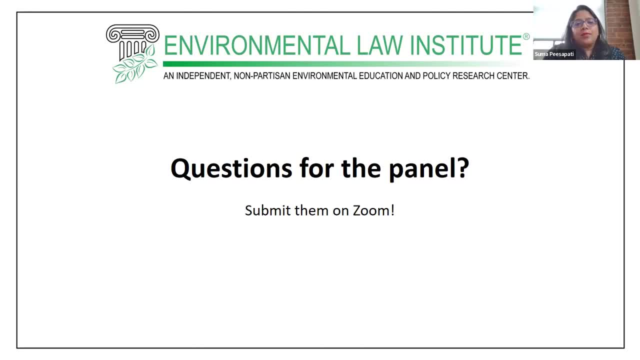 by government agencies. um. so ej scholars and advocates will often cite to another fundamental ej principle, which is that communities have the right to speak for themselves and have a right to transparency and accountability on the part of uh government actors and government action. um and so, if you're interested in learning a little bit more about some basic ej principles, 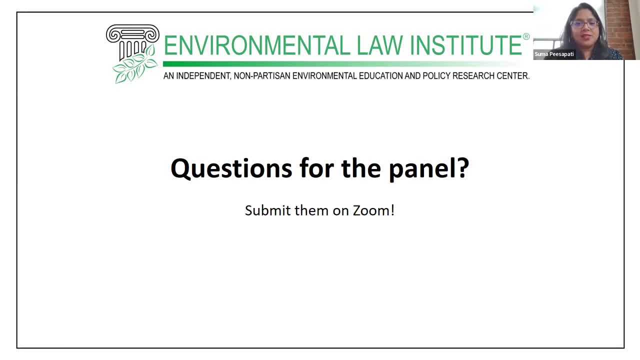 um doing a bit of a deeper dive into the subject, i might suggest uh taking a look uh at the 17 principles of environmental justice that were created um in 1991, um in an ej summit in washington dc. where ej leaders and advocates from around the country convened um to develop those 17 principles. 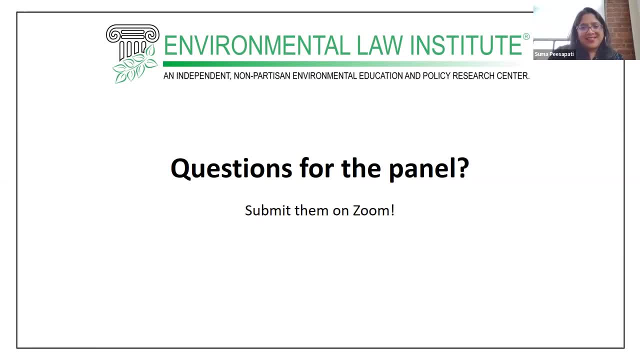 um and those are widely available um online. so i guess, with that um very simple and basic background um, i wanted to open it up um to the panelists to talk about um. you know ej um in executive actions and maybe we can start with evan um. i know that there's um an environmental justice enforcement. 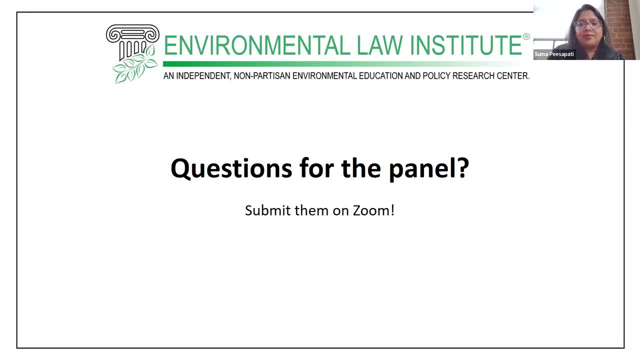 policy that recently emerged from uscpa. um, maybe you can talk a little bit about that if you don't mind. sure, yeah, the. you know, in the federal government there's a few different places where ej has been identified as a goal and it starts with executive orders out of the white house. 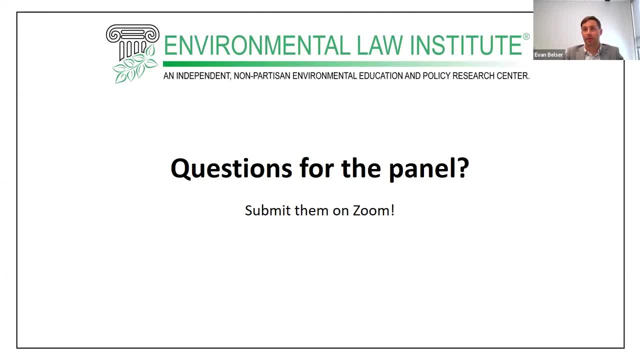 notably a clinton executive order which, at least with the results of the this week project, uh, especially after the election of um mayor- um, that it's not the current president kimchi- one of those things is a peace plan. i think that's what you're talking about. 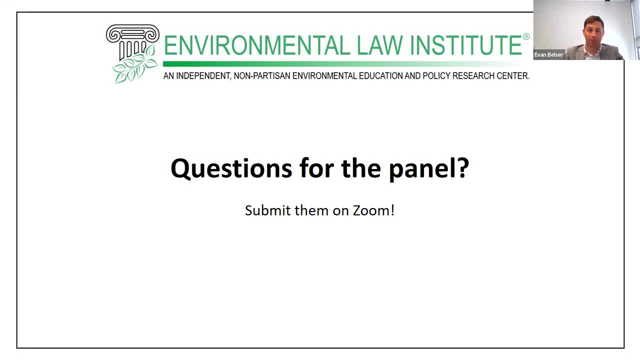 right. so there needs to be not only a good outcome, we need to. you know, the agency wants to protect people's health, and especially people whose health is most at risk for any number of reasons, including um, including regulated sources of air pollution, but also aggregate exposure from. 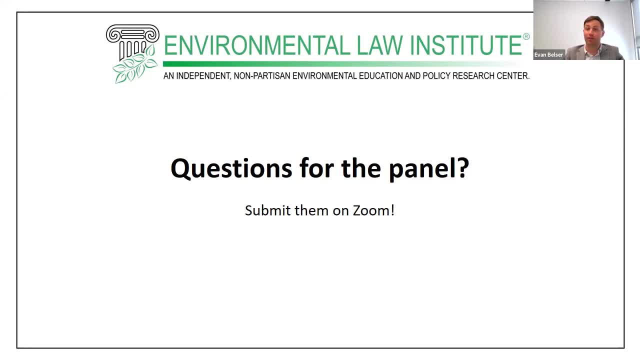 other things that maybe aren't in the jurisdiction of this or that statute but matter for the people's health, the length of their lives, but also a lot of process points too. so how to get people, uh in the community, more informed about, involved in rulemakings, in permitting decisions, in 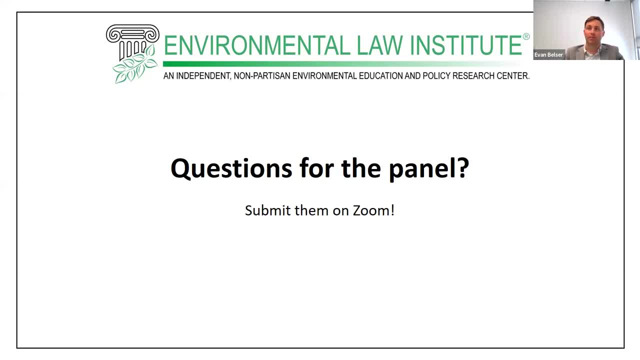 enforcement, including, you know, special focus in science that underlies all these rules to. you know, really make sure there's a hard look at and consideration of what science is can show. tell us about protecting people who need that protection the most, and then you know a lot of work on on. 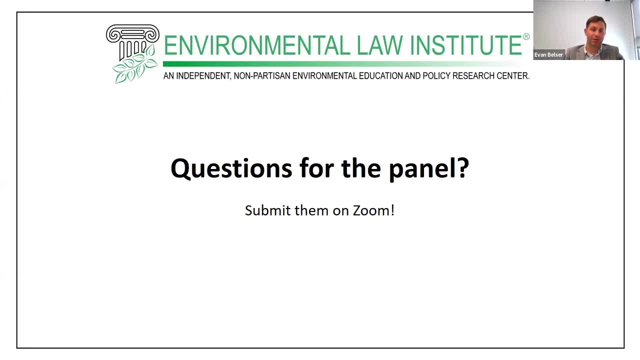 trying to integrate environmental justice goals into the governance of different federal agencies as they work together and, of course, epa with with the states and with tribes. you know, i think most notably doj- just in may of this year put out enforcement strategy which created a new office, office of environmental. 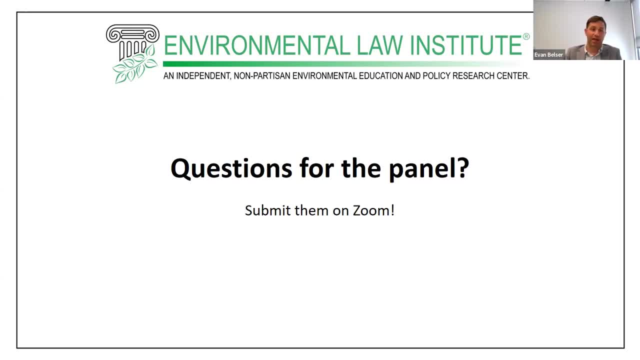 justice, identified how to prioritize cases that serve ej communities and, and there as well within the department, new governance, to be sure that the resources that they have are are down to the level that they need to be in order to be able to do the work that they need to do. 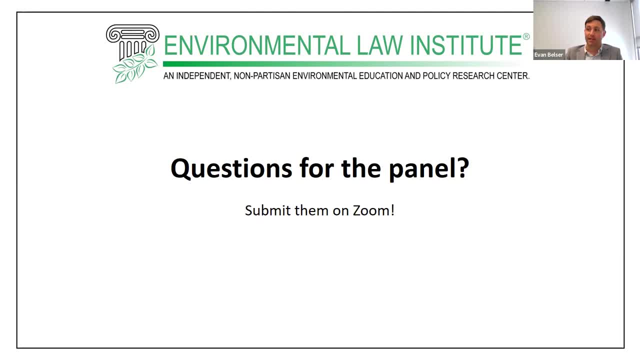 in order to be able to do the work that they need to do. in order to be able to do the work that they need to do, dedicated to to helping those communities that need it the most, uh, that are overburdened with air pollution, that are overwhelmingly communities of color, and so that that all matters quite a lot. 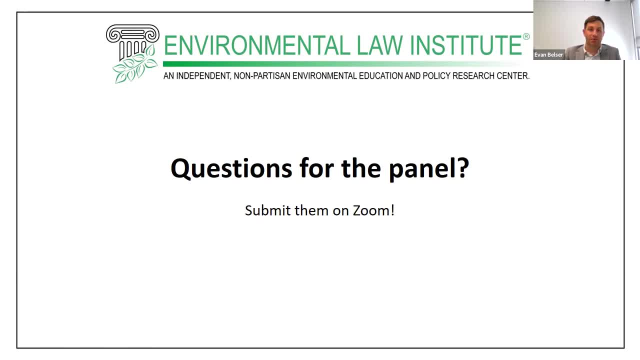 i think that's good policy, my own, my own opinion. i also think that it only goes so far, as long, as you know, the government has very, very little funding. you know, after my, you know, decade at epa, i will tell you that, certainly in the stationary context, the prioritization already, 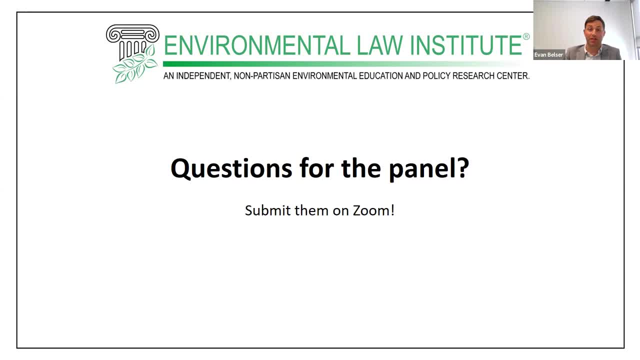 reflects where it will help the most, you know already. reflects where we're hearing from the community- uh, where we were hearing from the community when i was at the epa, and so while i think this, this is all value added, um, it might not necessarily amount to a dramatic change in how. 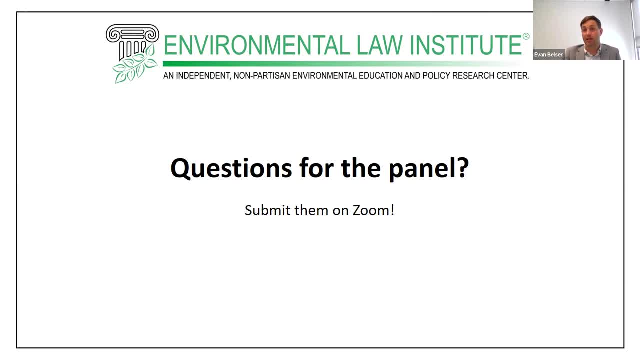 epa does enforcement at least, and i was less involved with rulemaking so maybe there's better options there. but primarily the limitation has been on resources- state and federal resources- to not only do the underlying work, to set the rules and take the cases that need to be taken. 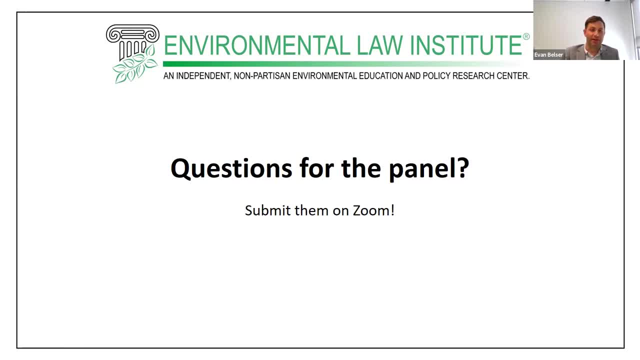 but also to engage the community. and there's a lot of complicated factors, like you know. we have at the federal agencies, understandably, policies that say, with enforcement, you keep it to yourself, this is federal law enforcement, you don't go telling everybody about it, but now you know. 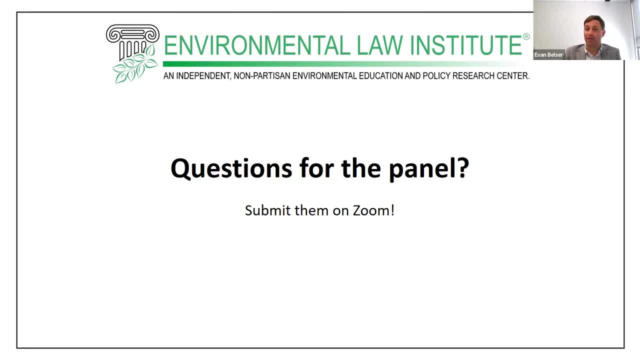 there's new policy that says engage the community about it, and that's tough, and i've talked to communities who want certain things out of an enforcement case, but those things they want don't necessarily align with what's possible, and so i think that's a really good point. i think that's. 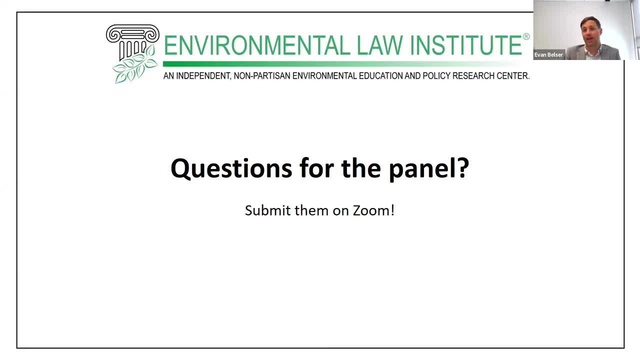 possible in that enforcement case and defendants aren't just going to hand it over. so there's a lot of work to do here and i think for quite a long time now there's going to be a period where it's going to be awkward and unsatisfactory for many people putting a lot of these principles. 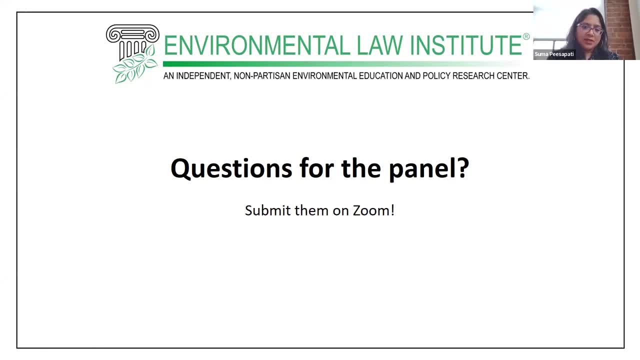 into action. thanks for those thoughts, angela. did you want to add anything to that? just in the In a permitting context, it makes, I think, more sense to focus on EJ if it's a brand new facility, rather than objecting to Title V permits for existing facilities unless they're not in compliance. 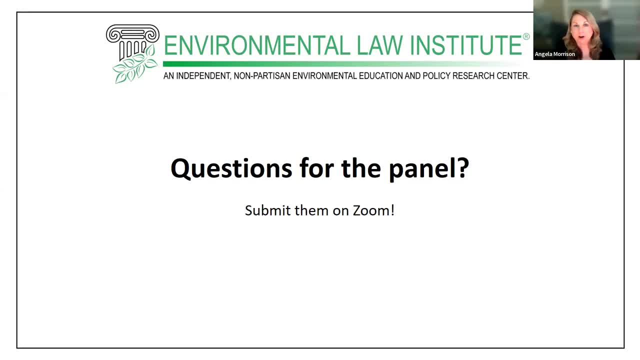 If they're in compliance with the standards and there are not known human health risks, it doesn't make as much sense to me to try to deny a Title V renewal for an existing facility. as long as they're in compliance, Yeah, Yeah, I mean that's a big. as long as right if they're in compliance. 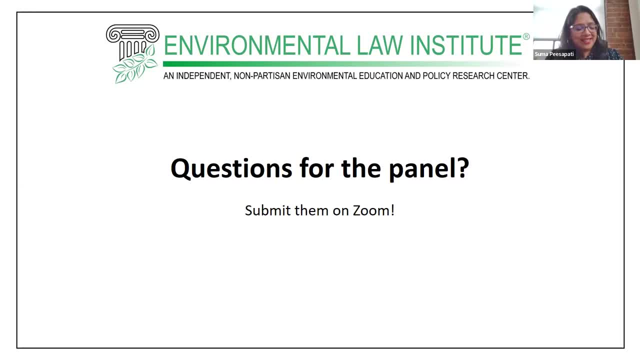 Right, Right so, but I guess What I'll add is that to this conversation is that I think there's a lot of innovation happening at the state and local level on the subject of environmental justice. We're starting to see it, as you mentioned, Evan, also at the federal level. 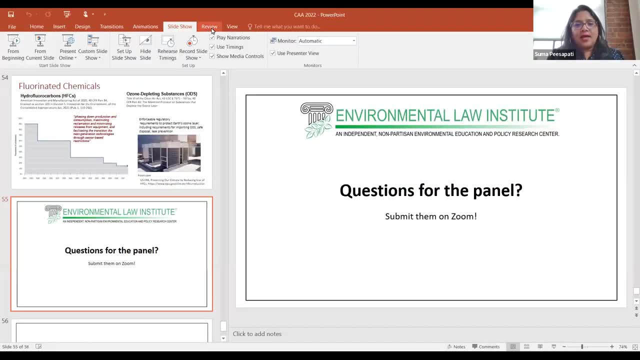 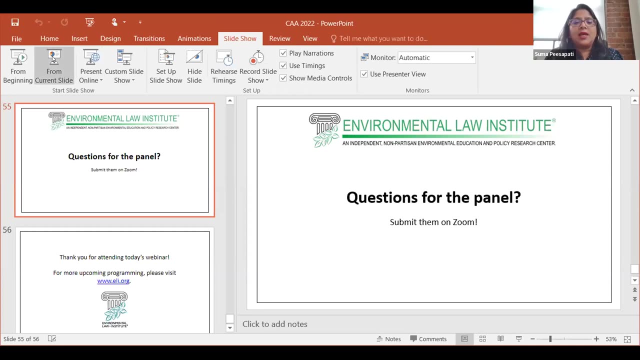 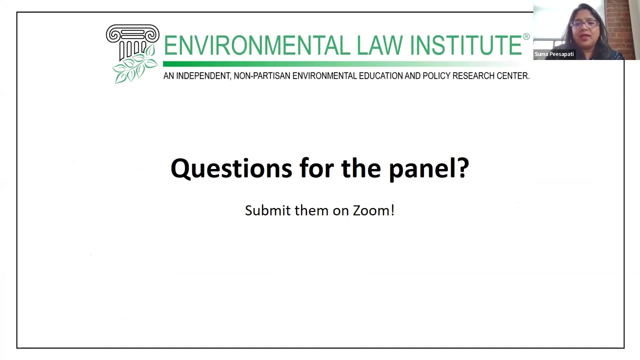 But you know, using, I guess, California as an example, we have initiatives like SB 1000.. Which requires EJ environmental justice elements to be included in general and specific plans at the city and county level. We have seen local jurisdictions applying their broad police powers to establish heightened land use permitting requirements in EJ communities that require, you know, an analysis of cumulative. 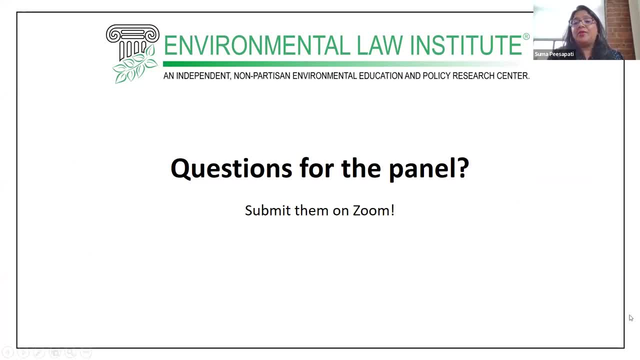 And synergistic environmental impacts When there's a new permit or permit renewal, actually for existing sources. we're starting to see that We also have something that's specific to air quality, which is maybe 617.. Which requires local air districts to partner with EJ communities- affected communities- to develop. So it's more a first step, It's a second step, It's a second step, It's a second step. So we have: It's a second step, It's a second step. So we have to think about where we're going to start. 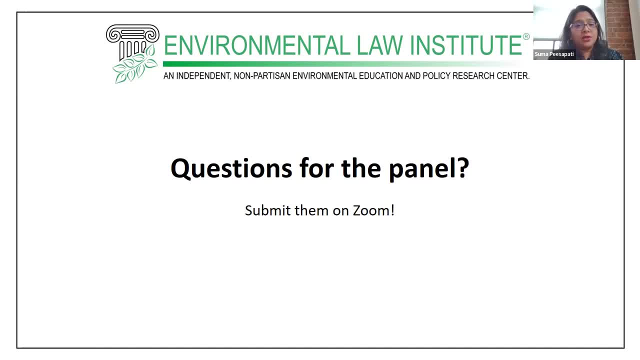 So we have to think about where we're going to start, develop tailored air quality monitoring and emissions reductions plans in those communities. But since we're here to talk about the Clean Air, the Federal Clean Air Act, you know, there, I think. 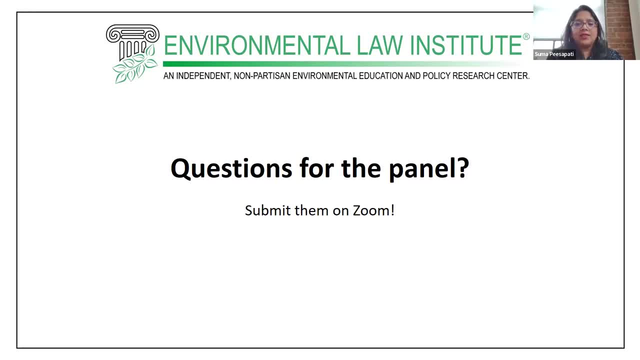 there are also certain provisions of the statute that could be leveraged to better serve environmental justice. You know you mentioned permitting, Angela. you know Section 173 of the Act requires an analysis of alternative sites and other considerations to show that the benefits of 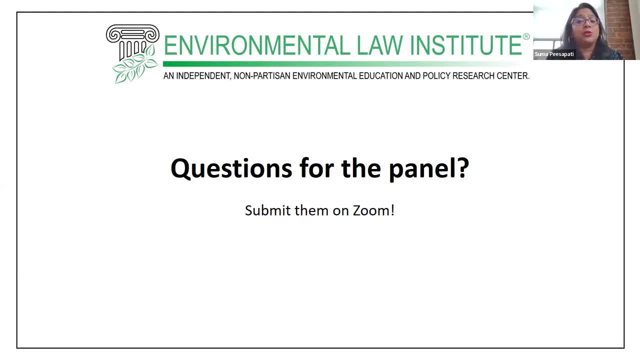 a proposed source outweigh the environmental and social costs that result from you know its location. I think this requirement could be interpreted to allow consideration of cumulative and synergistic impacts in the permitting of the proposed facility And, likewise, coming back to the concept of community-based science and participatory research. I think that Evan touched. 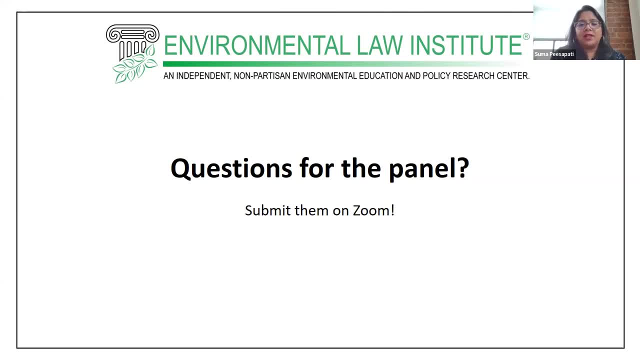 upon Section 504 of the Clean Air Act could allow for permit conditions that allow for things like community oversight of a facility's compliance. Yeah, and you know, we touched upon, you know, potential increased transparency in the enforcement process, right? Obviously, the bulk of the 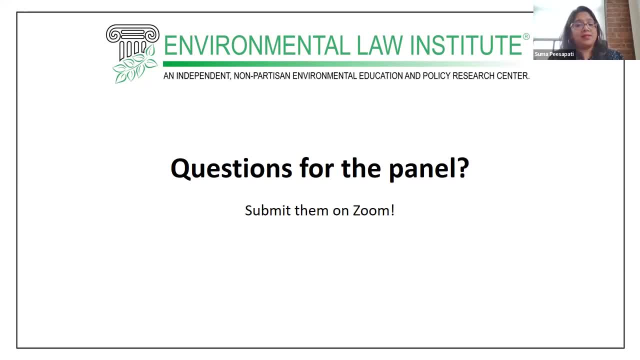 process is enforcement confidential, but there are ways to enhance partnership and transparency, you know, both from a participatory research, community-based science perspective in terms of identifying violations, and also at the back end and, as we discussed, the supplemental environmental project piece of enforcement and soliciting public input on how to craft SAPs. 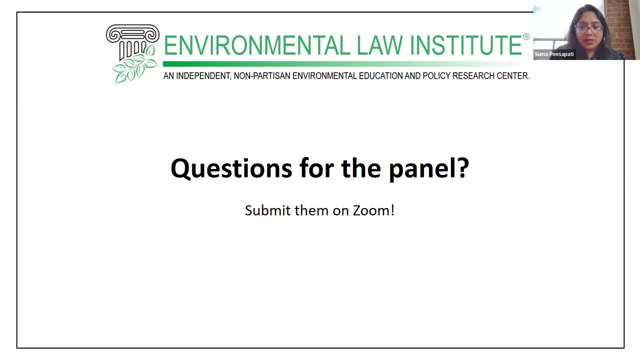 for example. So I know we're a little short on time, but I wanted to give Angela the opportunity to share shifting gears again, some practice pointers for our audience, which I think could be really useful. So, if you wouldn't mind, Sure, We had a question too in the chat box. 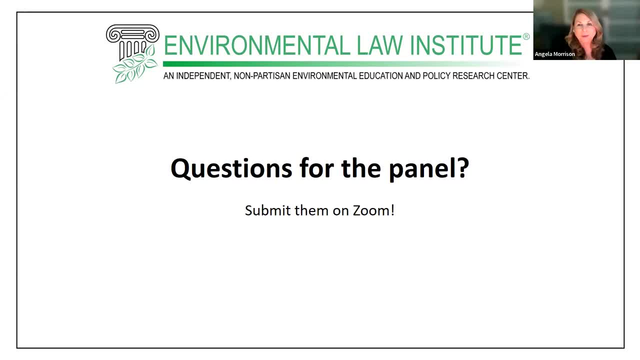 or in the Q&A, I don't remember which one it was. but you know it's never just static. you know These are the standards that apply And you get your Title V permit and you just operate, you know, for the next five years without. 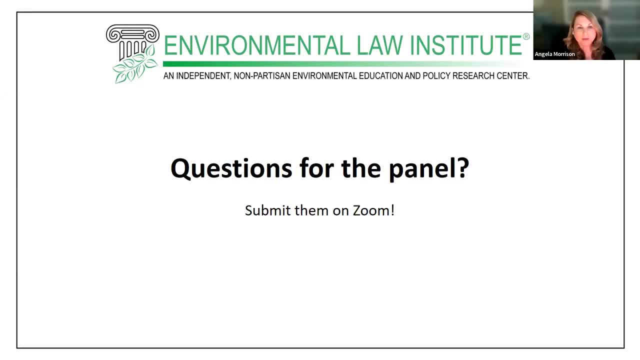 worrying about anything, because you might be making changes at the facility which could trigger a new source review. So it applies to modifications and SPS. If you're reconstructing one of your units and they're over 50% of the cost of the initial unit, you might be triggering. 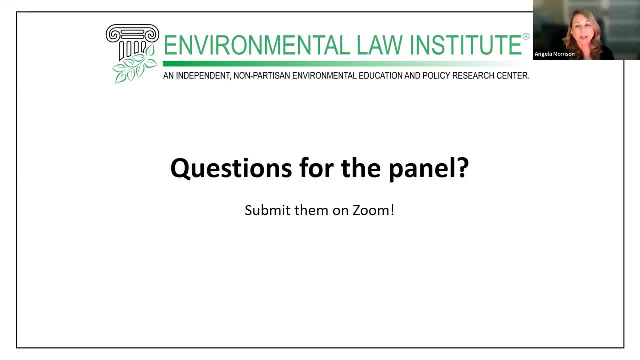 an SPS So you always have to be on the lookout for changes at the plant. There are also changes in the environment and there are changes in the environment and there are changes in the quality standards Every five years. those are under review. Sometimes they're kept the same. 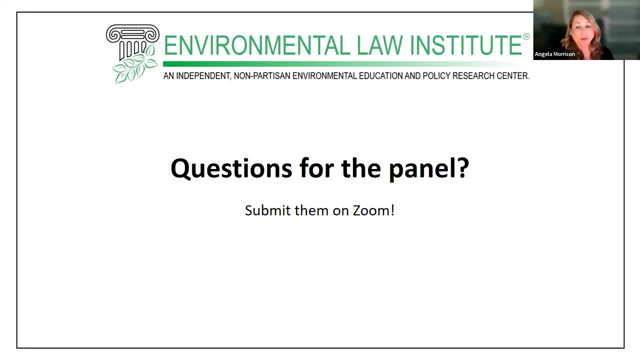 Sometimes they're lowered And so you always have to. you know the standards, you know the ambient standards can be lower. You could be under a five to eight-year review process of an NSPS or NESHAP. that could be lowered, And we recently there was a question about ethylene. 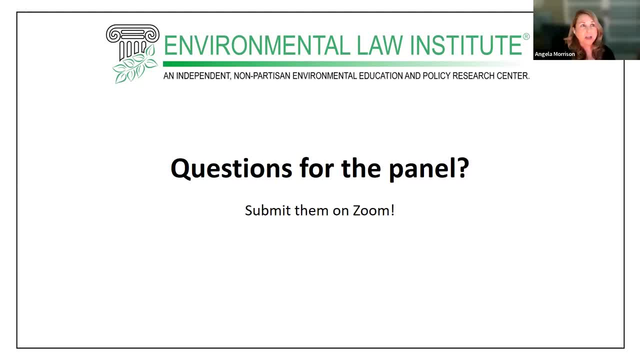 oxide and what happened there was. there wasn't really a change in technology during a technology review, But when EPA was looking at health impacts, they looked at a new study indicating that ethylene oxide facilities and their emissions, that ethylene oxide, would be a carcinogen. 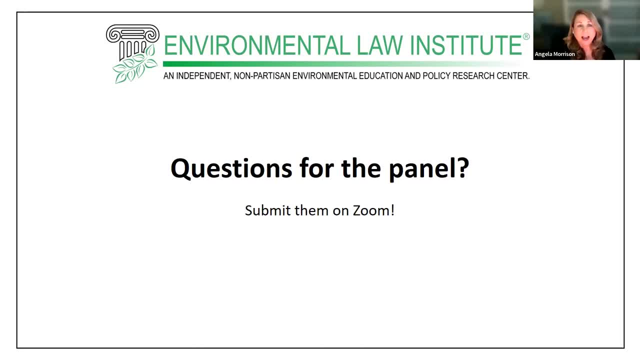 and maybe lower standards would be needed, And the residents near those facilities were very concerned because, all of a sudden, what had been a compliance situation was all of a sudden looking like there were ambient impacts of a HAP that were above and beyond the 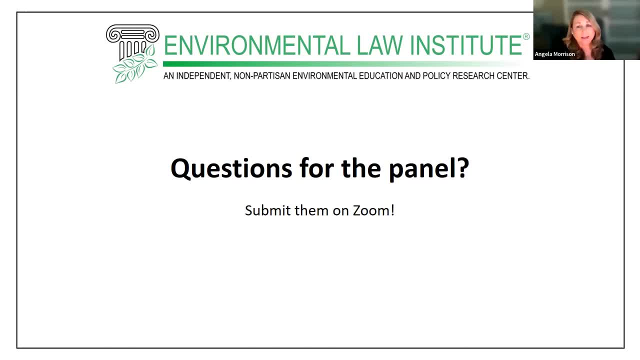 these screening thresholds, And so you know you always have to be on the lookout for new studies indicating that maybe there's a new pollutant. I said that you know there's a new pollutant being added to the list of 187. that could result in new regulation. There could be, you know. 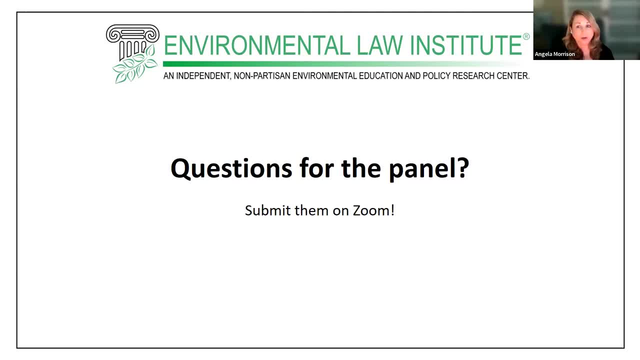 a change in the screening threshold, indicating that something is really a concern when you hadn't known about it before. The air quality models can change. where something was modeled and it looked like it was not causing or contributing to an exceedance of an ambient standard or a PSD increment. 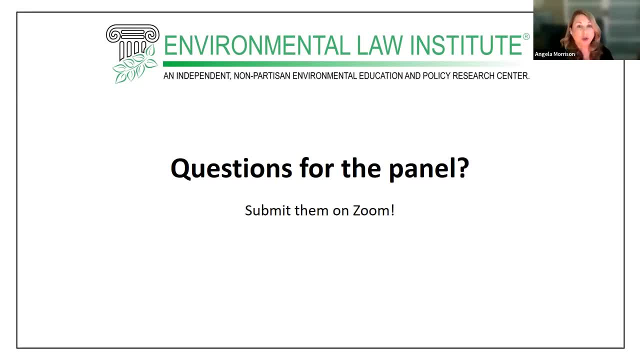 and all of a sudden, based on the new modeling it is, Maybe there's a new monitor put in a location and there was a question about what about? you know your local neighborhood corner where you see a lot of traffic? You know, maybe there's a new monitor put in that location and all of a sudden, 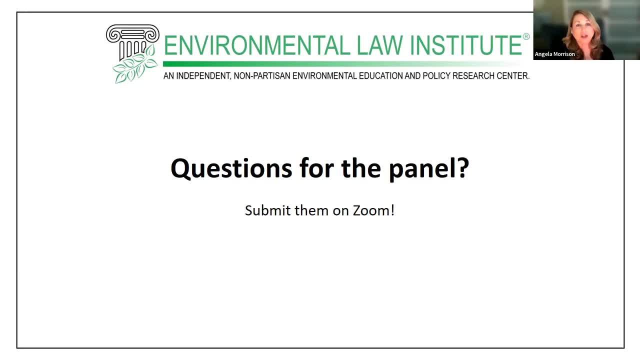 that area becomes non-attainment and you're subject to new permitting requirements or new emission reductions, And the non-attainment SIP requirements can apply to mobile sources too. So you know, there's just forever things changing in air and that's why air is a real interesting area. 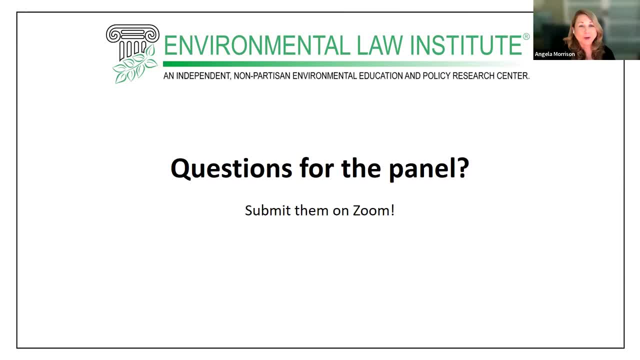 to practice. So we would encourage you to you know, continue your investigation of the Clean Air Act. Yes, Great. So if you're both open to addressing some of the questions that have been asked, any other questions by the audience, I'm trying to sort through some of these questions, I think. 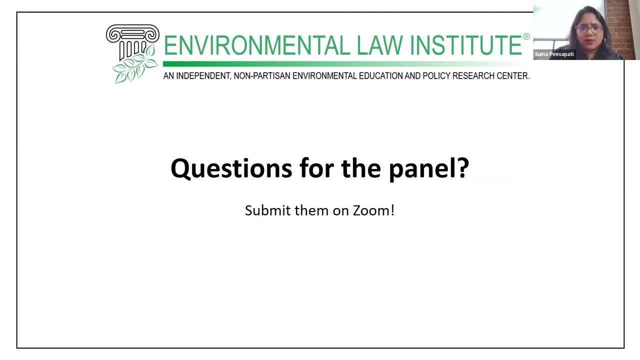 there was one asking why there aren't, why there isn't more use of the citizen suit provision under the Clean Air Act. Anybody want to take a stab at that? No, I'll start. I think that there's a lot of use of citizen provision in, certainly in a stationary. 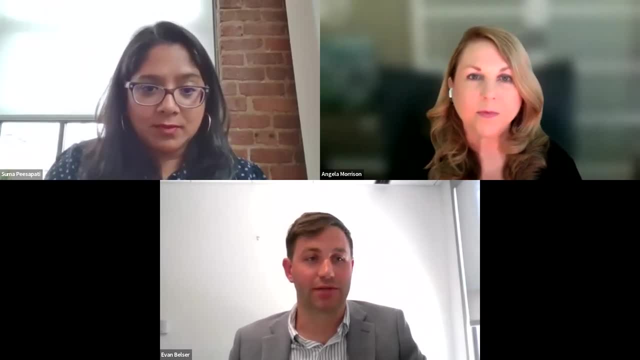 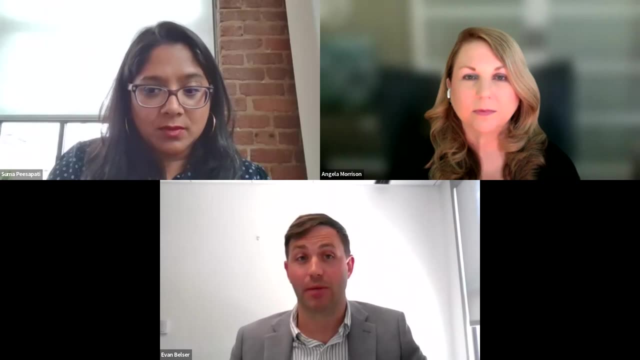 context, and I think that that is a product of the Clean Air Act. I think that there's a lot of use of the citizen suit provision under the Clean Air Act, Maybe two major things. One is access to information. Like Angela said, there's a lot of transparent information about what the facility. 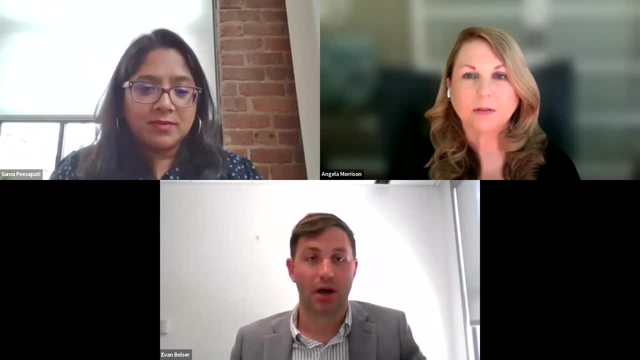 is doing and what its permit is supposed to be Also tends to be that it may be of more interest to a particular group of people that are going to organize and marshal the resources and the commitment to see through a lawsuit And for mobile sources. often it's spread out really. 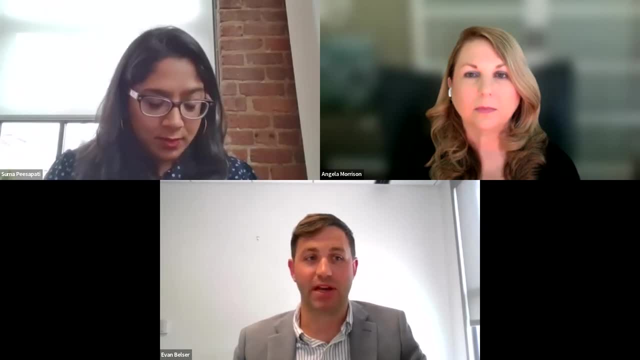 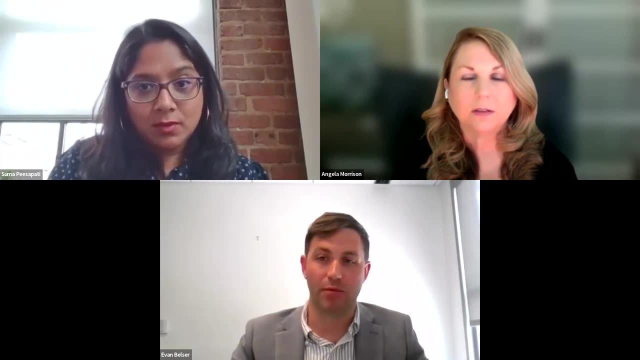 broadly. You know the exact regulated person may not be, you know, known And it's difficult to identify often any one community or person that's specifically injured by the alleged conduct. So it's not to say they couldn't do it, I mentioned. 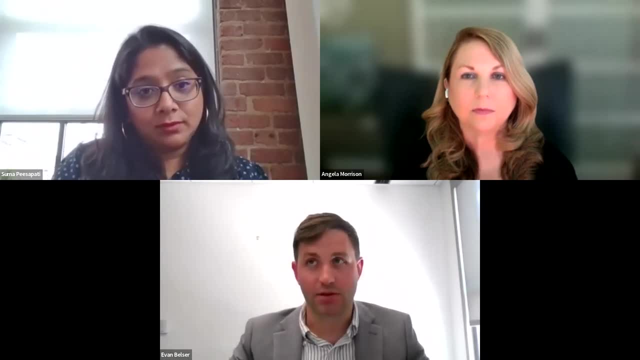 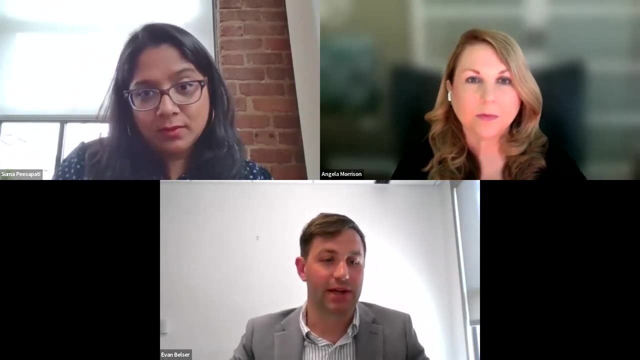 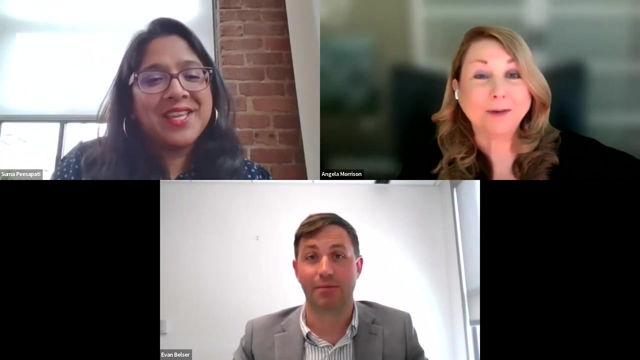 the Utah example, but it's going to be tricky. There's really tricky standing questions. There's tricky jurisdictional interpretation questions of 304F in particular- And, like any other lawsuit, it requires you to have good evidence and good lawyers And money and money. 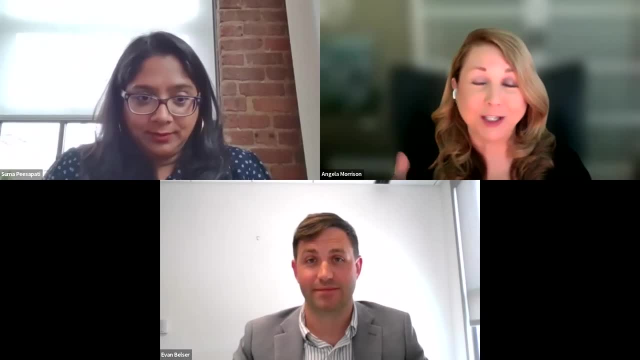 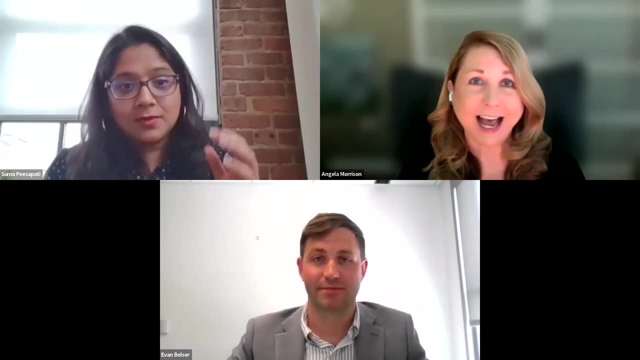 I usually tell people is: you know, if you have a problem, just call the agency, because they are good with enforcement. You know the local programs, the state programs and the EPA. if you can't get your state to act, you know they'll come out and investigate. And there are. 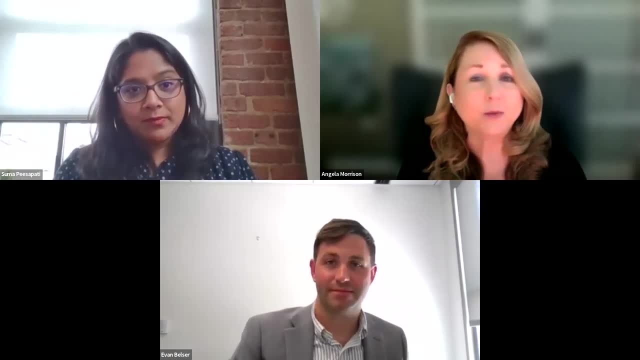 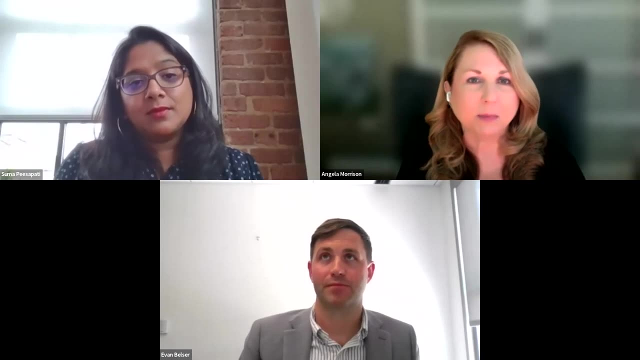 small business assistance programs established to help. you know, small dry cleaners, or you know, little mom and pop operations, comply with the Clean Air Act And you know the focus is always on compliance And you know, I think, that there's just a collaboration of the agencies working with. 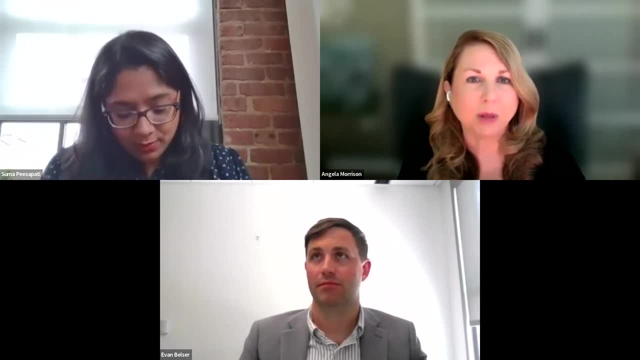 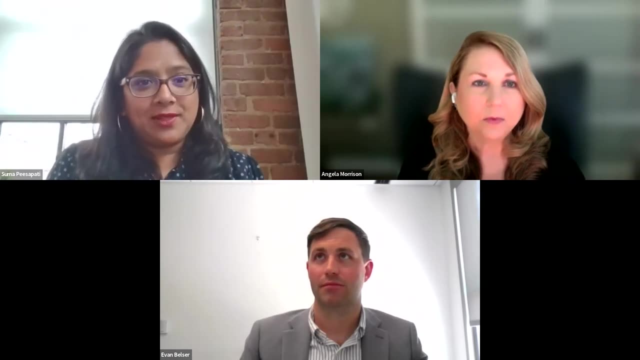 these And you know different industry sectors to make sure they comply, So maybe there's less need for citizen enforcement. Yeah, I mean having brought citizen suits over the in the past, I mean I think case selection is critical. right, You know, can you win? for instance, you know questions like: can you win? 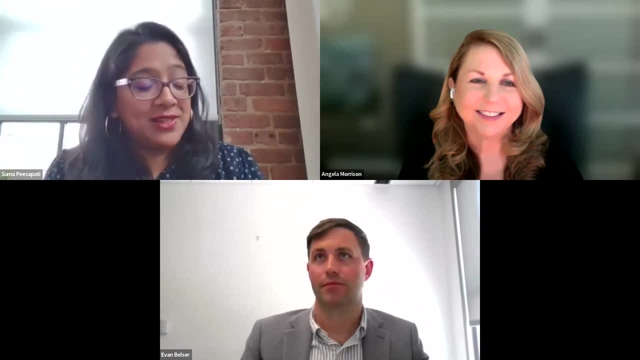 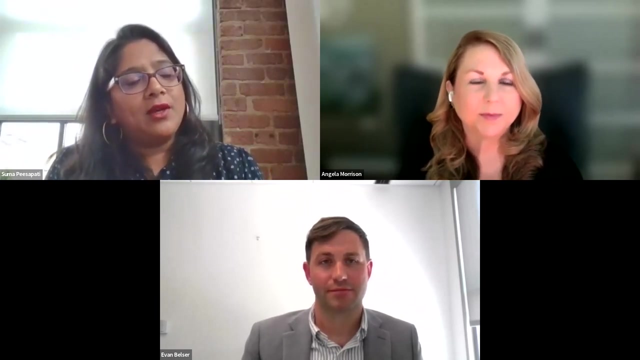 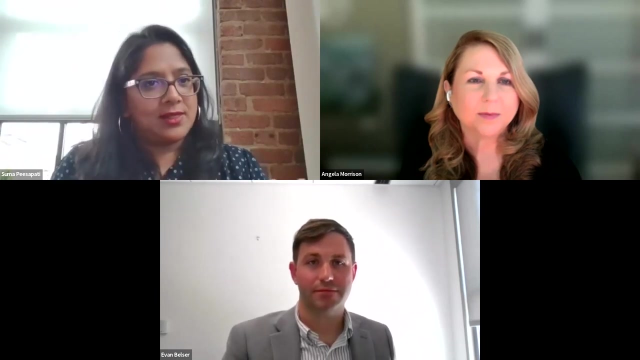 on summary judgment. You know, those are the types of things you think about as a practical matter, especially when there is a vast differential in resources. That being said, there are also. I've also found it particularly rich to like a rich experience to be able to partner with federal prosecutors. So, for instance, 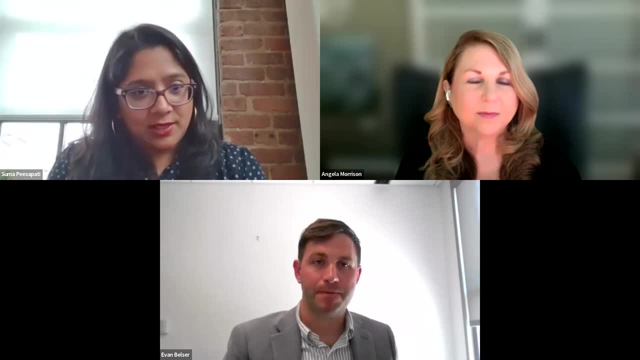 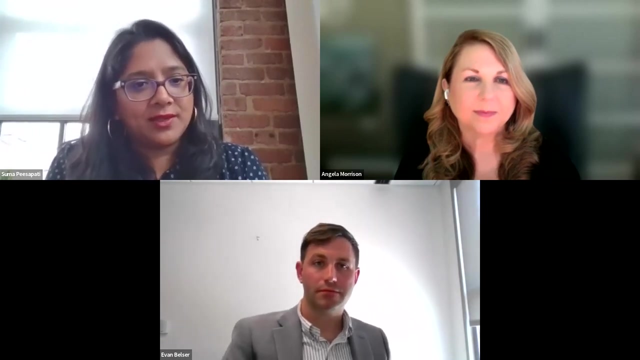 a joint citizen suit and federal action and joint prosecution effort with Region 9 of EPA in reducing pollution from what was then one of the largest coal plants in the country And I found that collaboration incredibly productive And so those are also opportunities. you know citizen suits do occur, you know. but 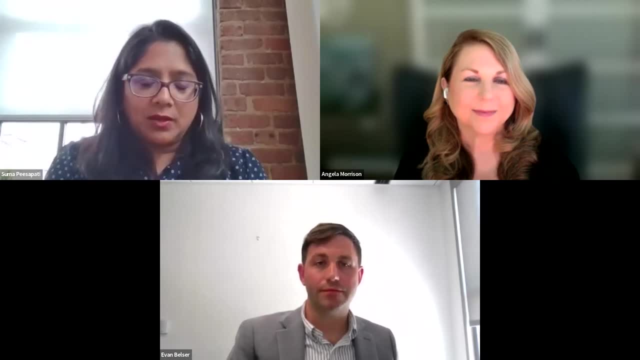 yeah, I think all of the elements you both mentioned are obviously really critical. Somebody- I saw my name bringing EJ to the forefront. Would you mind speaking to the impact of permits in the Gulf South And opportunities there are for communities who aren't located in states with slightly progressive SIPs? 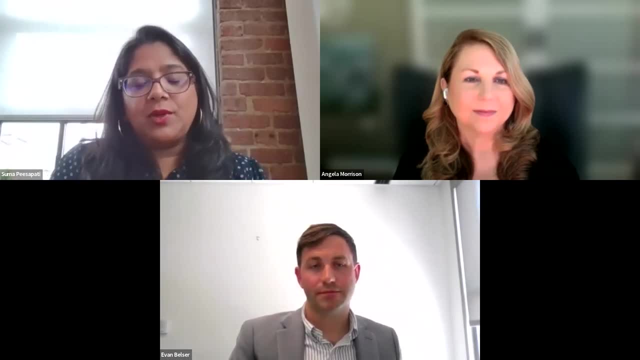 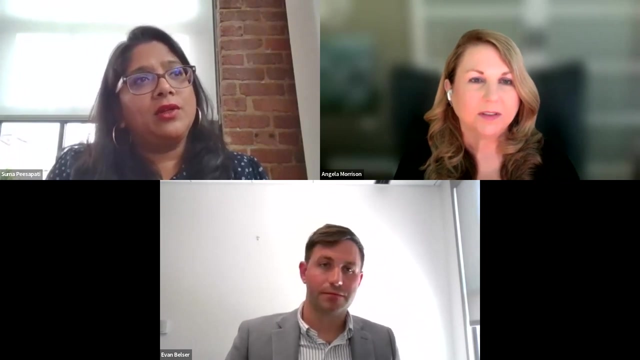 You know that's a bit of a tough one. I don't really know all that much about the regulatory landscape in the Gulf South. I know that there are critical EJ issues there. I will say that in the coal plant context, and as I mentioned earlier, there were opportunities to leverage other aspects. 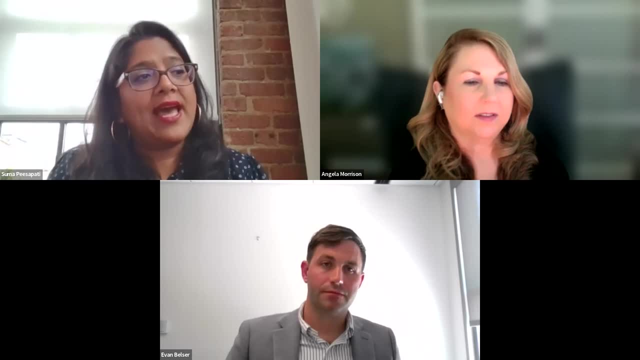 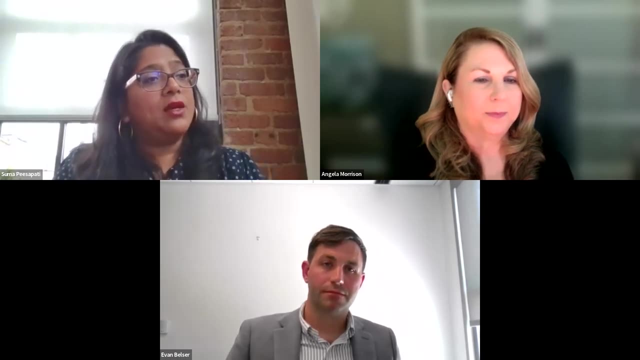 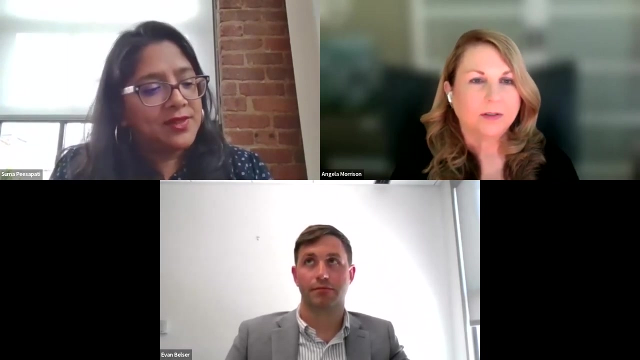 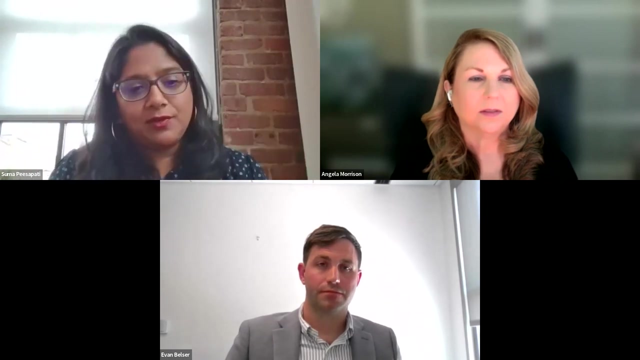 About the Clean Air Act, like the HAPs hazardous air pollution provisions that Angela mentioned in her presentation, the regional haze provisions- I don't know if there are Class I like national parks in the vicinity, but ensuring that there's compliance with other elements of the Act, Just apart from you know the specific sector based requirements that might be relevant to the plan and I can't say that this is a long process. So thank you. 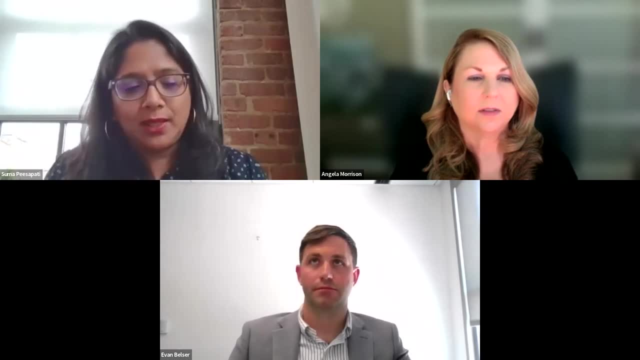 Okay, Alright, Thank you, Thank you. Okay, thank you so much. Thank you so much. might be in a particular SIP, but you know, often a careful look at permit requirements. I mean, you know Title V permit, I mean the air quality permits for stationary sources are rather complex. 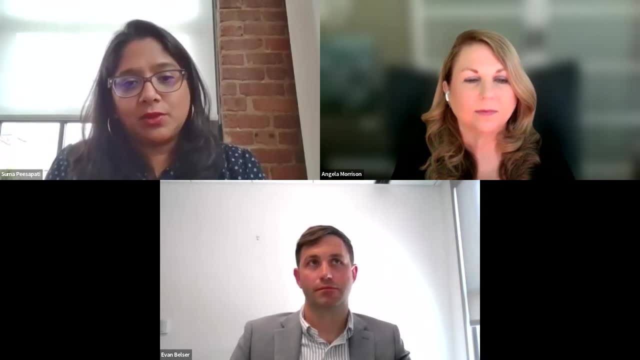 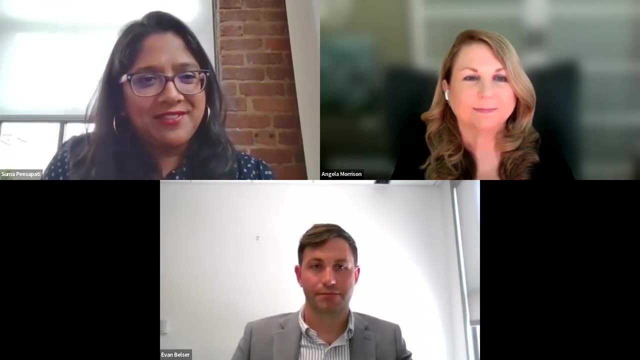 and long. So taking a close look at compliance with those permit requirements is often an important place to start, is what I would say. Anybody else have things to add on that front? Like you said, I think it would be case by case the actual legal hooks, but often citizen. 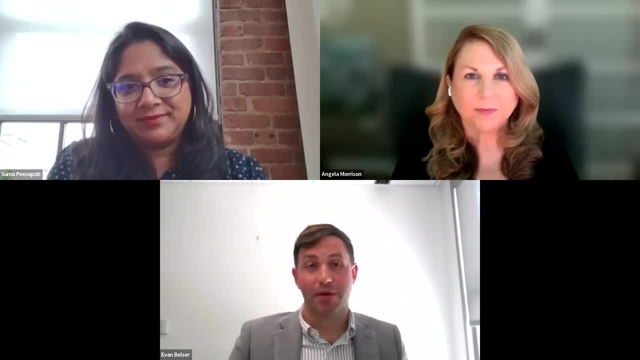 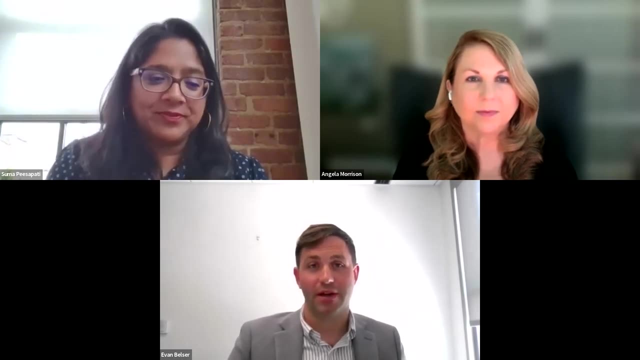 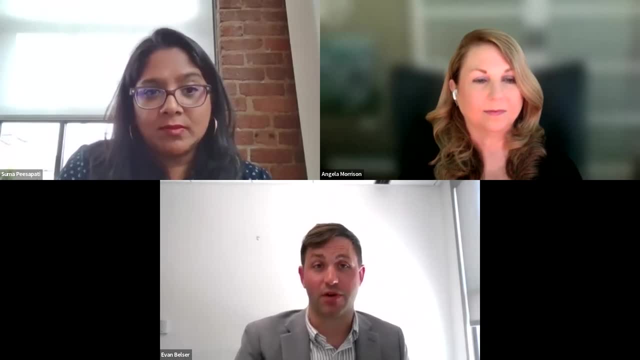 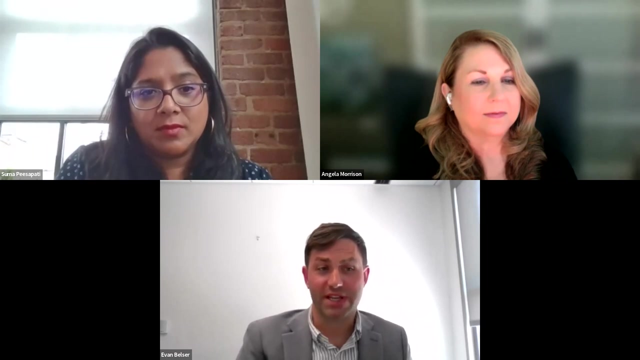 cover only those vehicles that conform in all material respects to what you certified. they mean make it that way, and so you know vehicle manufacturers around the world are watching that very carefully, and it is of particular consequence with diesels. it's more, it's been found to be. 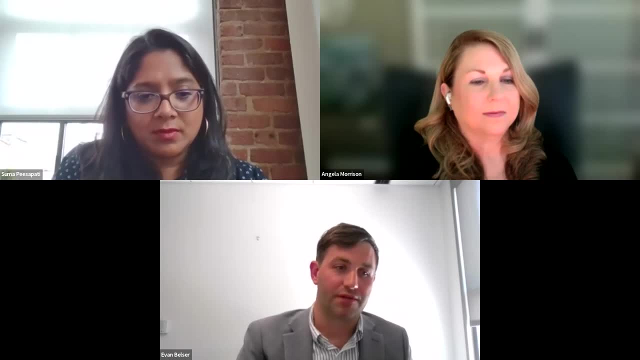 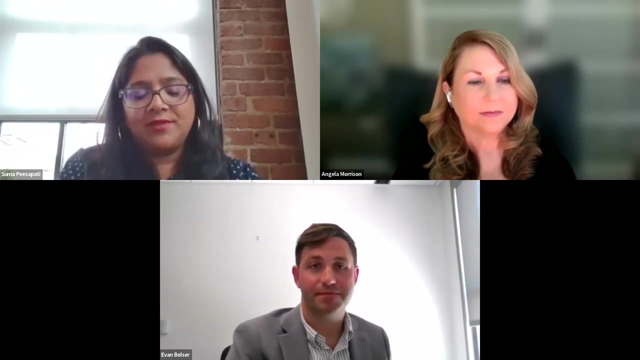 primarily with diesel vehicles, and the proportion of diesels in Europe is much, much higher than in the US, and so that's just additional context for this week's news, but I don't know anything about the merits of the investigation that the German authorities are running. that's helpful. thank you, um. do either of you have views? 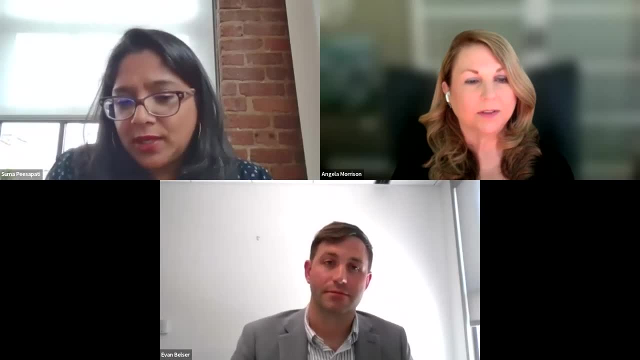 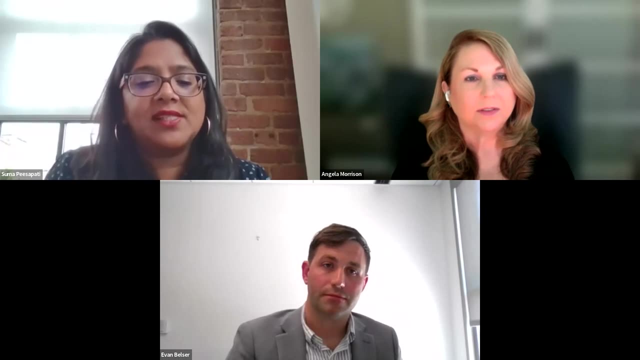 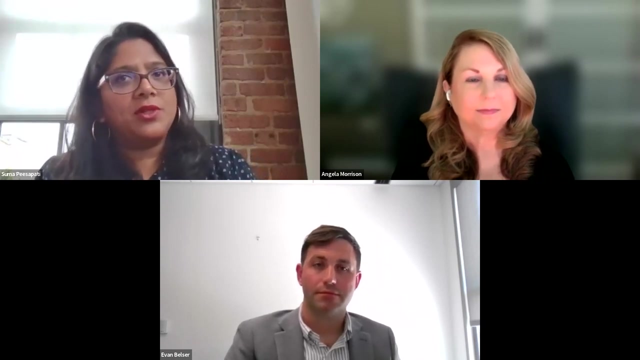 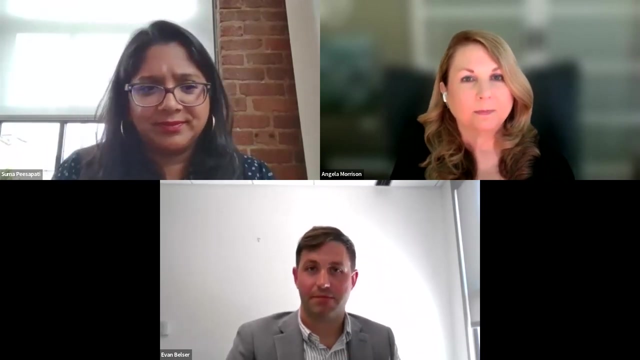 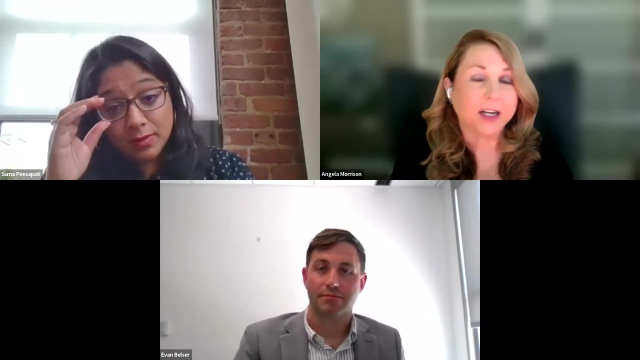 on whether the Clean Air Act and subs, um and what, and surrounding case law have implications for facilitating carbon sequestering programs going forward. that's an interesting question: the connection between carbon sequestration and the body of law surrounding the Clean Air Act. I think that would come under best available control technology or really the technology forcing. 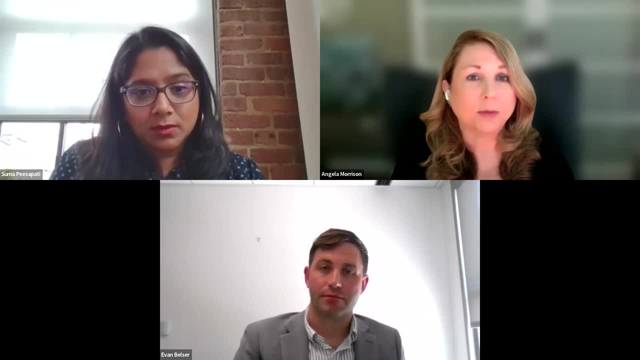 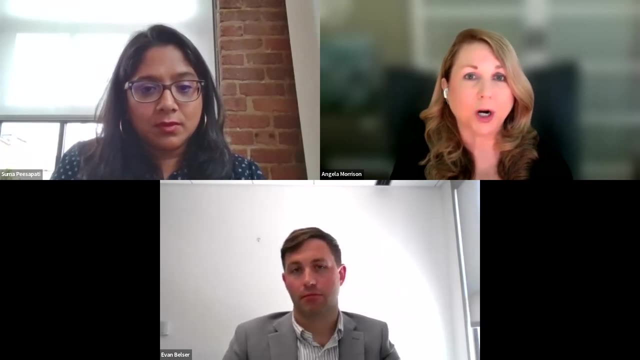 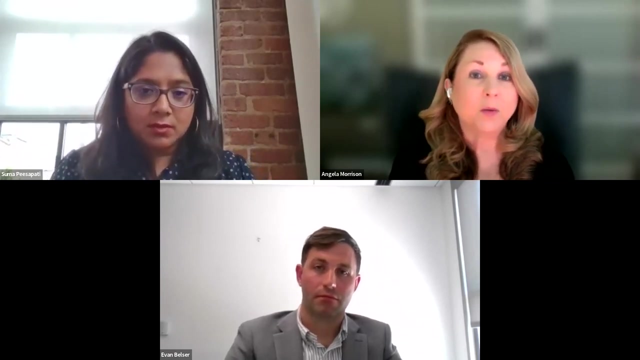 NSPS standard that exists for new coal-fired plants. there's no way a coal plant could meet the NSPS standard without carbon capture and sequestration, or CCS for short. the natural gas plants can currently meet it without CCS. but if, if we did want to turn, to new coal, it would definitely need CCS and going forward once that technology becomes proven- and we're still on a fairly small scale, so it's not necessarily proven technology- that would constitute BACT. once the technology gets there, it could be required even for natural gas plants. my understanding is it doubles the cost of a natural gas plant. so I think extreme improvements would be needed, you know, for the scale of that technology and the cost of it to become reasonable. but I think BACT is probably the the place it would most likely be imposed. 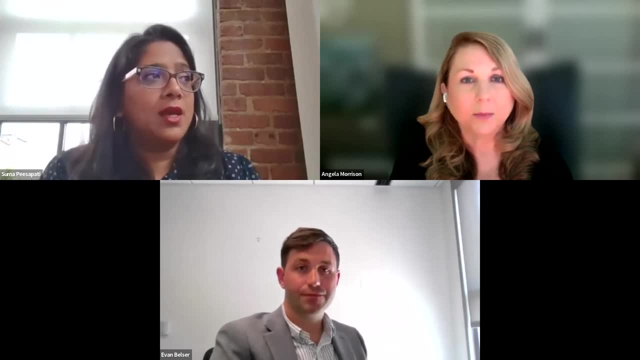 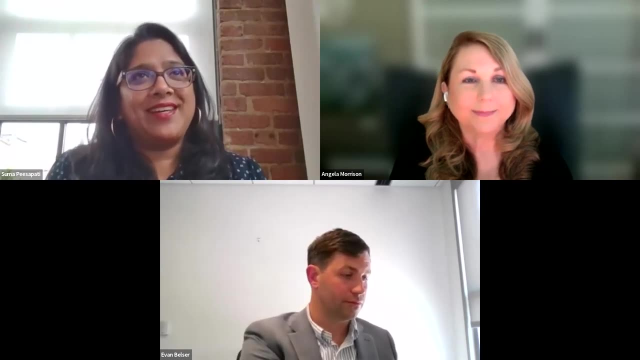 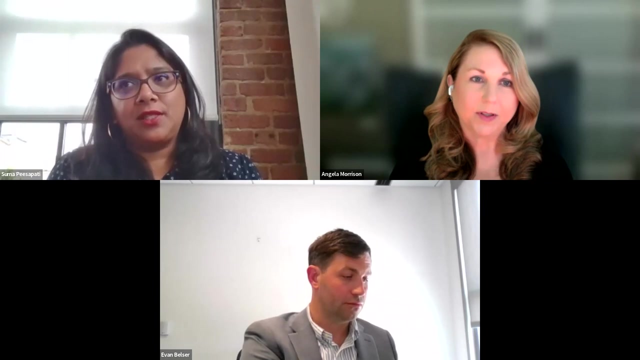 yeah, I mean yeah, that is um. and to your point, Angela, I think there's um. there are some questions still about um, the effectiveness of that technology, um and um and also um some controversy as to how it's used. um, you know, I've seen some coal. 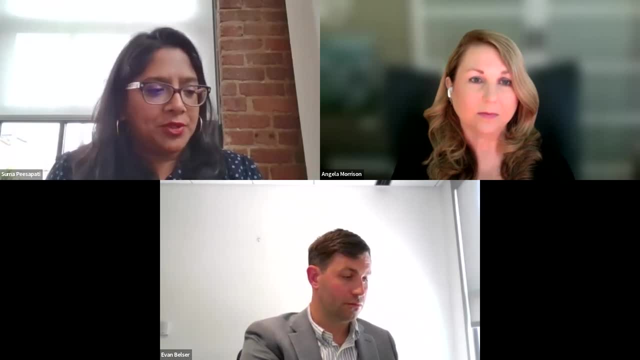 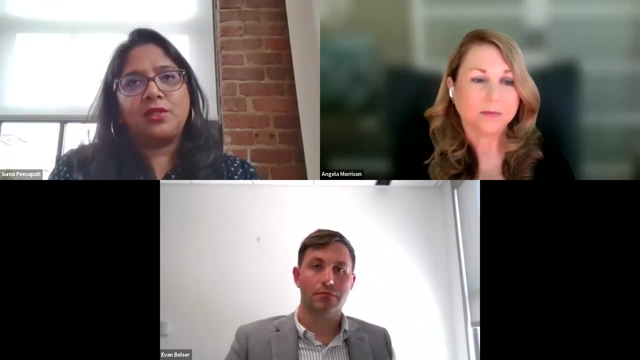 projects where um carbon capture and sequestration is paired with enhanced oil recovery, which can be cause some controversy, um with respect to those projects, and so it's a it's a big topic and a complicated one and um. thank you for your wonderful insights on that um and I might 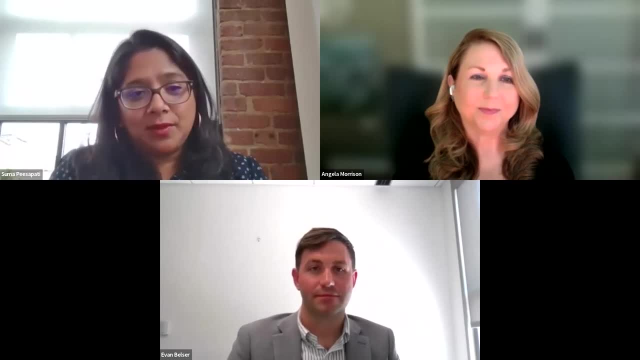 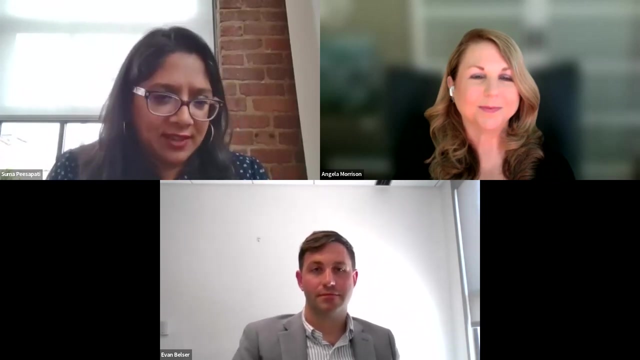 tap you to provide a little bit more um information, Angela, on the connection to the quote-unquote new science, but actually just quickly one of the issues. for sure you know that it's about climate change and climate change and all that, but, but the question between, or the differences rather between, NEPA and Clean Air Act, and so somebody has asked: does NEPA address? 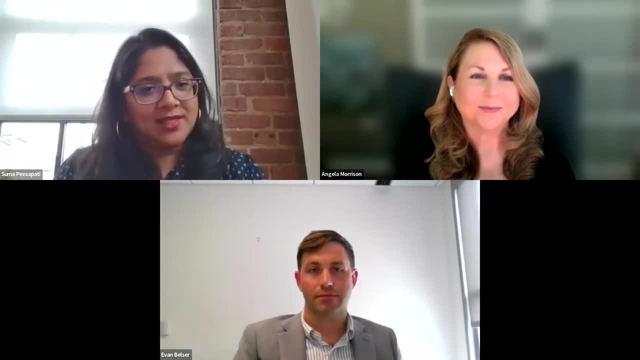 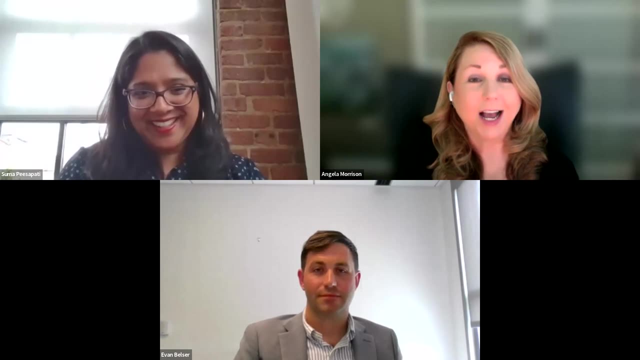 the environmental consequences of an activity, and the Clean Air Act deal with regulating sources. I think they're trying to understand the difference between the two statutes. if you wouldn't mind, well, since I spent most of my career dealing with the Clean Air Act, I have dealt a lot less with NEPA. 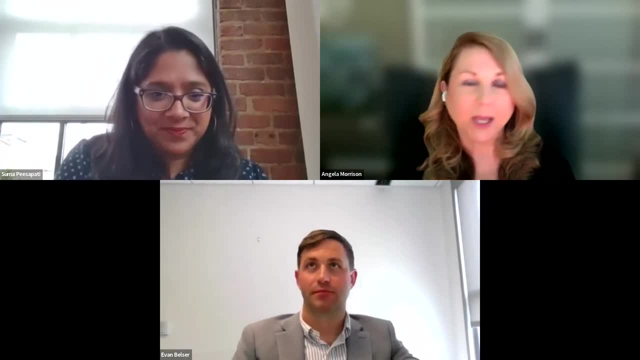 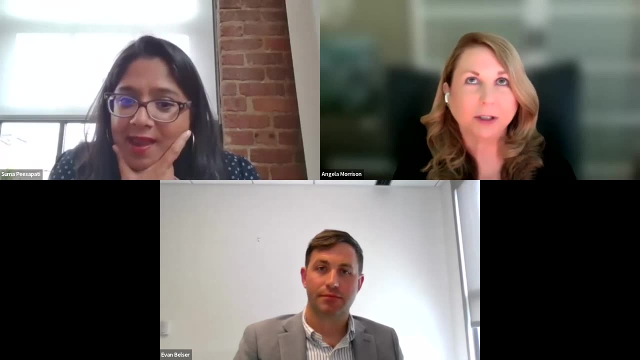 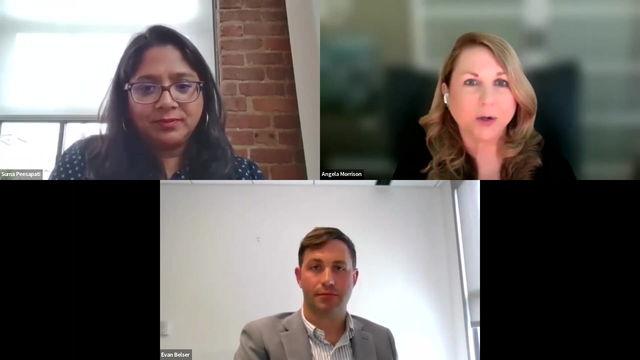 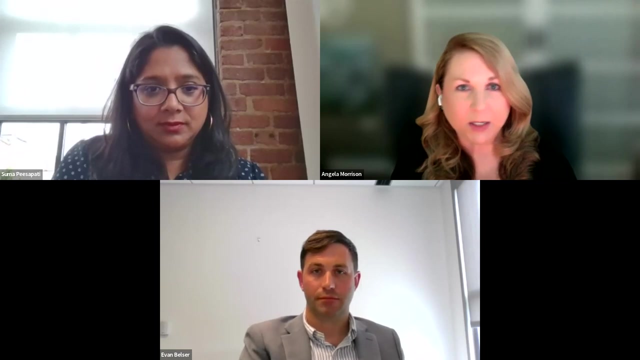 but in NEPA you're generally looking at all kinds of environmental impacts and if there's federal And if there's federal money involved and an air permit, you know you can get into NEPA and an air permit in the same context. But NEPA is generally looking at all the different environmental impacts, whereas the Clean Air Act you're really looking at compliance with the ambient standards and PSD increments and just compliance with all the standards, not, you know, impacts on endangered species or you know something like that, unless they're endangered at a class one area. 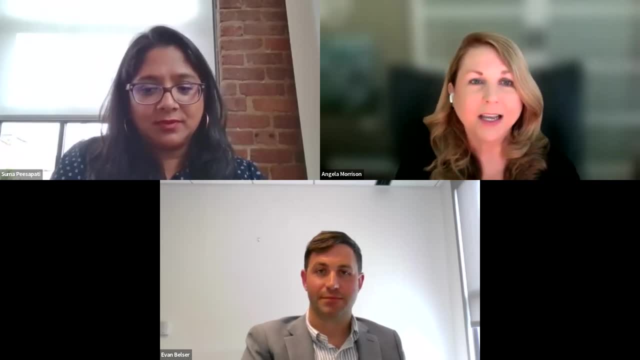 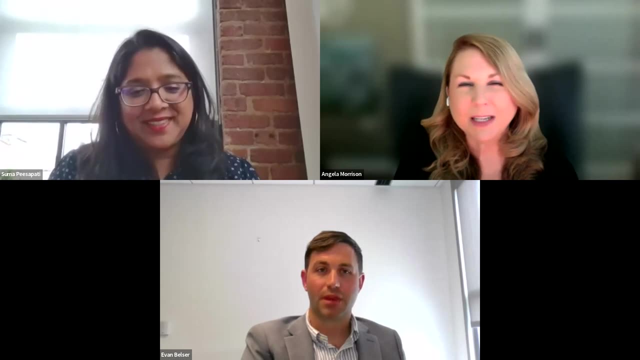 And we do get into additional impacts analysis there in a class one area. but you know, maybe not you know- endangered species just next door. Does that make sense? I think so, And I'll just add that the nature of the statutes are different. 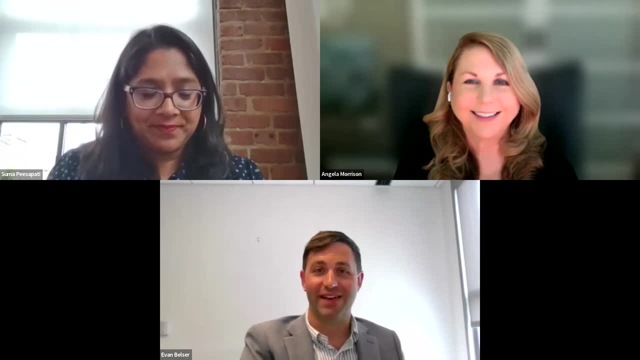 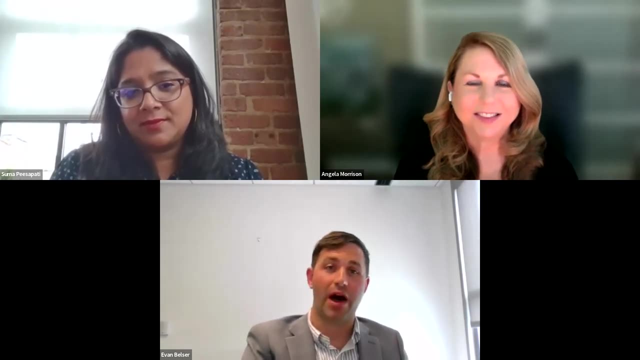 They're both big statutes so this is risky to try to compare them at all, but NEPA requires that certain federal actions undergo a process to evaluate a wide- like you said, Angela, a wide- range of potential environmental impacts, But doesn't set standards, requires that there be consideration of alternatives that are less impactful, and Clean Air Act is more about setting a standard for performance or or or operation of a source. that's often boiled down to numeric standards. 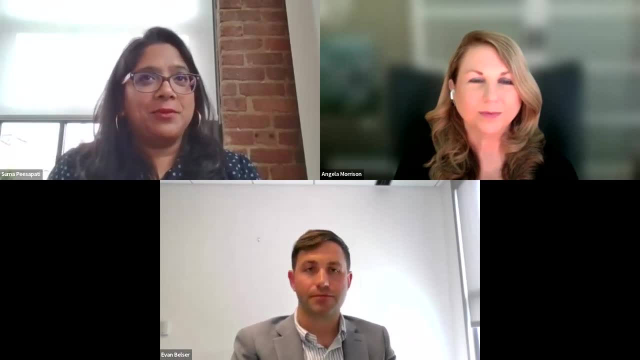 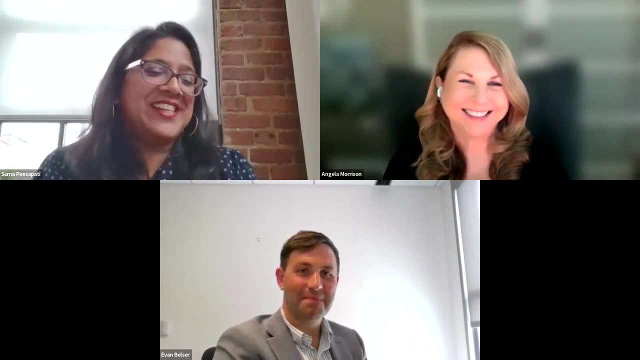 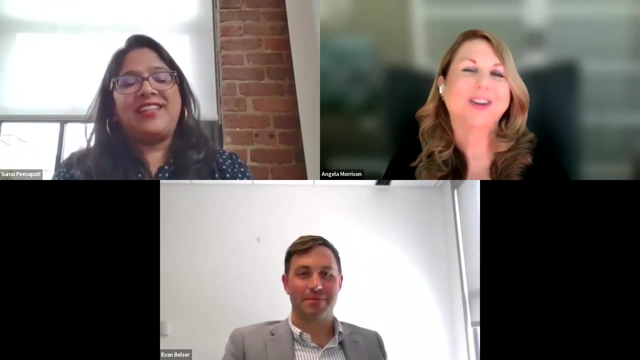 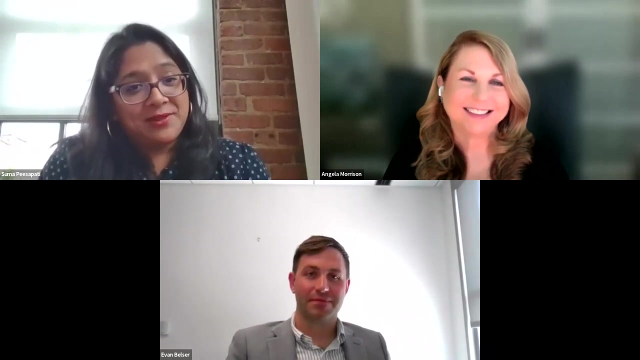 Yeah, I mean, I hate to muddy the waters here, but here in California we have- I don't know why it's little- NEPA- Yeah, they call it baby NEPA, but it's our CEQA statute and I'm like that's NEPA on steroids because it actually requires mitigation and you know, and quality permits are subject to CEQA and you know NEPA, which is really a disclosure statute, information disclosure statute, you know, is there's a distinction because, yeah, like I said, on top of whatever permit conditions may be included, there's also this requirement of mitigation. 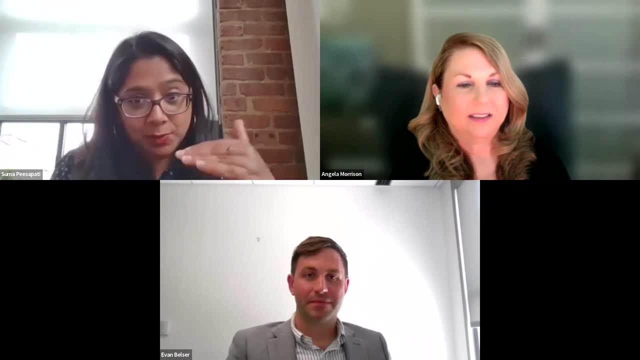 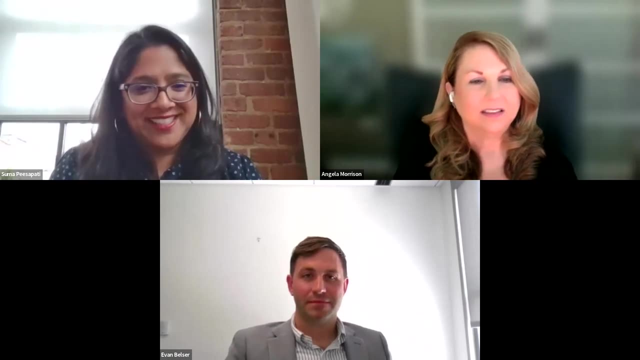 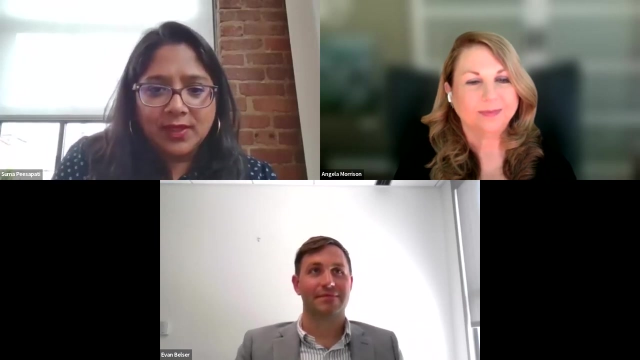 I mean, if you're just applying a sort of a positive, you need to have some kind of an appropriate recommendation to you know, make your decision made And- and I think it's also part of the Department's work- to reduce impacts below CEQA's thresholds. And so, yeah, kind of an added layer of complication here in here in in in California. Let's see, I think you already answered this question, Evan, about the decision handed down by the court today in Chevron. deference For whether it might be intended or not, it's something we're here to answer and make sure. yeah, I won't go over that anymore, And if it's not a decision, it's okay, All right. 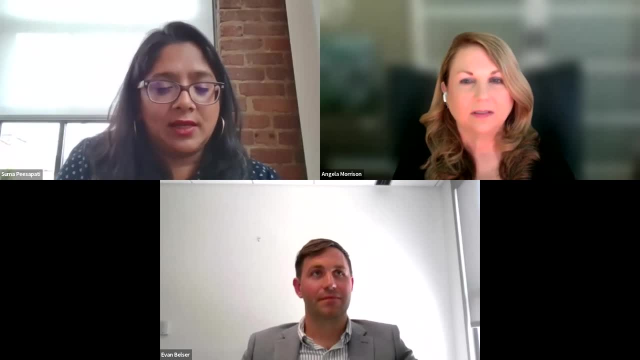 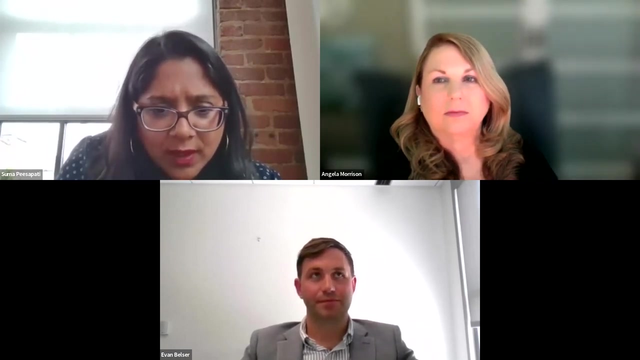 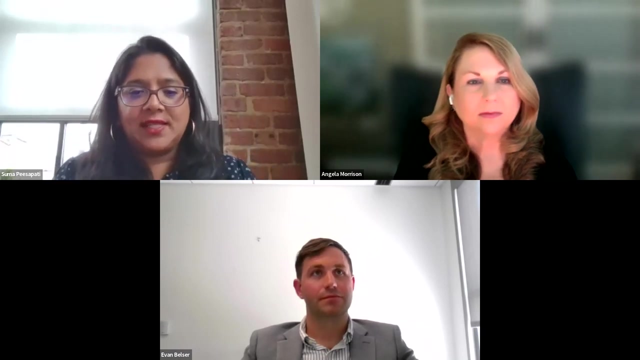 further eroded. um, i think you mentioned you didn't see a reference to chevron deference. it was unclear that, um, that you know that particular uh doctrine would be impacted, right, yeah, um, let's see there's one. how how would a permit process for a facility that is currently in compliance? 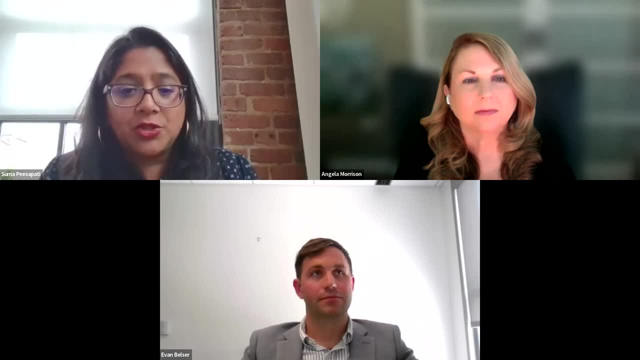 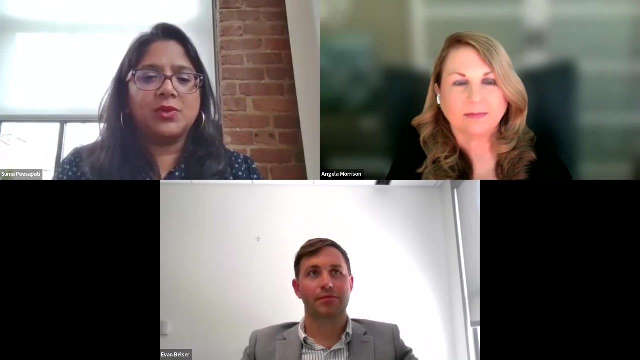 with local standards. uh address health impacts present based on past actions when a facility was not in compliance. permit process for citizens currently in compliance will address health based on past actually was not in compliance. well, to me i feel like that's more of an enforcement issue um so long as, then, past non-compliance um i don't, i mean, i think um. 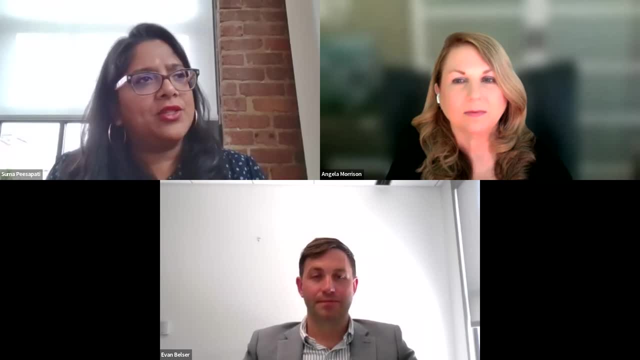 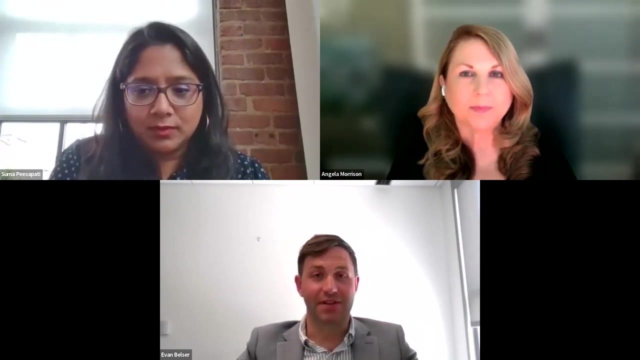 yeah, i mean, you know, if you're within the statute of limitations of the previous non-compliance. yeah, i would see that not as a permitting issue but an enforcement issue. what do you both think? yeah, i think that's right, permitting it's. you know, obviously past data is is relevant to setting. 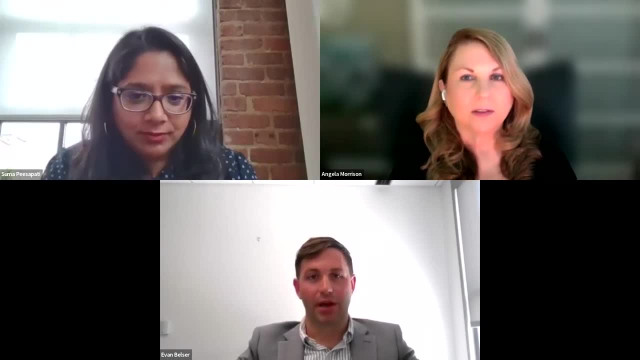 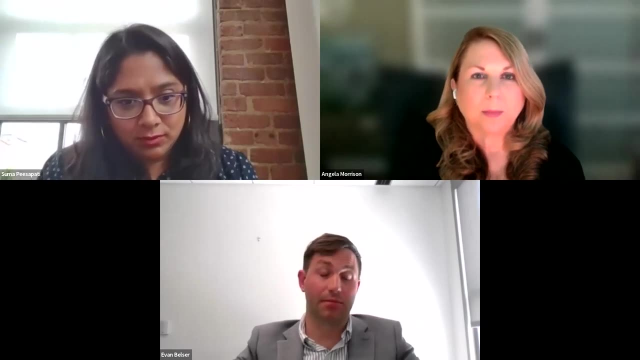 standards or whatever going forward, but i i'm not aware that the permitting that requires lower than otherwise required to account for past emissions. that would be a remedy in an enforcement case in most cases. yeah, one thing to keep in mind- and this is what you need to take away from this- is: 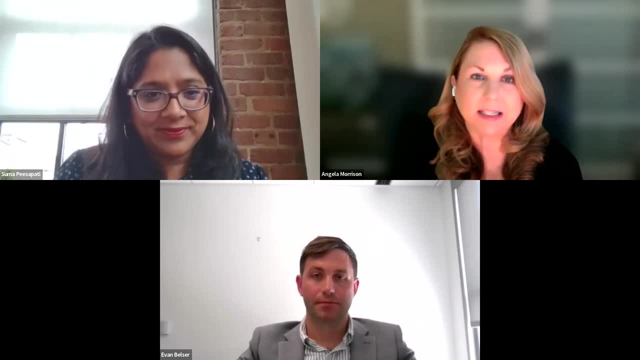 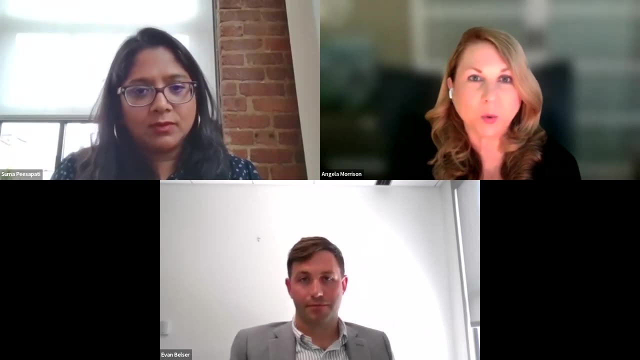 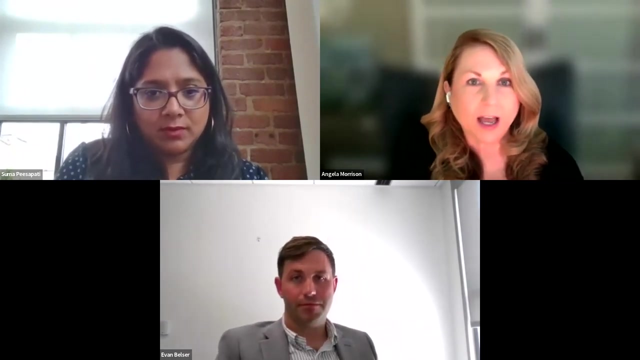 ambient standards don't apply to the sources, they apply to states, and so if your facility is causing a violation of an ambient standard, there's no enforcement action against that source. the state needs to revise its sip and establish, maybe stack, specific standards for that implicated source, but you wouldn't violate it and there aren't even ambient standards for the hazardous. 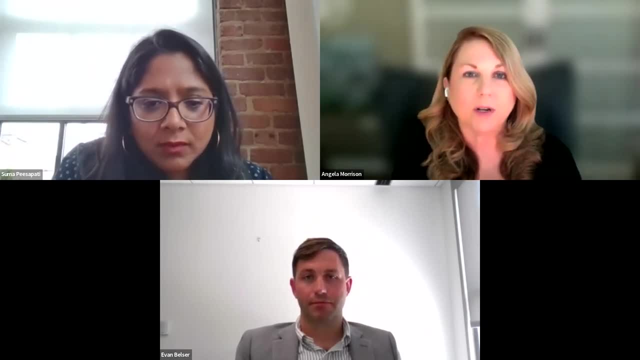 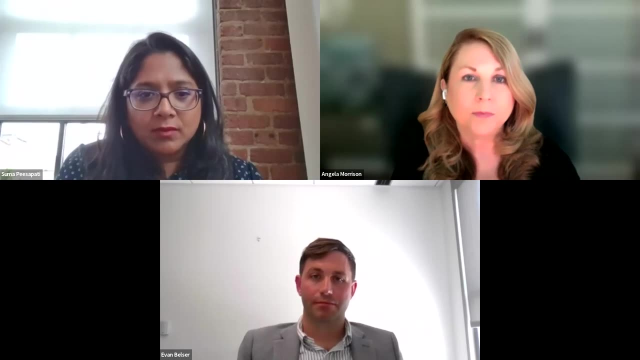 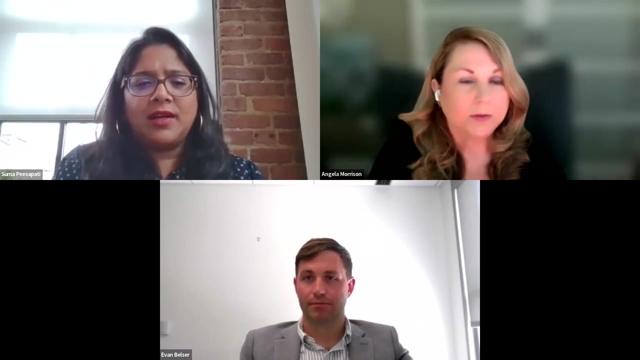 air pollution. there are only screening thresholds that epa looks at when it's reconsidering its max standard. so for the most part, stacks are regulated at the stack, not at the fence line. oh, this is an interesting question. are aerodynamics regulated under the clean air act?